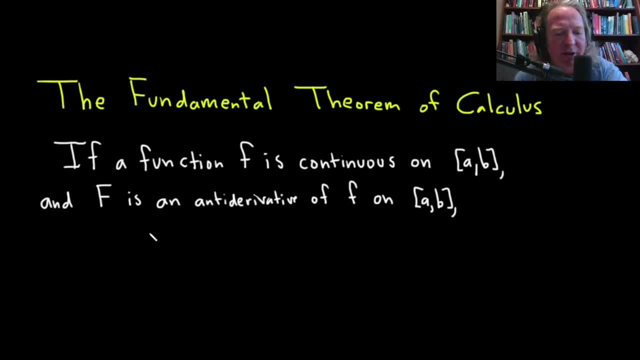 of calculus says that if you have the definite integral from a to b, of little f with respect to x. So normally we had to use, you know, limits and stuff. We had to take the limit of a sum and the process was very, very difficult. This gives us a. 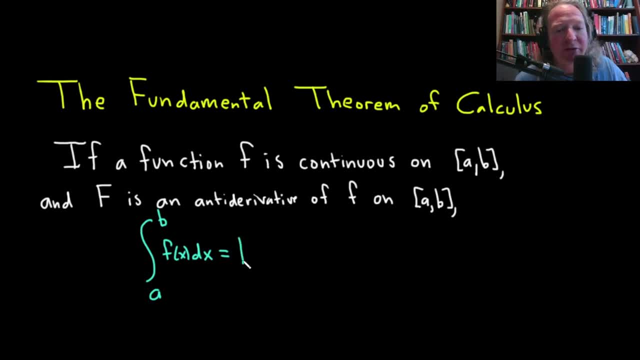 formula: This is equal to the antiderivative of little f, so big F evaluated at the uppermost limit of integration, minus the antiderivative of little f, which is equal to the antiderivative of little f, so big F, evaluated at the lower limit of integration. So it's a really cool equation. 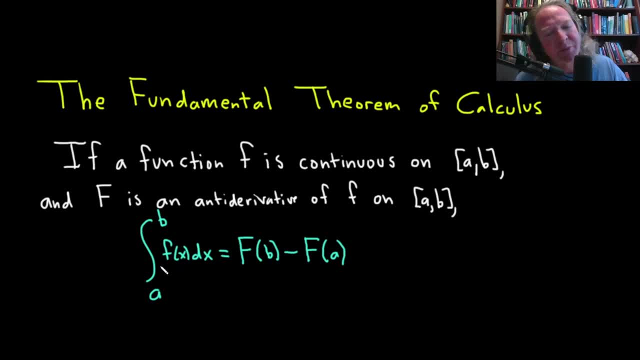 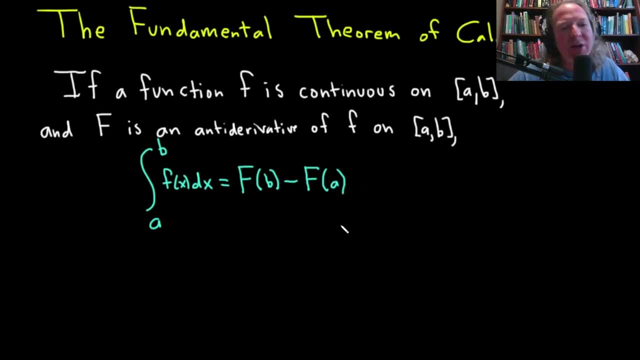 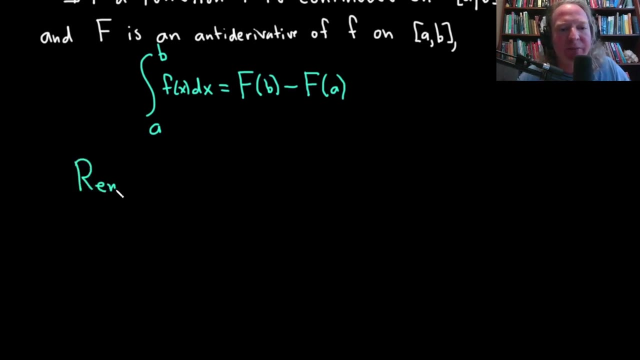 because it relates everything we were doing with definite integrals back to antiderivatives, right? So it's big, big step and it makes the computations so much easier, right? So much easier. A couple remarks that need to be mentioned here, So perhaps 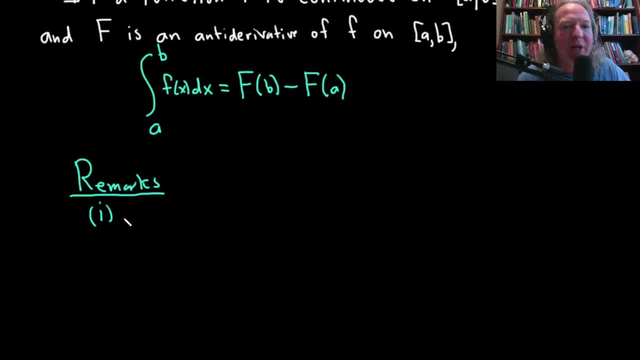 the most important remark, or an important remark, is that you don't need to write the constant of integration anymore. So whenever you're doing definite integrals, you don't need the constant of integration. So don't need, don't need to add c And two. second remark: 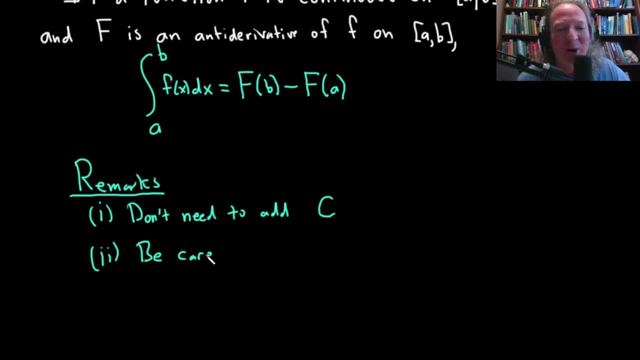 is to be careful. So we're working. we're going to be working with numbers now We'll have a lot of fractions, So you want to just take your time and, you know, go through things slowly. Let's start with a simple. 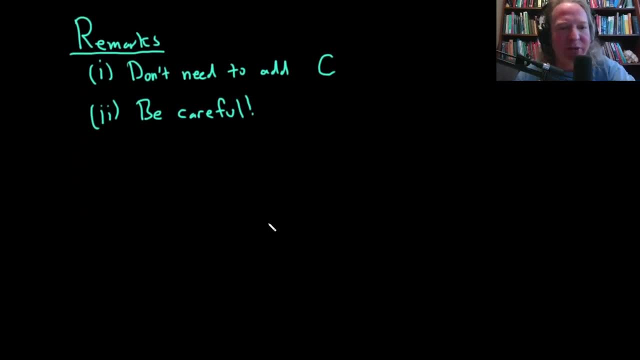 example that we can work out. So you see how to use the fundamental theorem of calculus. So let's start off simple. Let's say we're integrating from 1 to 2, and we just have x with respect to x, So x, dx. 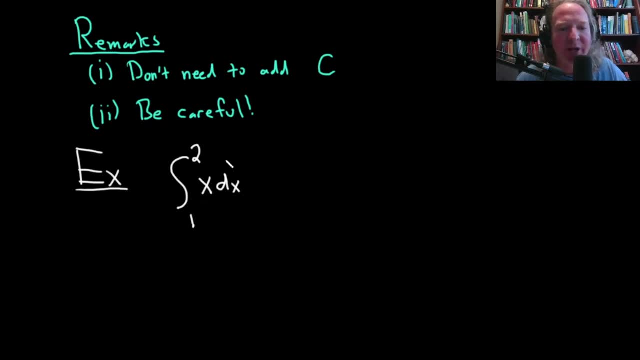 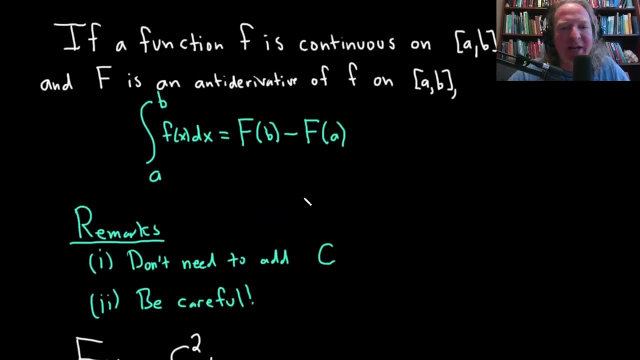 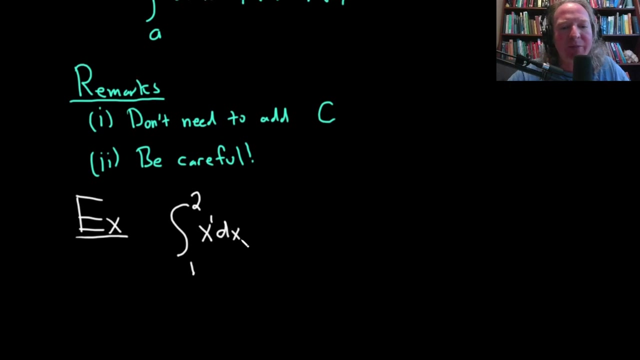 We're integrating x with respect to x. So basically, according to the formula, it's going to be big F of b minus big F of a. So typically what you do is you just integrate it and then you don't write the c. So here we'll use the power rule. So you add 1 to the exponent. 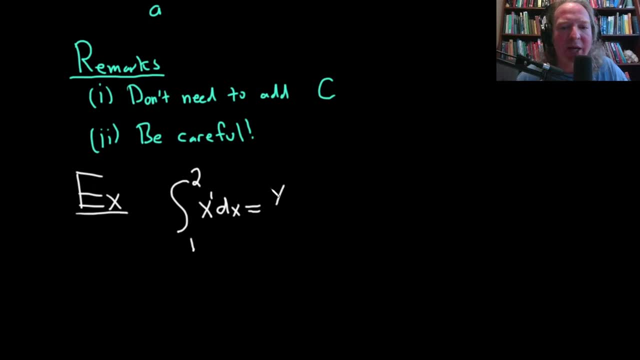 so it's x squared, and then you divide by 2.. So it'll be x squared over 2. And then normally you'd put a plus c. but you don't have to put a plus c, Just to indicate that you don't have to. 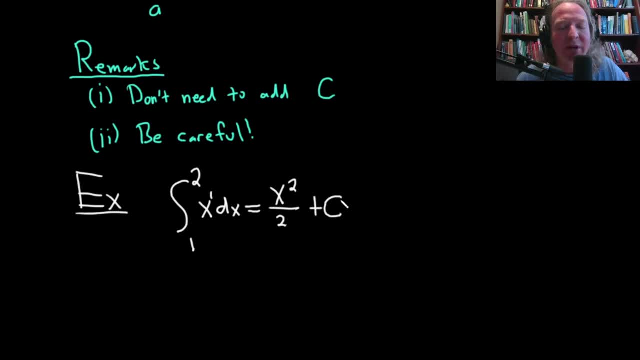 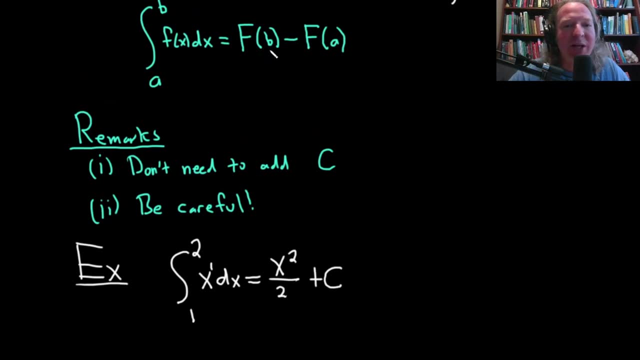 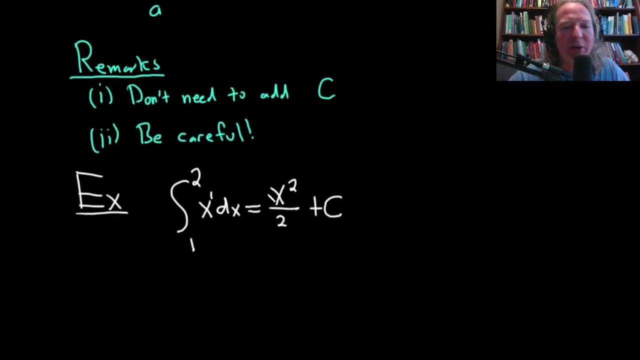 I'm going to put it this time, just so you see what happens. So this is just the antiderivative right. This is wrong. We have to have the antiderivative evaluated at the top limit of integration, the upper limit, and then subtract it from the antiderivative evaluated at the lower. 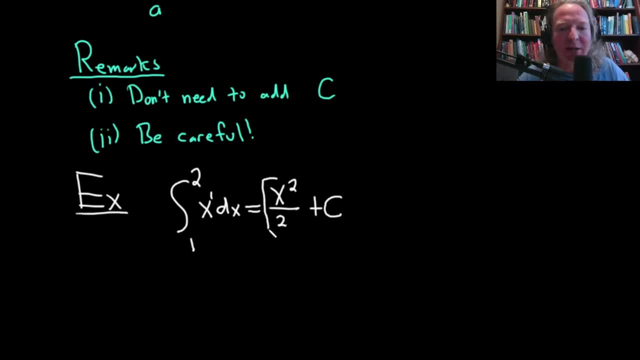 limit. So what I'm going to do is I'm going to use a double bracket like this and I'm going to put a 2 here, And what this notation tells you is that you first plug in the 2, right, Because this is. 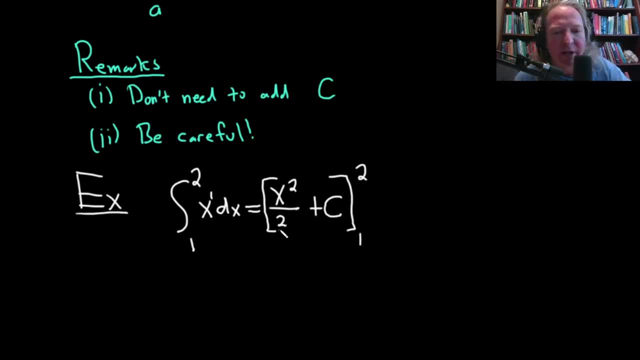 your big F of x right here. Let me just circle it. This is big F of x. So if you plug in a 2, you get 2 squared over 2 plus c. right, That's big F of 2, right, Because you plugged in 2 into. 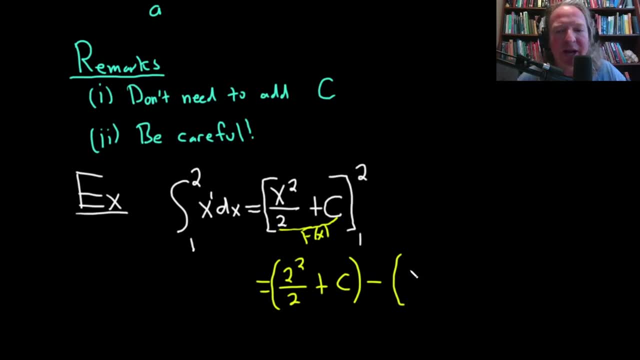 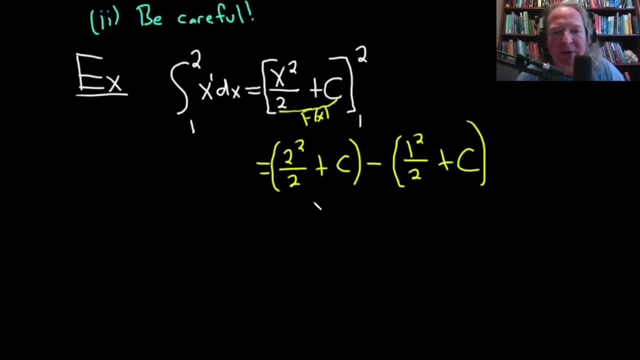 big F Minus and then plugging in 1 to big F, it's big F of 1.. Let me see that. So let me just scroll down here and write it for you. So this is big F of 2,. 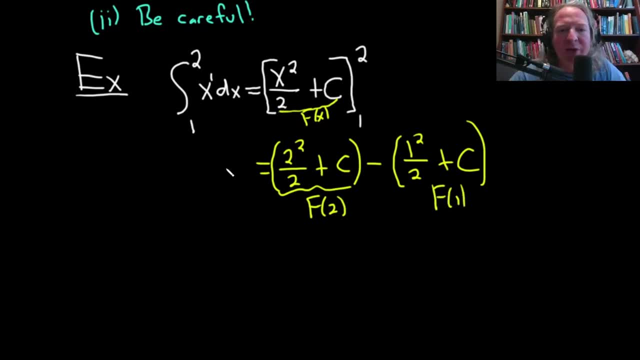 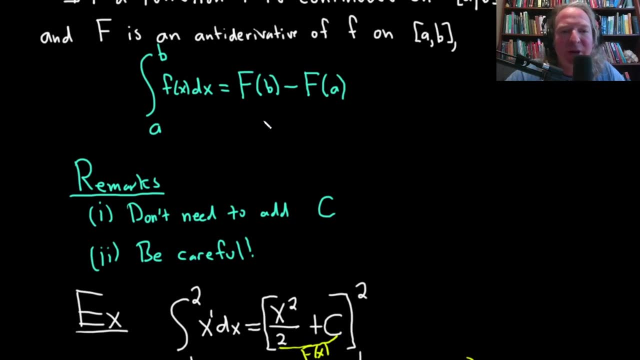 and this is big F of 1, right, Just using the formula, which again is F of b minus F of a. I think a lot of people don't actually think about the formula, which is fine, You don't really have to, but I just want to show you that we are actually using it. right, We're actually using it. 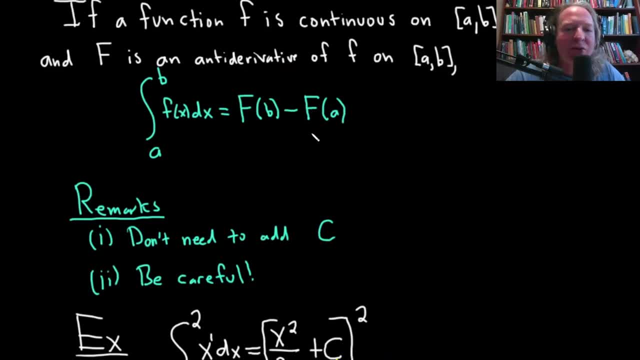 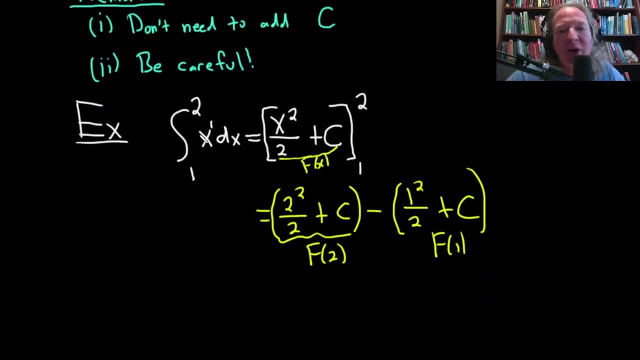 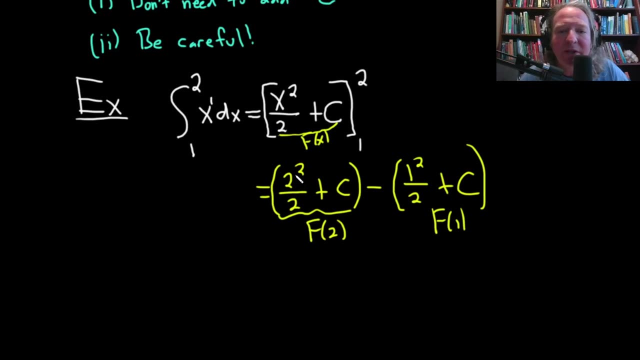 And I think that's lost in calculus, because you take a calculus course and then you learn how to do this and you just keep doing it, thinking about what's happening. So every time you do a definite integral, you're using the fundamental theorem of calculus, which is super key, And so what happens here is you get a 4 over. 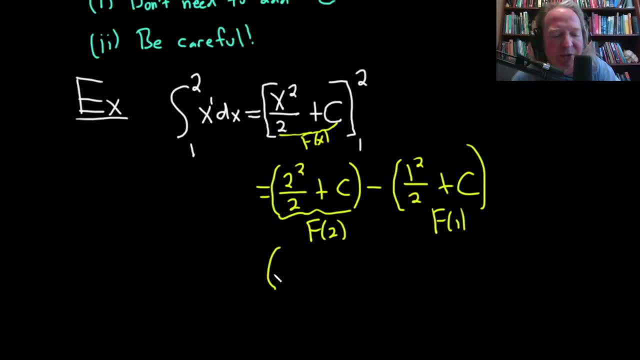 2, which is 2, right, Because this is 2 squared, So it'll be 2 plus c. You can actually drop the parentheses here, So it'll be 2 plus c, right, Because that's 4 over 2.. This is minus 1 half. 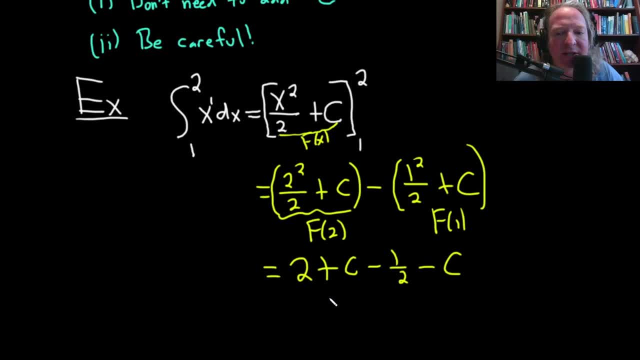 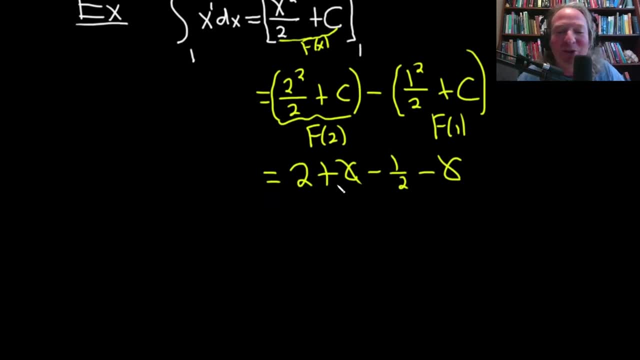 minus c, Minus 1 half. minus c. Oh, this is cool, right? Look the c's cancel. That's why you don't have to write the plus c, right? So 2 is really 4 halves, just thinking of it as a number over 2.. And then minus 1 half, So that's. 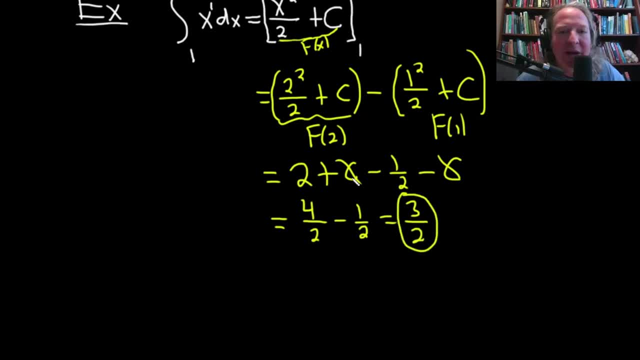 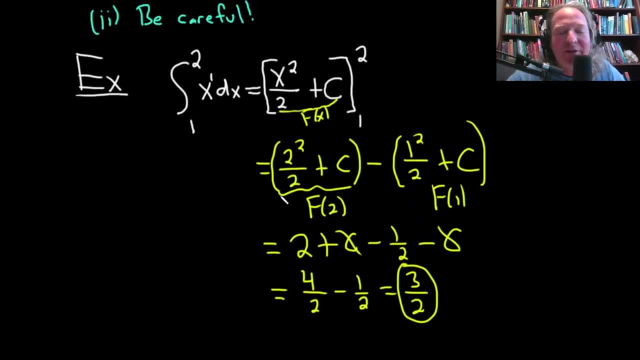 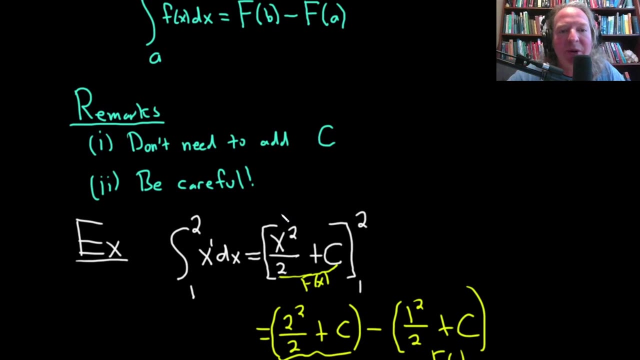 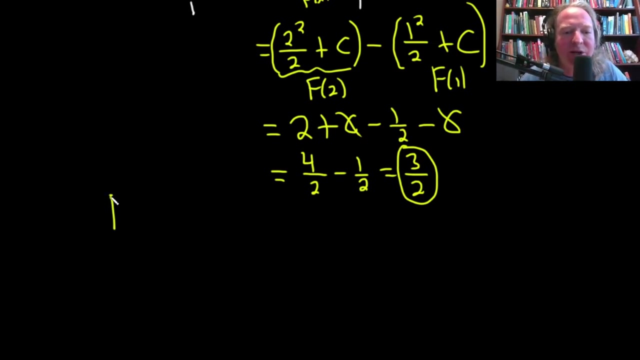 going to be 3 halves. So much quicker than the approach we would take using limits and all of that stuff. So very, very fast way to find definite integrals now thanks to the fundamental theorem of calculus. A comment here on the notation, by the way. So just some comments on notation. 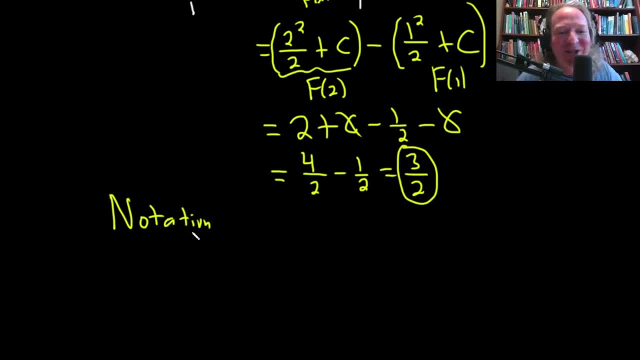 Notation. It's not that hard to spell it: Notation. Okay. so in this example we had, it was a 1 to 2 x dx And I wrote it with a double bracket. right, You could do a single bracket. 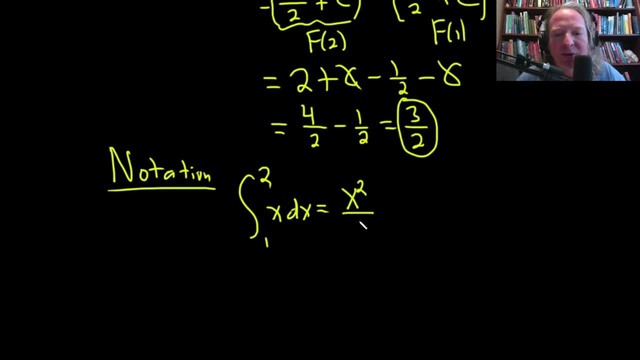 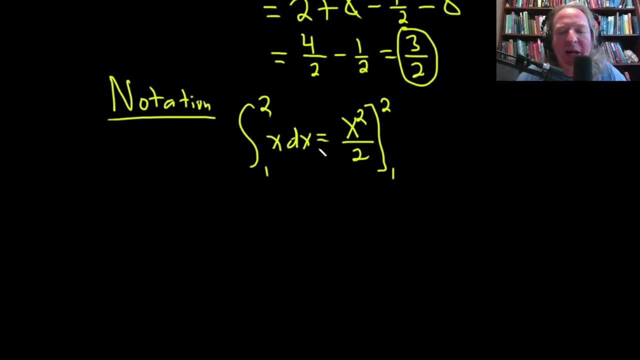 So you could do x squared over 2, and then you could do this, okay. Or, if you prefer, you could simply use a line. So you could do x squared over 2. with a line like this, You can use a double bracket. right, You could do x squared over 2 and a double bracket. So all of these are. 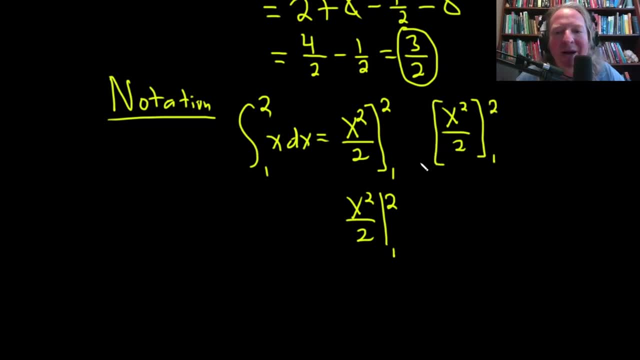 acceptable notations. Just use whatever you feel best fits the situation. I think that's the best way, So I usually do the line or the bracket. I go back and forth between notations. Let's see if I can find another example. 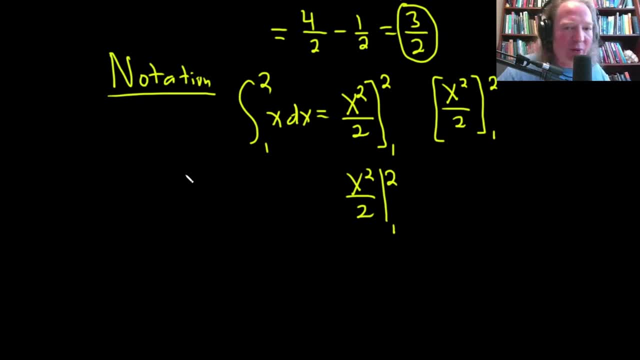 That's a little bit harder. that we can do just for practice. I guess I'll make one up. Here we go, Let's see, Let's try just again. maybe let's put a 0 here and a 3 here, okay, And actually. 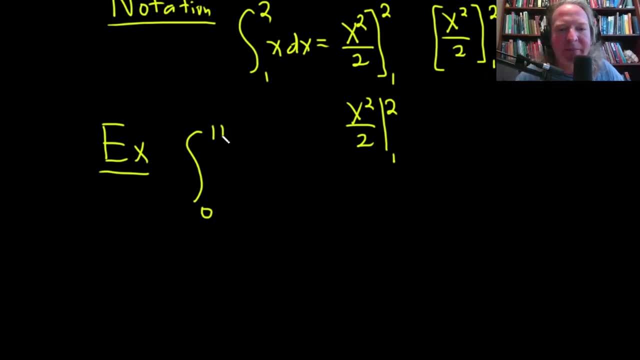 let's make this a pi, Let's do a trig function, Let's integrate cosine x with the x. So if we were doing this using the limit process, it would be much more challenging. So thankfully, we can use all of our integration formulas now to compute definite integrals. 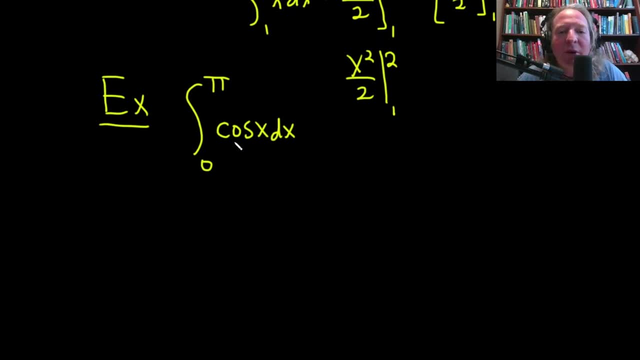 which is huge. So here we're integrating cosine. So we're thinking: what's a function whose derivative is going to give you cosine? Well, the derivative of sine is cosine, So this is equal to sine x. And then I'm just going to use a single bracket here. Then you put: 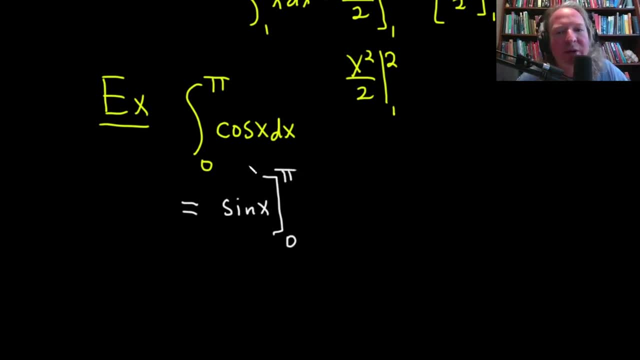 the 0 here and the pi here. Notice I didn't write the plus c right. We know it's not necessary because the plus c's they cancel each other out. And this notation means that you first plug in the pi and then you subtract and you plug in the 0. So you plug in pi, so you get the sine of pi. 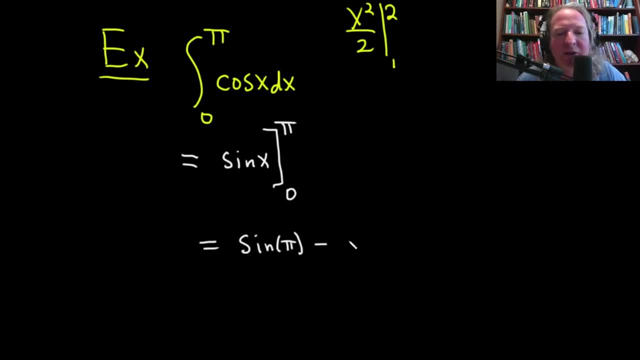 minus, and then here you get the sine of 0.. On the unit circle, sine is the y-coordinate right. So here's the unit circle. This is 0,, this is pi, And you see that sine is the y-coordinate on the unit circle. 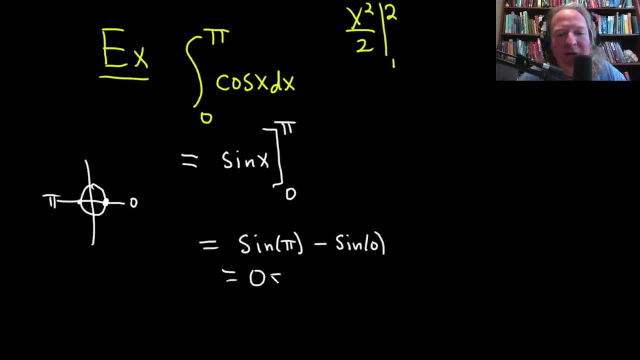 So at 0, it's 0.. At pi, it's 0.. So you get 0 minus 0,, so you get 0.. So that's the answer there, Intuitively, let's think about what this means. We're integrating cosine. 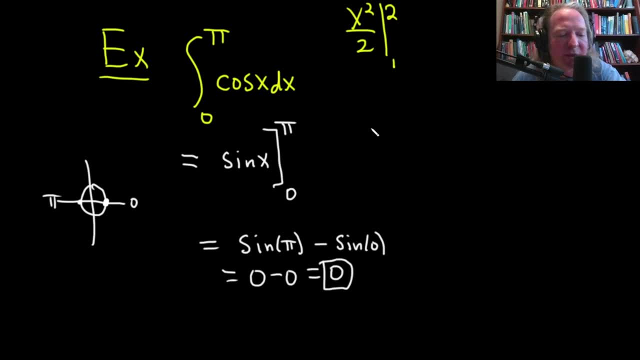 from 0 to pi. So if you think about the graph of cosine, so cosine of 0 is 1, right, And then cosine of pi over 2 is 0. And then cosine of pi is negative 1.. So this is pi here. 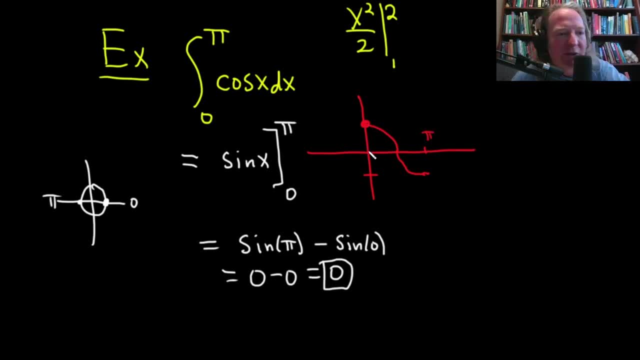 And this is pi, And so we're basically integrating. We use a different color. This is kind of an interesting example. I just picked one, and all examples can be interesting, If you well. most examples So integrating. here we got the area under the curve. 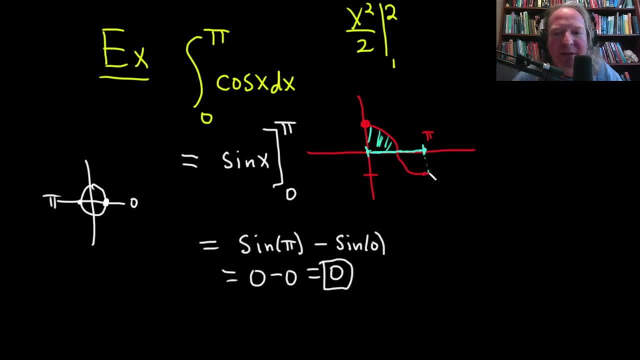 right from 0 to pi over 2.. But then over here it's like we got the opposite of the area under the curve. So if you add these up, you're going to get 0. So if you add this p. 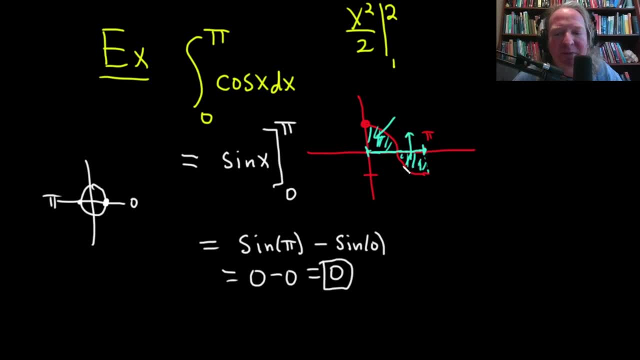 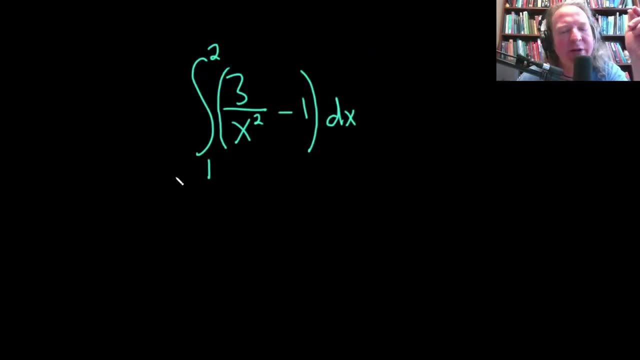 here to this piece here. this piece here is the opposite of this piece, right? So you end up getting 0, which is what we got in our definite integral. In this example, we're going to find the definite integral of 3 over x, squared minus 1 from 1 to 2.. So the first thing we have to do, 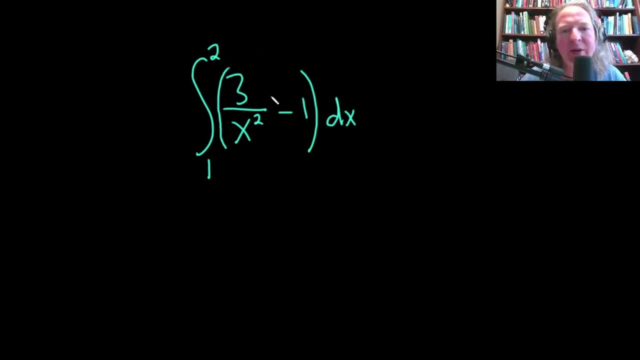 is write this in a way that allows us to integrate it. So we'll start by taking this x squared and bringing it upstairs. This becomes the definite integral from 1 to 2.. Of parentheses: 3x to the negative, 2 minus 1, and then dx. And the reason we did that is so now we 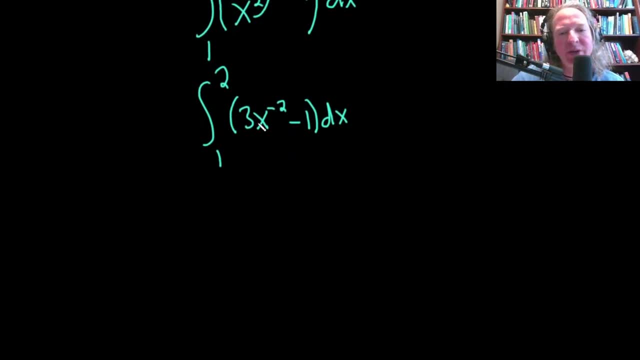 can apply the power rule for integration to integrate this. So when we apply the power rule, basically we add 1 to this exponent and divide by the result, So it will be equal to, so it'll be 3x and then 1 plus. 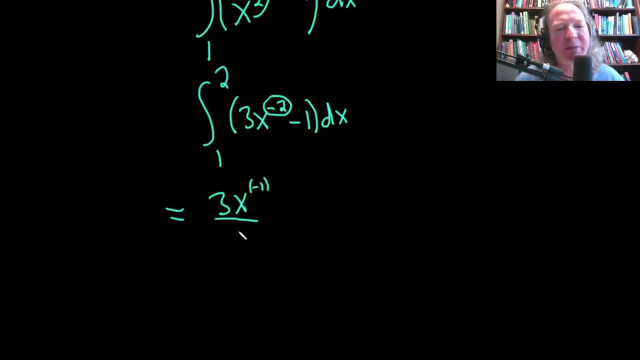 negative 2 is negative 1.. Then we divide by negative 1, minus integrating 1, that's just going to give us x, And this is a definite integral, so we don't need the plus c. I'm going to use a bracket and then I'll write the lower limit of integration here and the upper limit. 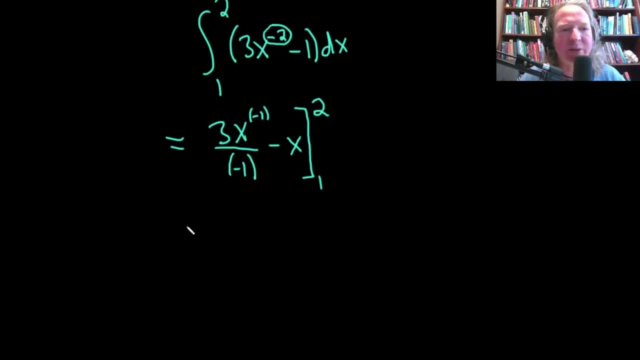 here. Okay, so this is equal to. you can go ahead and put the negative in the front, and I'm going to- actually I'm going to write it like this: I'll write it as negative 3 over x, Basically just taking this and bringing it back downstairs and making the exponent positive. 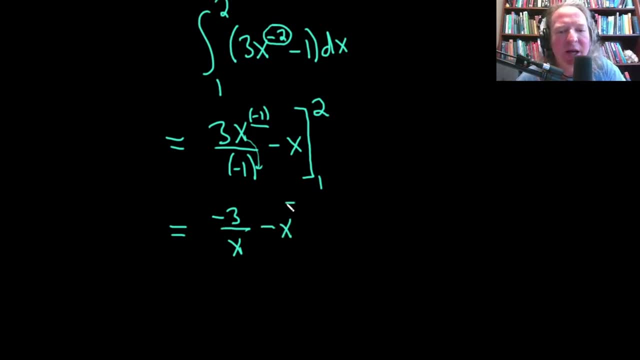 And let's put the negative up top, minus x, and we're going from 1 to 2.. Okay so first we plug in the 2, subtract, then we plug in the 1.. So this is equal to, let's see, plugging in the 2 for all the x's. 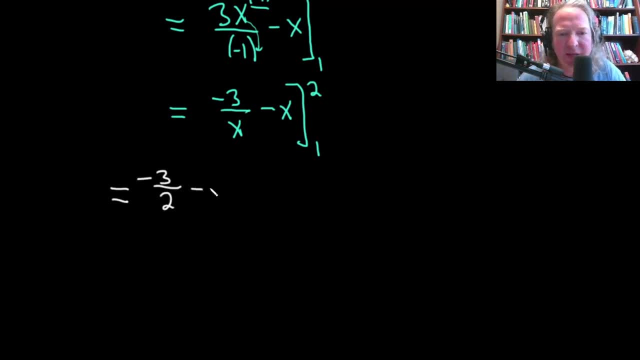 get negative 3 over 2,, minus 2, and minus. now this is two terms, so it's really important to use parentheses. So parentheses negative 3 over x or 1, because x is 1, minus 1.. 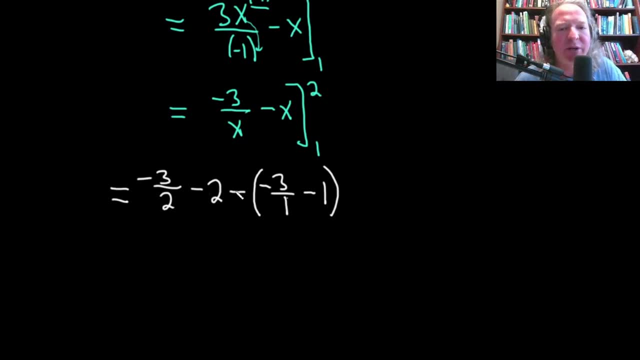 All right. so plugging in the 2,- let's check- 2 here, 2 here, minus- and then plugging in the 1s, everything looks good. Okay, let's clean this up. This is negative: 3 over 2,. 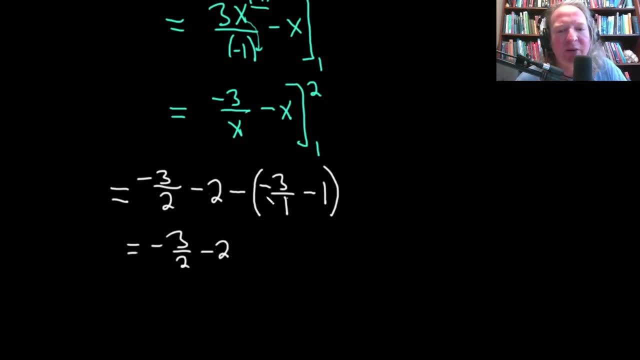 minus 2, and here we have this minus here. I'm just going to leave it out here for a second: Minus 3 minus 1 is minus 4.. Okay, so this is going to be negative 3 halves minus 2, and then plus 4, plus 4.. This is equal to negative 3 halves, and then minus 2 plus 4 is plus 2,. 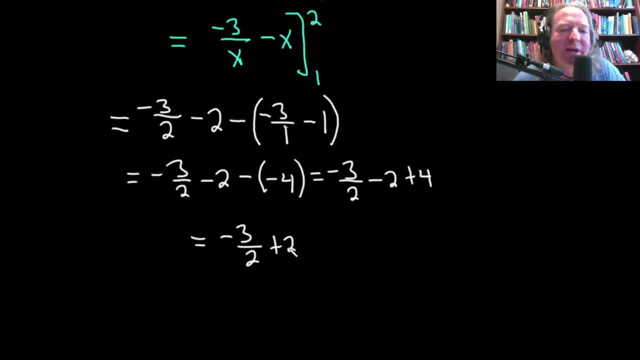 and we have to add these. Easy way to do that is: think of 2 as a number over 2.. So you can write this as negative: 3 over 2, plus 4 over 2.. When you add these, you're just going to get 1 over 2,. 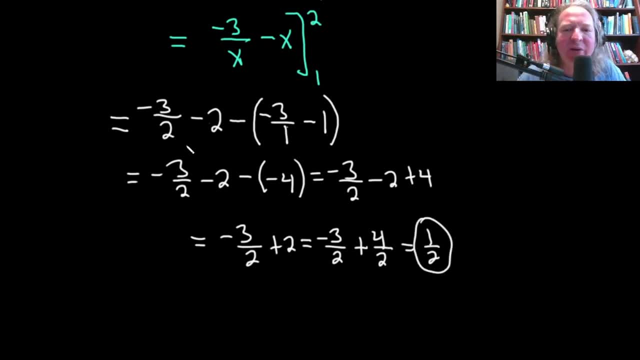 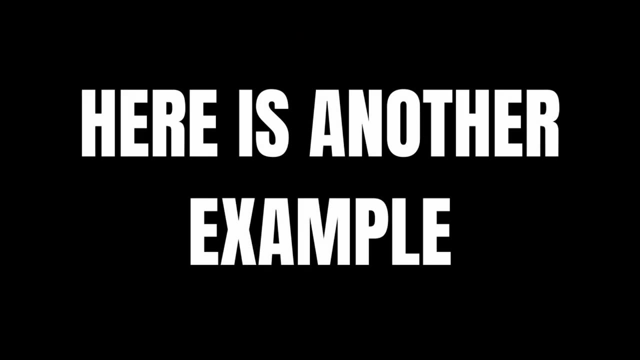 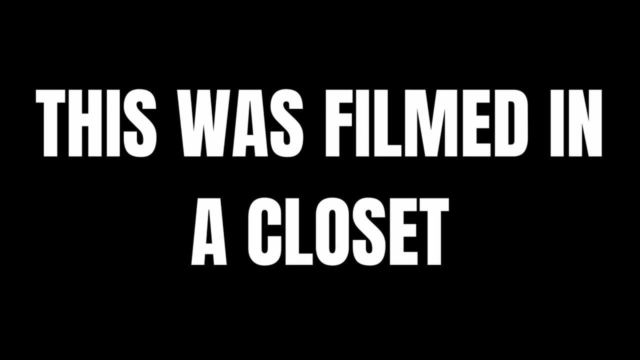 which is the answer to the definite integral. So very, very easy to mess up in this process. So yeah, just got to be careful with these. In this video, we're going to integrate sine x minus 2, and this is a definite integral. 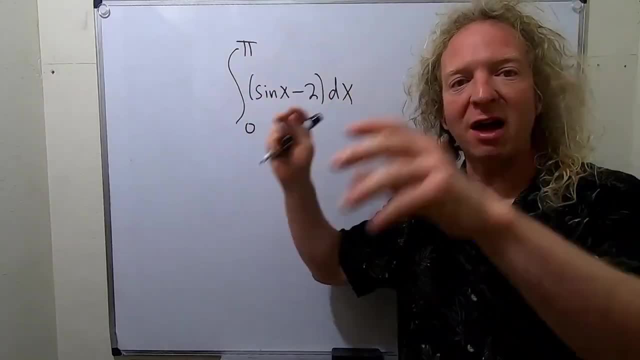 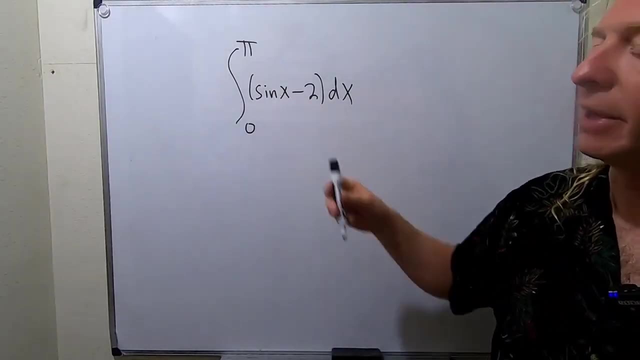 which means that after we perform the integration, we're going to evaluate the results at the limits of integration, So we can just go ahead and jump into it and integrate. So when you're integrating sine, you have to think backwards. So you have to think what is a function whose derivative is sine? 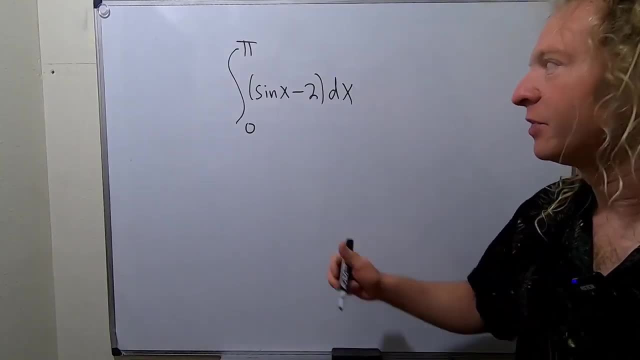 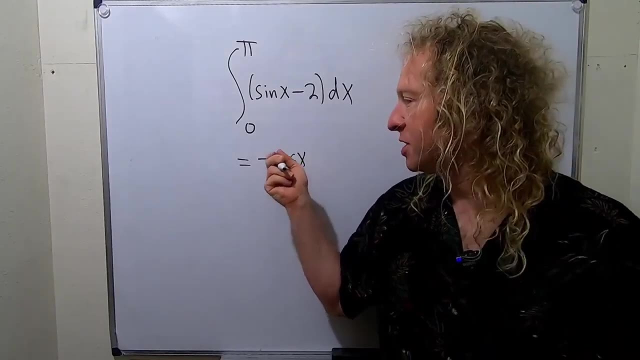 Well, the derivative of cosine is negative sine. So this is going to be negative sine, negative cosine, Because when you take the derivative of cosine you get negative sine and there's a negative here already. so it's like negative, negative, so it's positive. 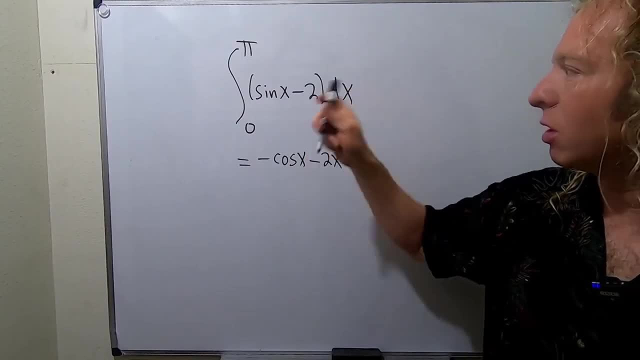 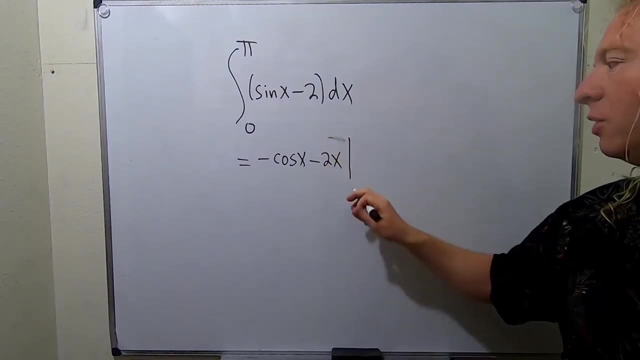 When you integrate 2, you just get 2x and then we're going from 0 to pi. So you can use. there's three choices here: You can use a line, you can use a bracket, or you can use two brackets. 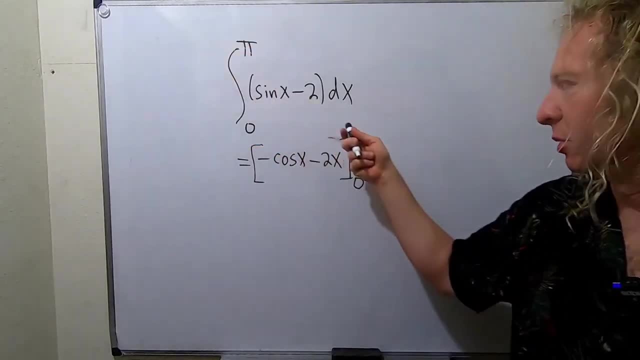 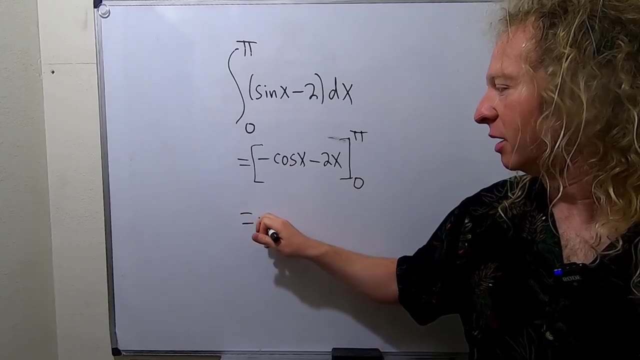 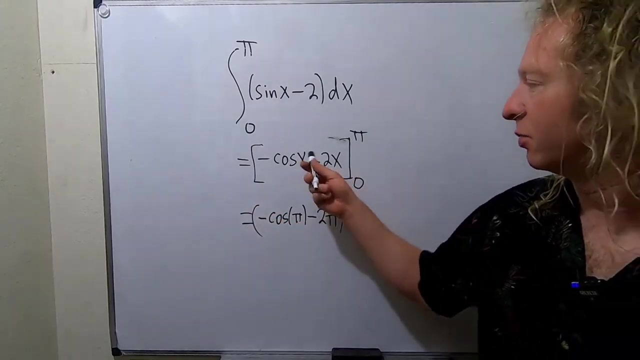 and the 0 goes here and the pi goes up here. so pi, All right, good stuff. So now we plug in the pi first. So plugging in the pi we get negative cosine pi minus 2pi. So this is just replacing all of the x's with pi's at this point. 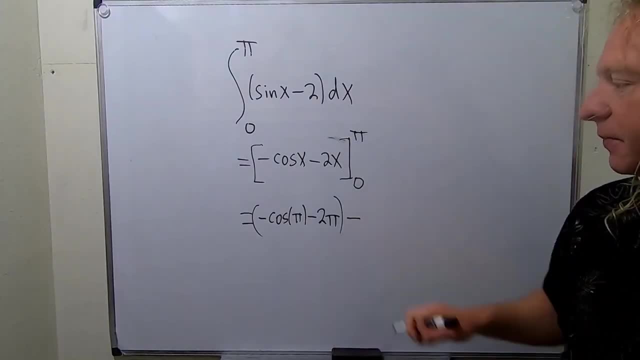 Then you always subtract, no matter what. So minus. Now you plug in the zeros, So I'll put parentheses here. So negative cosine 0, and then minus 2 times 0. I didn't skip any steps, I don't know why. 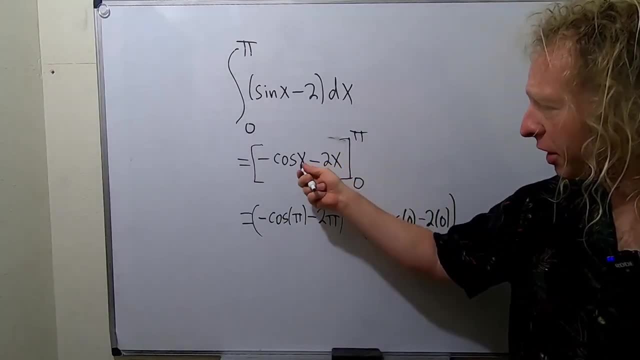 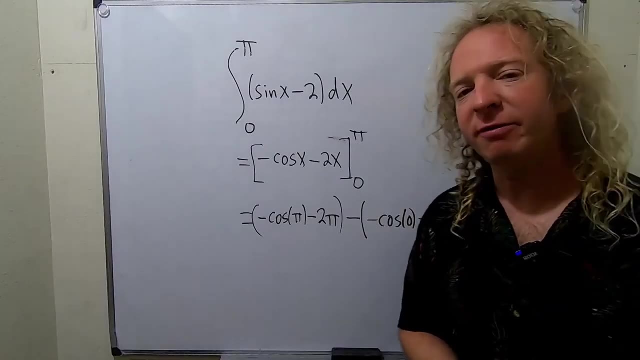 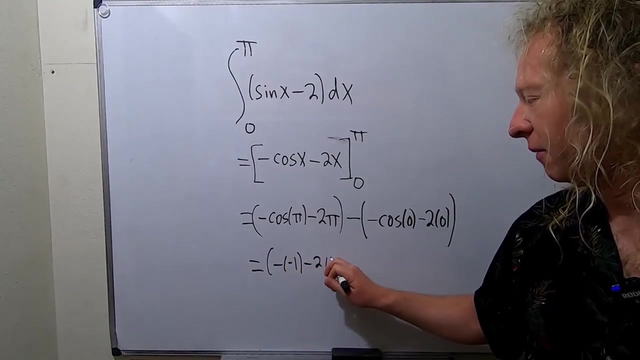 Maybe it's better not to in this example. So first you plug in the pi, okay, Then you put a minus, and then you plug in the zeros: Okay, cosine of pi is negative 1.. So this is going to be negative negative 1 minus 2pi. Cosine of 0 is 1, so this is minus negative 1 minus 0.. I'm showing. 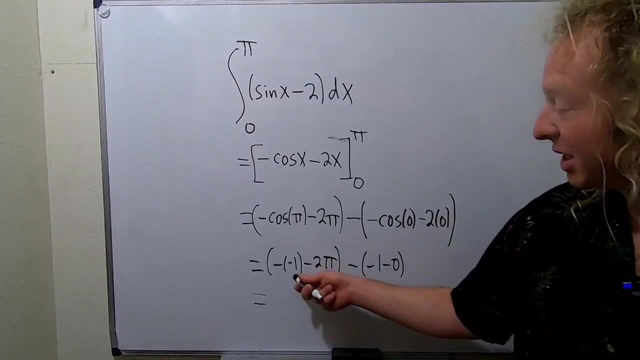 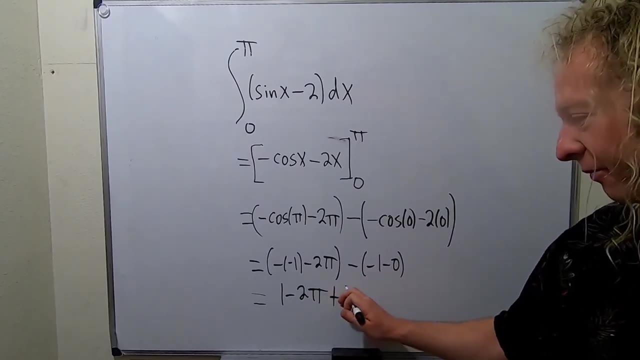 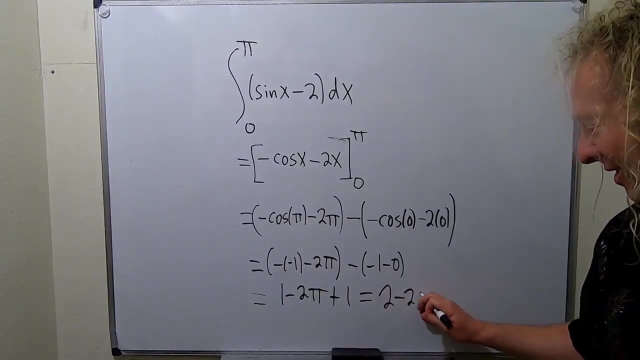 every single step. It's kind of fun. This is 1, right, This is 1 minus 2pi. Interesting, oh, that's fun Plus 1.. And let's not mess up here: 1 plus 1 is 2.. 2 minus 2pi And that. 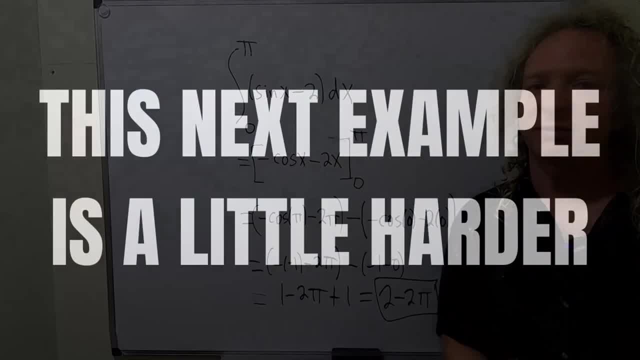 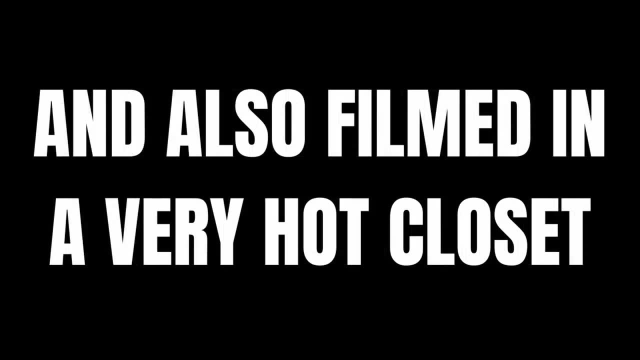 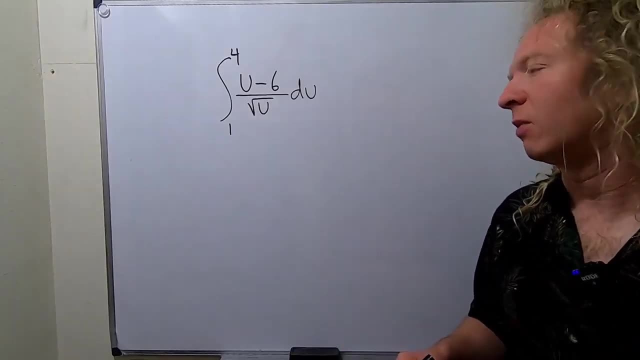 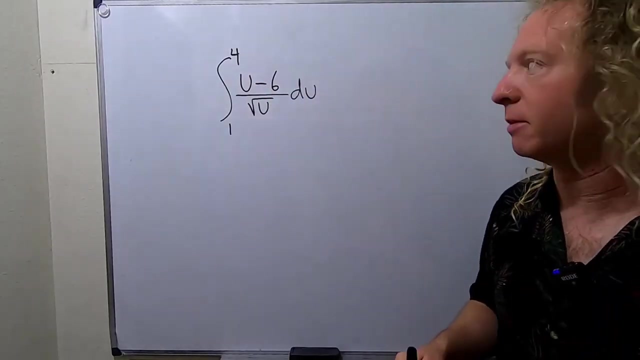 is the final answer. I hope this video has been helpful. Take care: In this video we're going to evaluate this definite interval, So before we do that, we want to write everything As u to a power. You'll notice we have two terms up top and one term on the bottom, So whenever 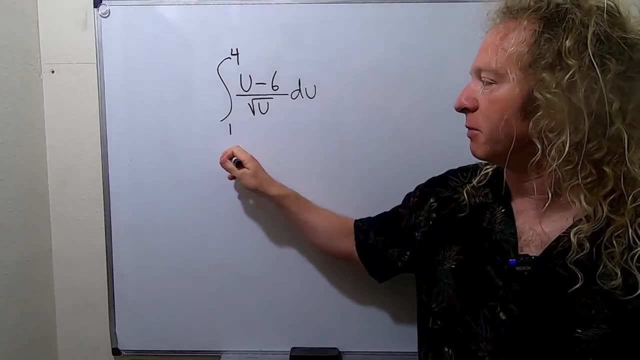 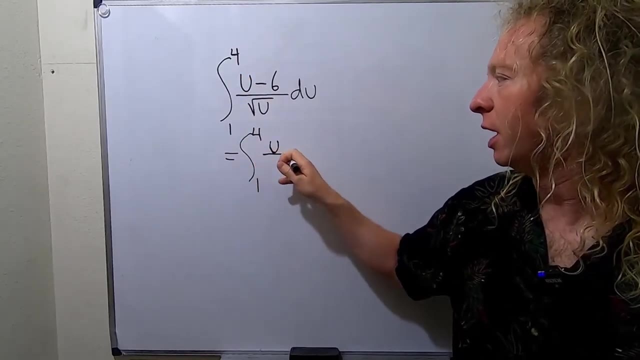 you have that, you want to break it up, So we're going to break it up as follows: So we have the definite integral from 1 to 4.. So it's this over, this, So u over, and I'm going to go ahead and 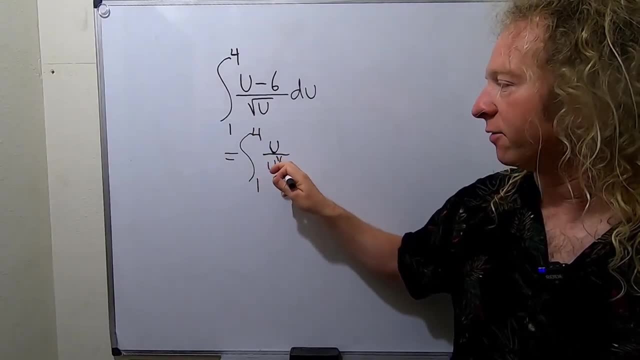 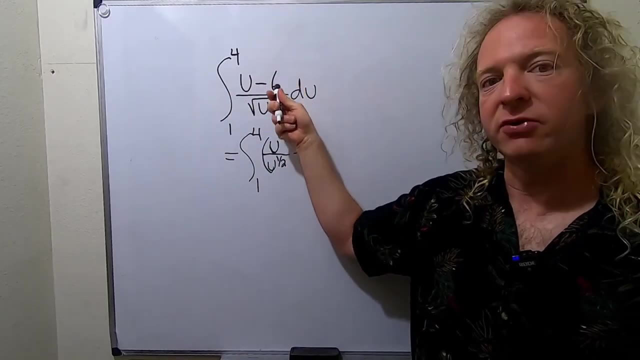 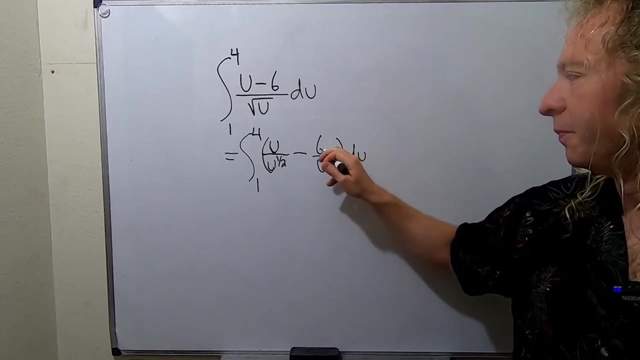 write the square root of u as u to the 1 half. It'll just make it easier to simplify. So it's u over this minus and then this over this, So it'll be 6 over u to the 1 half, And then we have our du here. 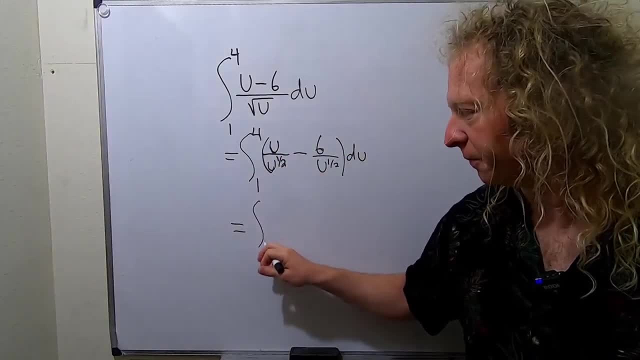 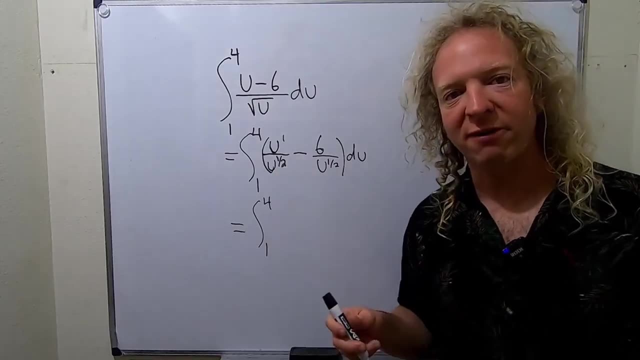 OK, now we can simplify this, So we still have the definite integral. So what you do here is you subtract the exponents, You have u to the first power, and then here you have u to the 1 half, So you do 1 minus 1 half, so you get 1 half. So this is u to. 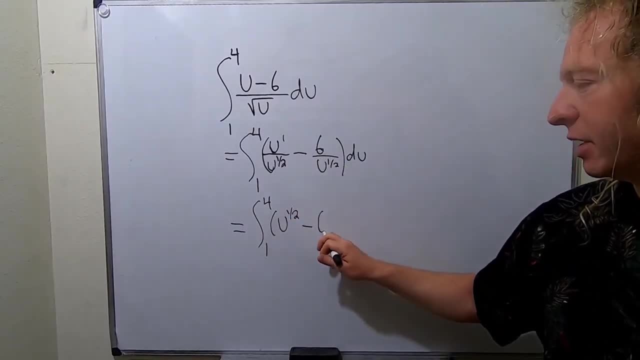 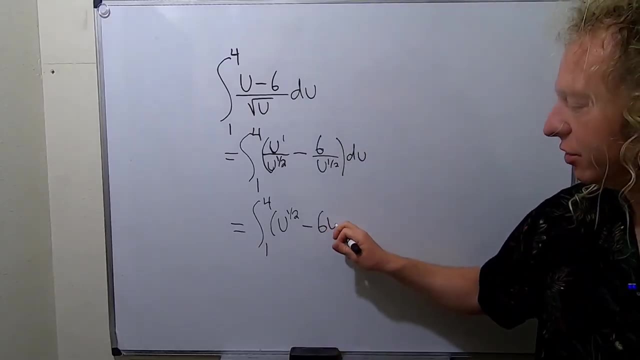 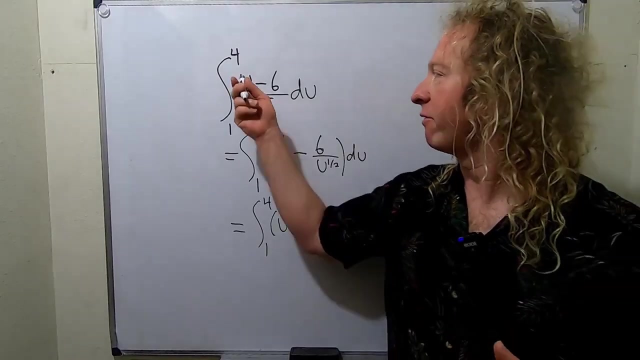 the 1 half minus and then 6.. Then you can take this and you can bring it up, And when you bring it up the exponent becomes negative. So this is u to the negative 1 half and then we have our du. So again, whenever you have like 2 or 3 or more terms up top and a single, 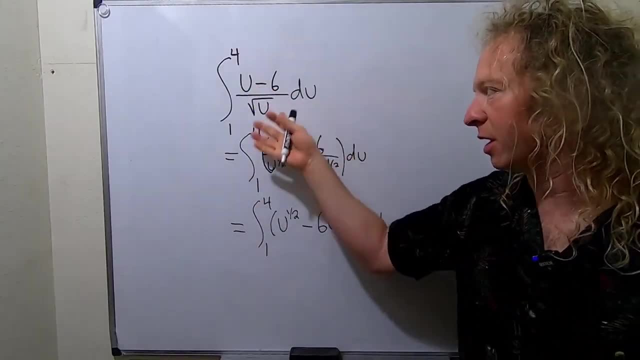 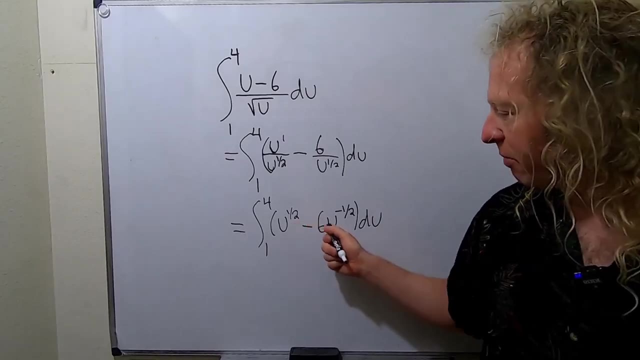 term on the bottom that should automatically come to mind. Can you break it up using this strategy? So it's super, super useful. OK, so now we're just going to integrate. So when you integrate both of these pieces, you just use the power rule, So you add 1 to the exponent. 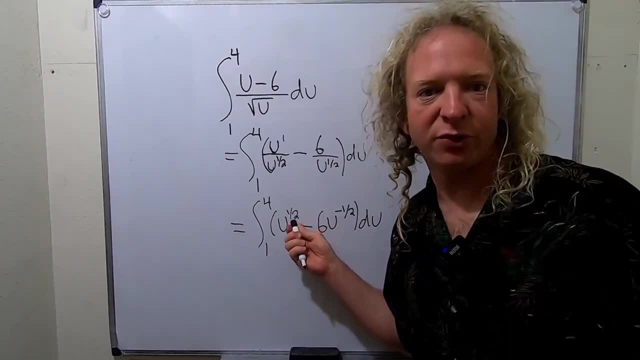 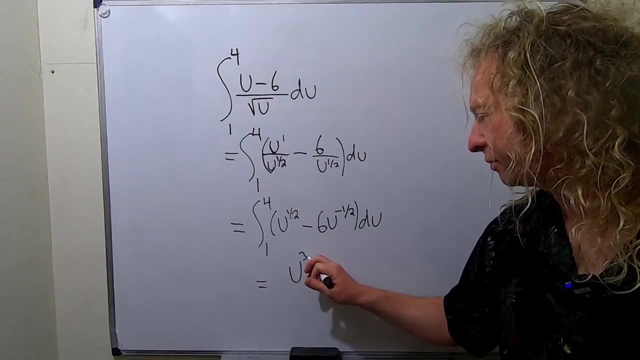 and divide by the result. So we have 1 half plus 1.. So it's really 1 half plus 2 halves, So that's 3 halves. So this is u to the 3 halves. Then when you divide by 3 halves, you really multiply by the reciprocal. 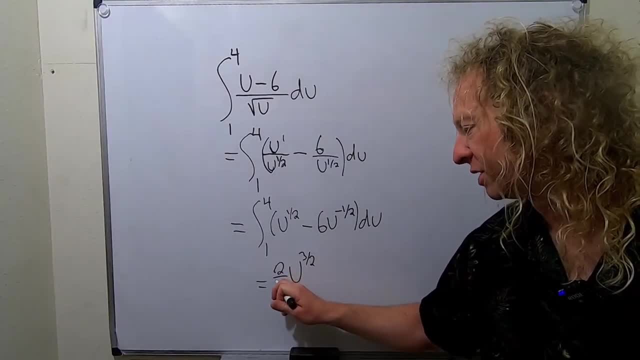 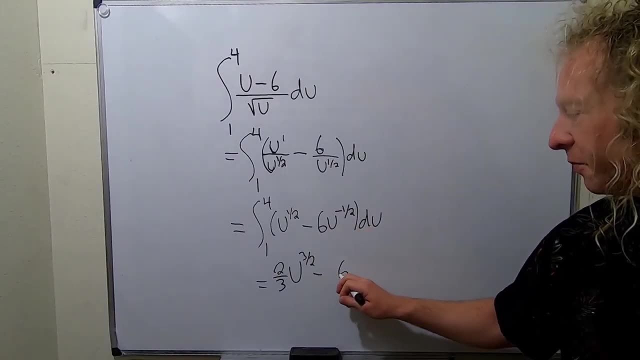 So instead of dividing by 3 halves, I'm going to put a 2 thirds here, because that's the reciprocal. OK, the same thing here. So now this one. it's minus. I'm going to leave some room here- 6. Notice, I'm leaving some room here for whatever is going to go here. So 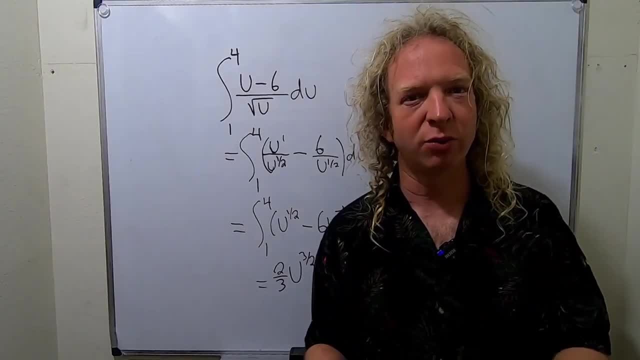 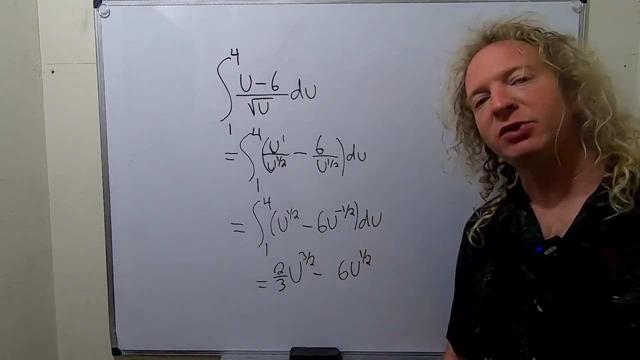 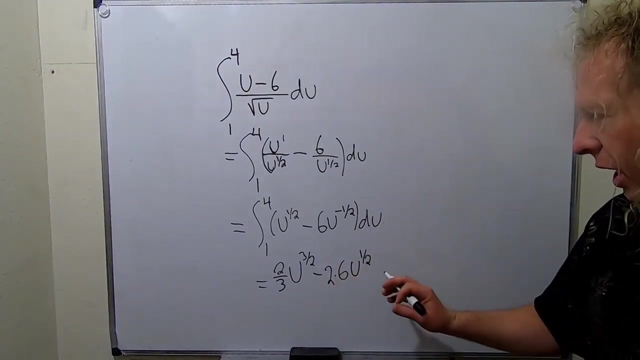 we're adding 1 to this, So negative 1 half plus 1 is 1 half. So this is u to the 1 half. And then again: dividing by 1 half means we multiply by 2.. So times: 2.. OK, and then you have three choices here. 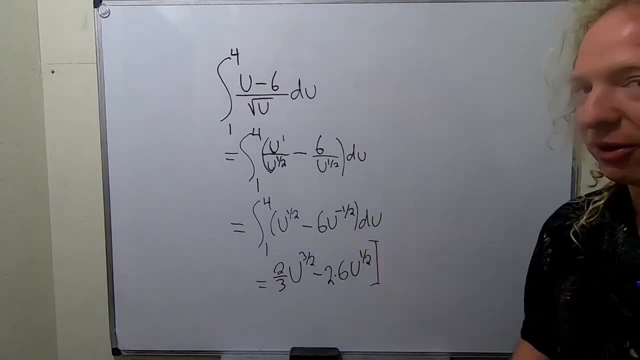 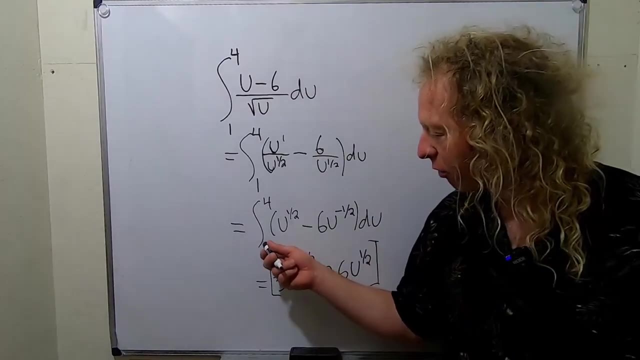 You can put a line, you can put a bracket, or you can go all out and do 2 brackets. It just depends what you're comfortable with. So, line, bracket or 2 brackets, And we're going from 1 to 4.. 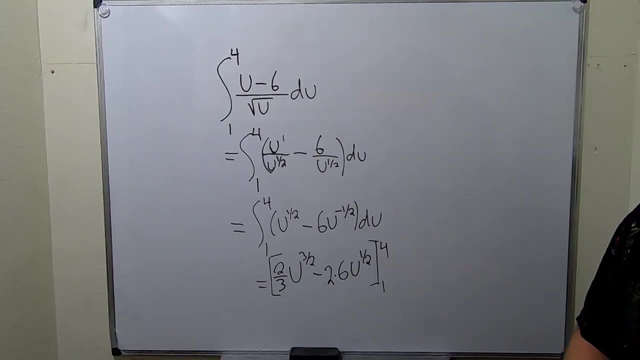 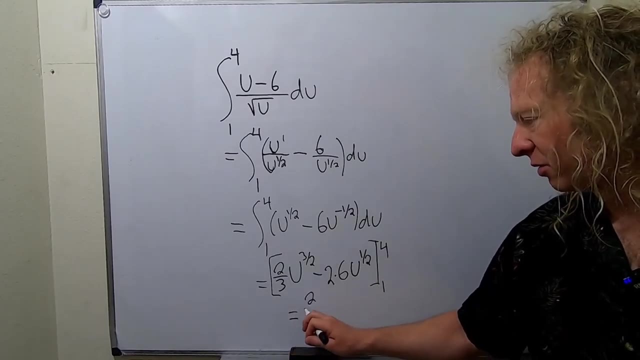 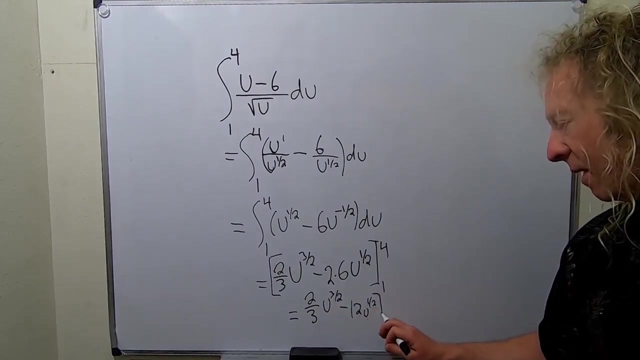 So then you put these numbers here. These are called the limits of integration. All right, I'm going to go ahead and clean this up a little bit, So I'm going to write this again: This is 2 thirds? u to the 3 halves, minus 12? u to the 1 half, And then we have 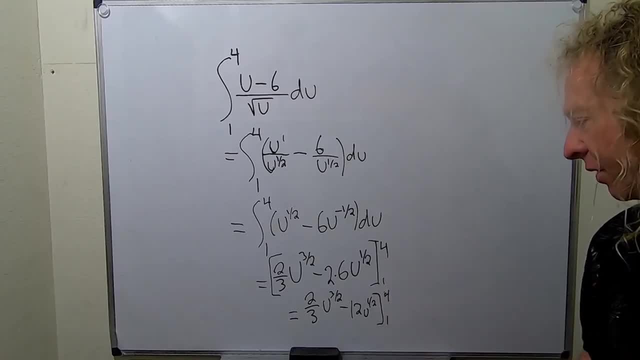 our limits. Let me just write it again: 1 to 4.. All right, so first you always plug in the top numbers. It's always the top number first You subtract, then you plug in the bottom number. So plugging in the top number first, we get 2 thirds, 2 thirds 4 to the 3 halves. OK, 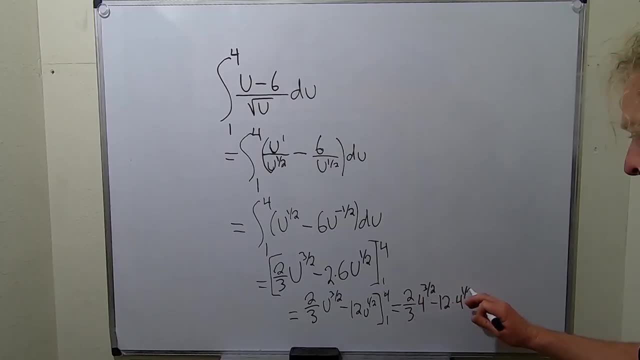 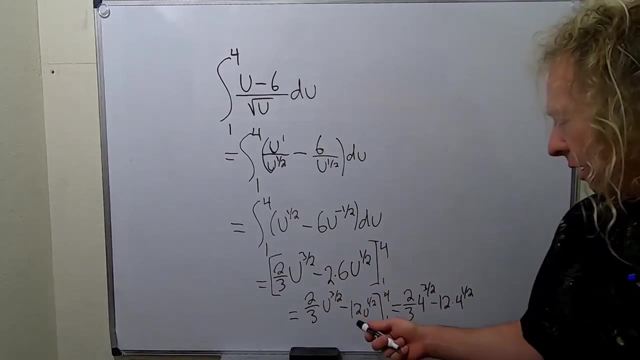 Minus 12,, 4 to the 1 half. So all I've done so far is simply put a 4 wherever there is a? u Let's check that. So 2 thirds, 4 to the 3 halves, check Minus 12, and then 4 to the 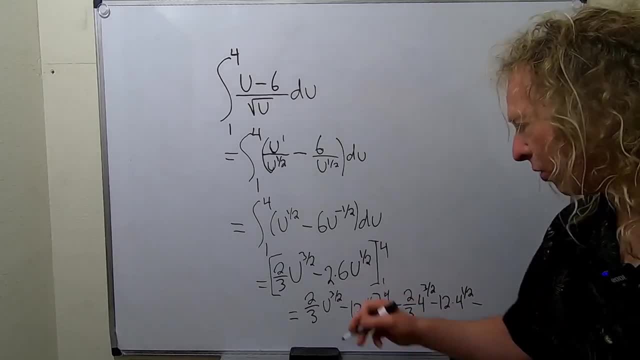 1, half check Minus. And now we have to plug in the 1s. That's going to be a little bit easier, because whenever you put a 1 where the u is, it's just going to become 1. Because 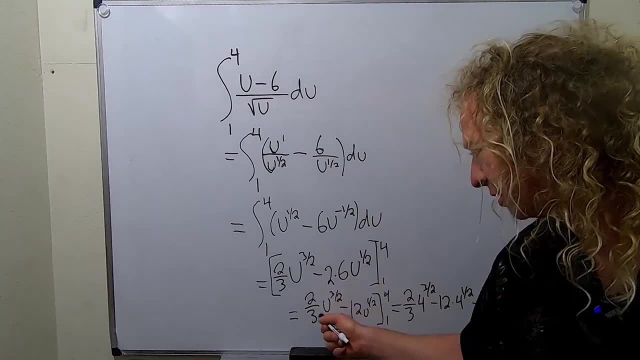 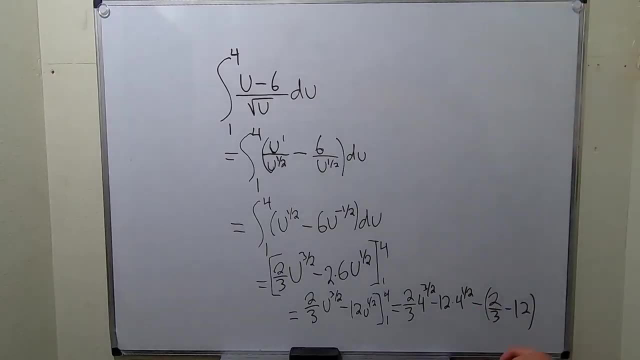 u to the 1 half is 1.. u to the 1 half is 1.. So I'm just going to get 2 thirds minus 12.. So 2 thirds minus 12.. Yuck, Typically you get fractions in these problems, So that's. 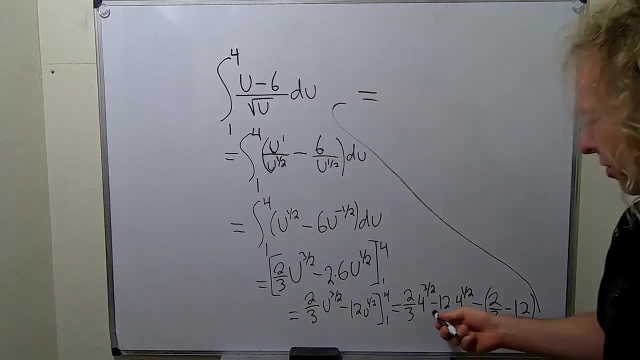 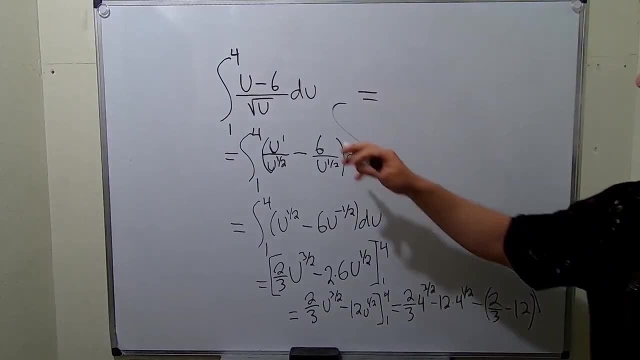 probably the most annoying part about these problems is the fractions. OK, So I don't have a calculator in my hands, So I have to do it all by hand. So 4 to the 3 halves. So here's the old school way, or here's how I do it. I don't know if it's the old school. 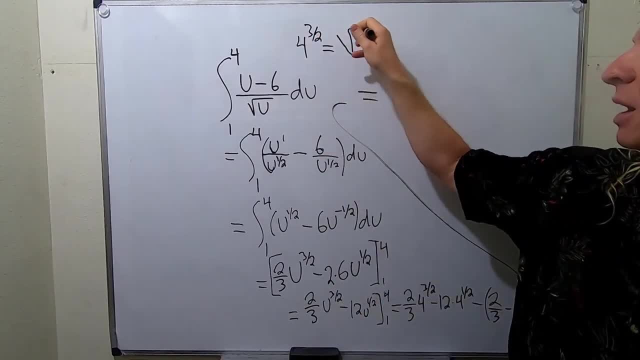 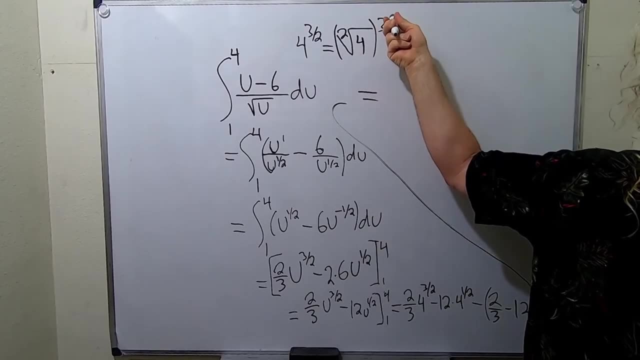 way. Maybe it's new school, So the 2 goes in the little pocket always. Every time you put the 2 in the pocket, the 4 goes here And you can put the 3 on the outside, Or you can put it on the inside too, but it's better to put it on the outside. 2 goes in the pocket. 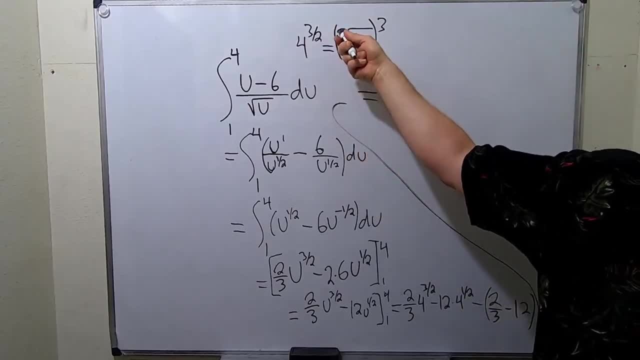 always: 2 goes in the pocket. 2 goes in the pocket. 2 goes in the pocket. Put the 4 there, The 3, you can put it on the outside or the inside. Square root of 4 is 2.. So you get 2. 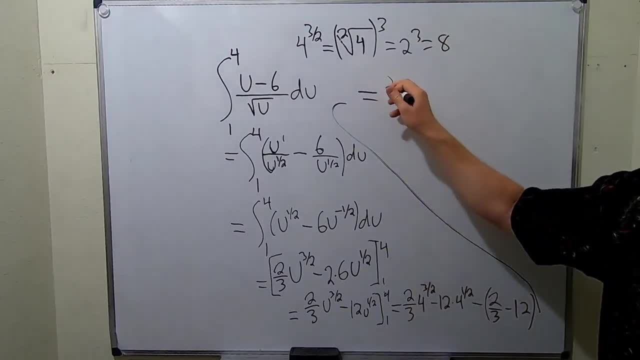 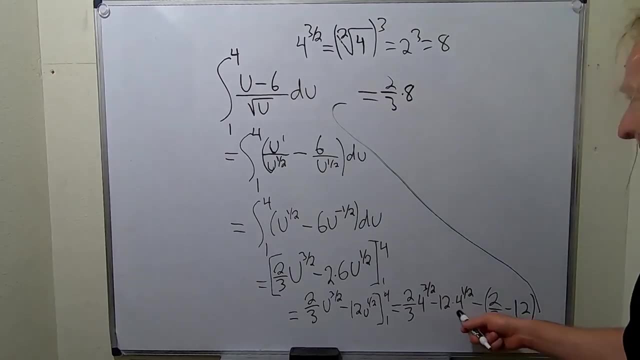 cubed, So you get 8.. Boom, So that's 2 thirds times 8.. 2 thirds times 8.. That's beautiful, Minus. Oh, square root of 4 is 2.. That's easy, right. So 12 times 2. That one's not so bad. 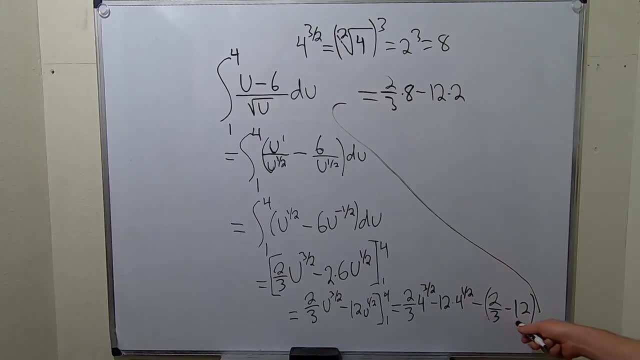 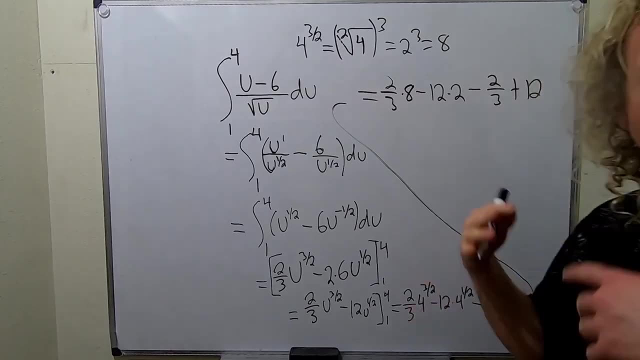 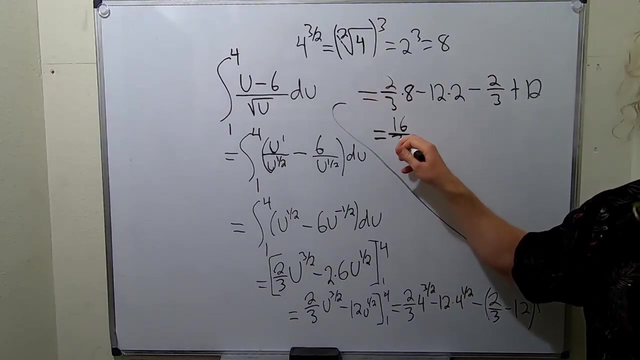 Here minus 2 thirds minus 12.. I'm just going to distribute it, So it'll be minus 2 thirds plus 12.. Let's just put it all together before we start adding fractions. Let's see what arises from all of this. So here we have 16 thirds. 16 thirds minus 24.. Minus 2 thirds. 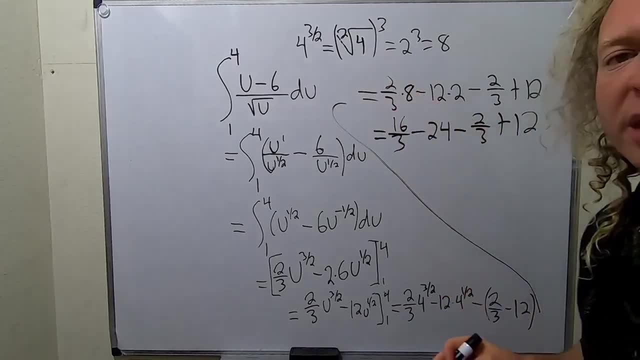 plus 12, right. So just multiply the 2 and the 8. And let's see: Sixteen thirds minus 2 thirds is 14 thirds. That's combining this 1 and this 1.. Negative: 24 plus 12 is minus. 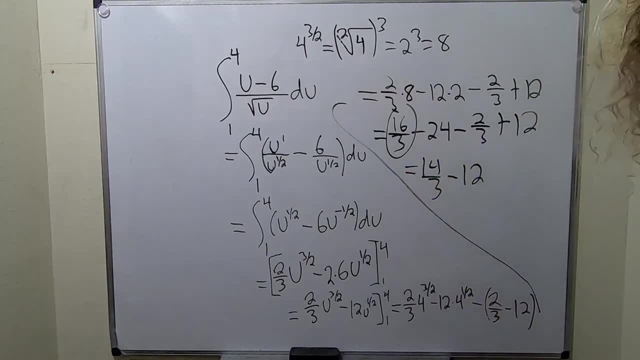 12.. To finish this computation, we want to write 12 as a number over 3.. So we can multiply it by 3 over 3.. So this is 14 thirds minus 36 thirds. 14 minus 36 is negative 22 thirds. 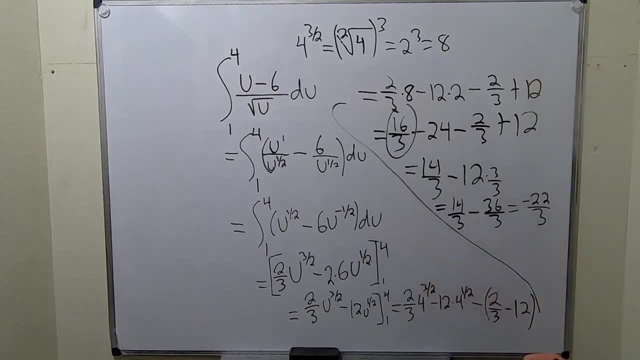 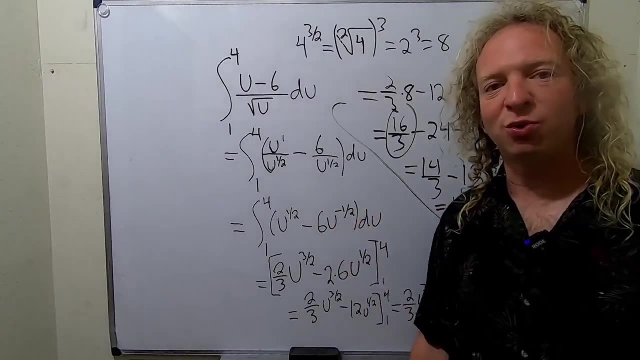 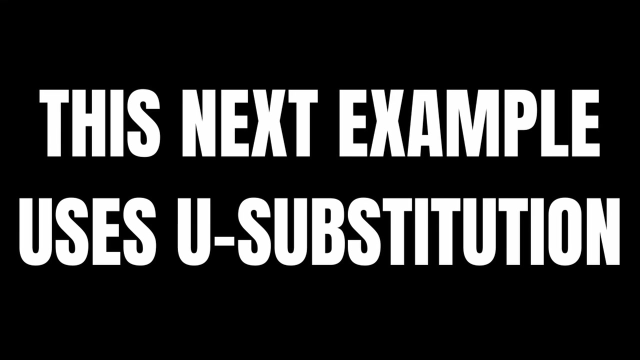 Yeah, that's right. Yeah, because 36 minus 12 is negative 22 thirds. So, like I said, 14 is is 22, and so that should be the final answer. I hope this video has been helpful to anyone who is working on some calculus. take care, video we're going to. 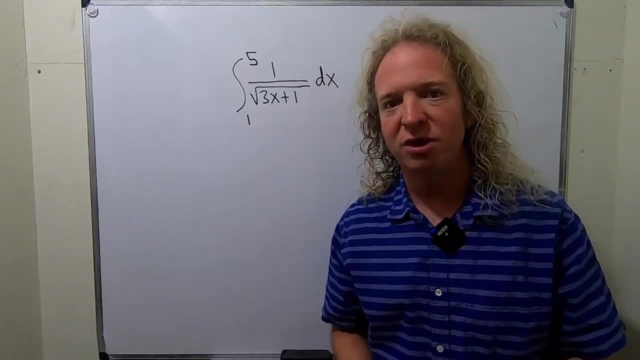 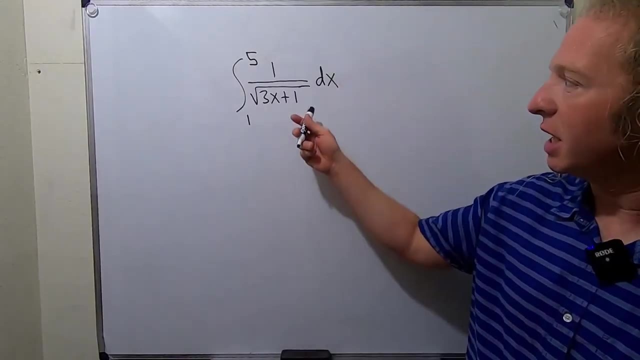 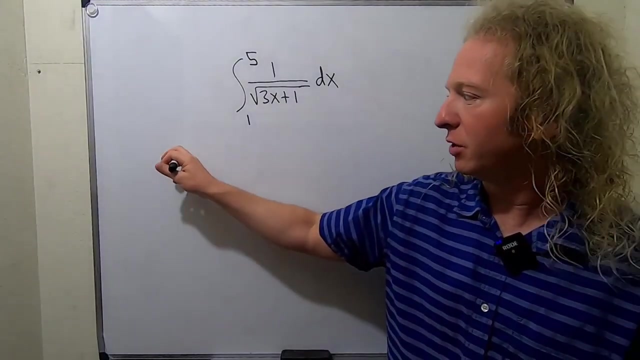 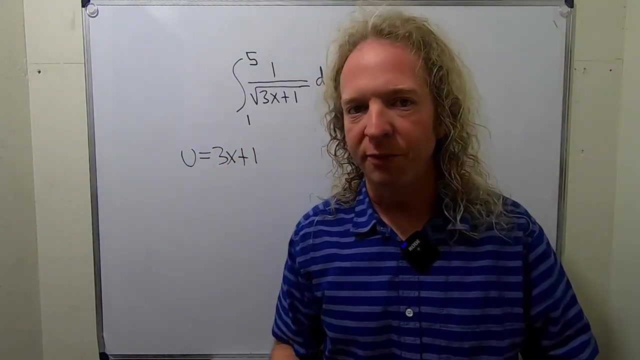 evaluate this definite integral using you substitution. so whenever you're using you substitution, usually you is your inside function. so in this case a good first attempt for you is the piece inside the square root. so we'll start by letting u equal to 3x plus 1. then you always compute du as normal. so du is the. 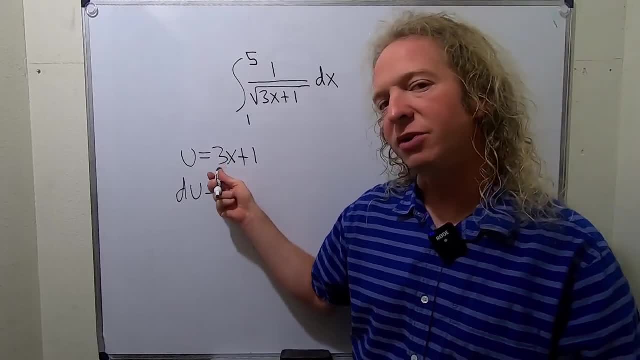 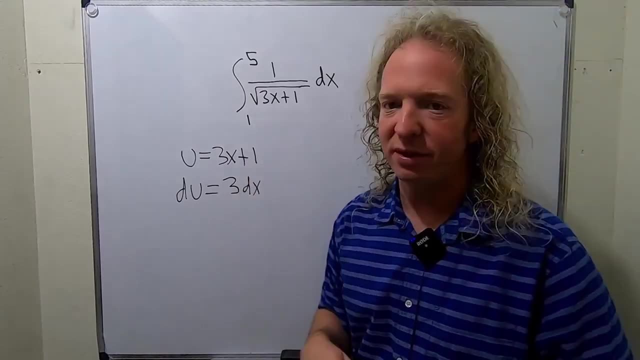 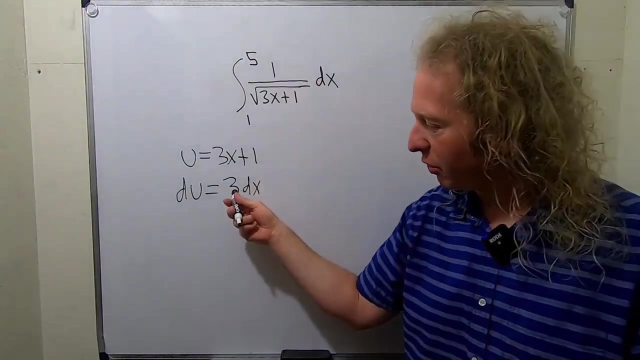 derivative of u. so du, here we compute this derivative. the derivative of X is 1, so we simply get 3 DX and the derivative of 1 is 0. then, when you get to this step, you're always supposed to make this look like this: so here we have 3 DX and here we have 1 DX, so we 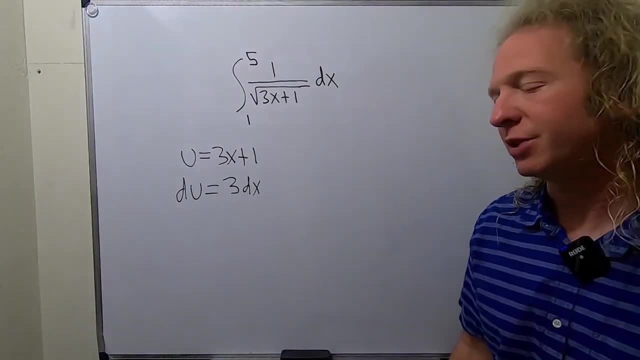 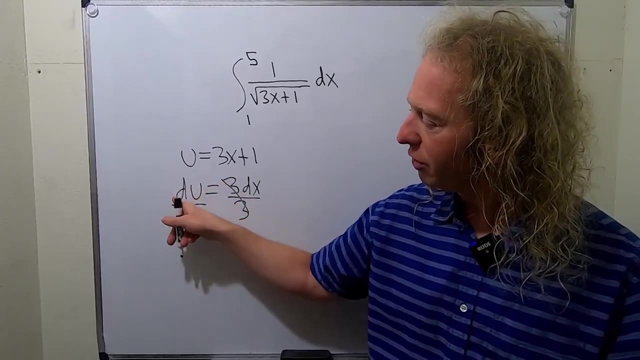 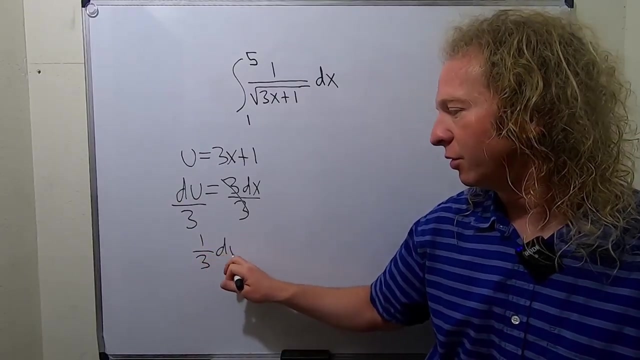 have to get rid of the 3. so to do that, we'll just divide both sides by 3. so divide by 3, divide by 3, so we end up with du over 3. typically, what we do in this point, at this point, is write it like this: 1 third du equals DX, because 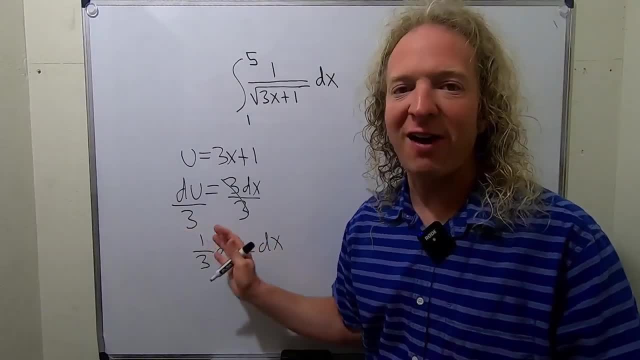 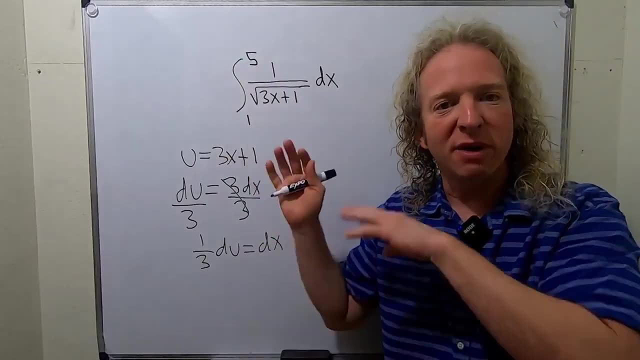 in the next step, when we make the substitution, we're going toúltie 27, just in case I'm missing out. so that's okay, but what we typically do is factor out the constants, okay. so if this was an indefinite integral, like if they didn't have these numbers, we would just go ahead and make. 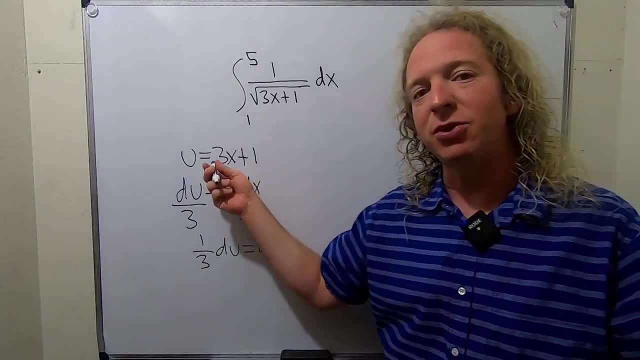 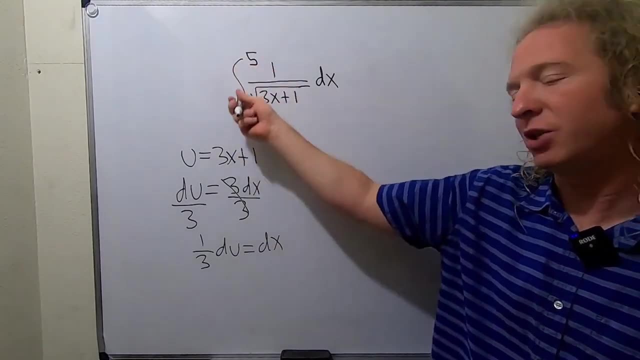 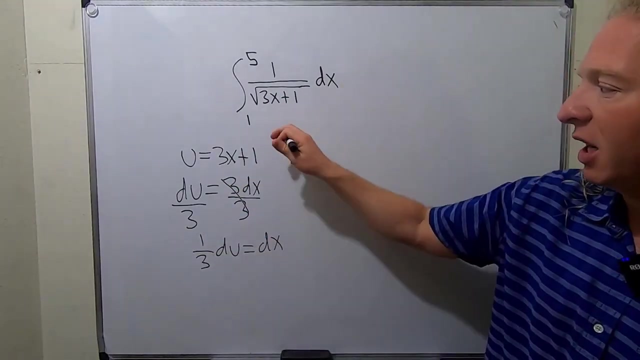 the substitution. however, this one has limits of integration. so whenever you make a u substitution and you have limits of integration, you have to change them. so these are X values, right, because we're integrating with respect to X, we are converting to you. so we have to turn them into u values. so let's. 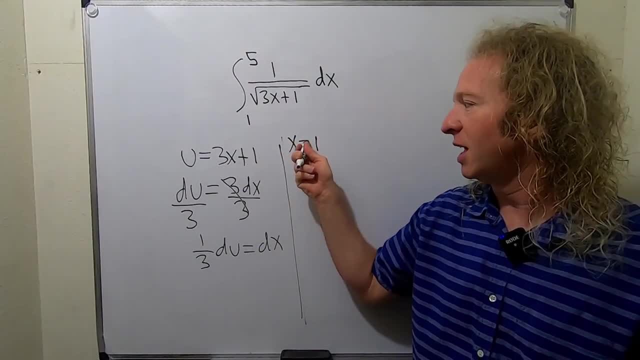 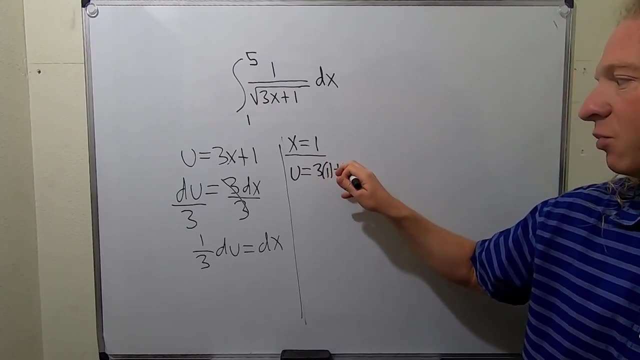 So when x is equal to 1, we're going to take the x and plug it in here and that will give us the u. So u equals 3 times 1 plus 1.. 3 plus 1 is 4, so there is our u. 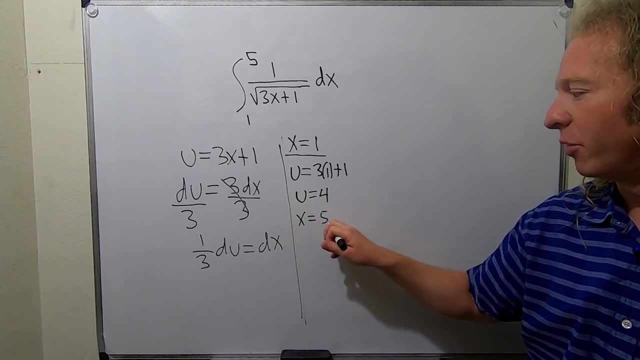 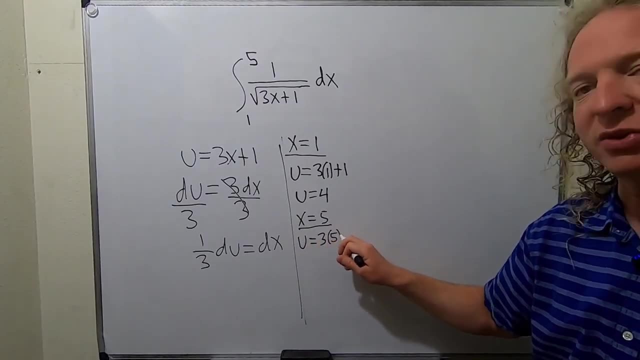 And then when x is 5, we end up with, let's see: x is 5, we get 3 times 5.. So u equals 3 times 5 plus 1.. So you get 15 plus 1, so we get 16.. 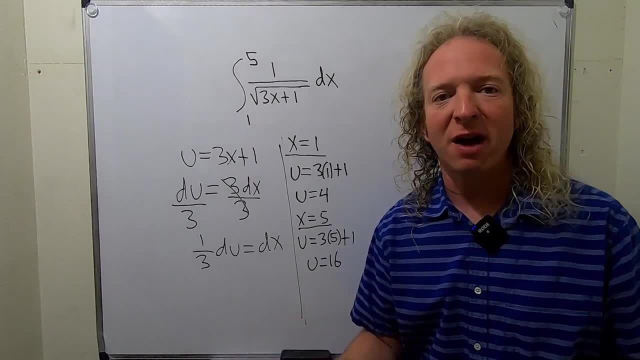 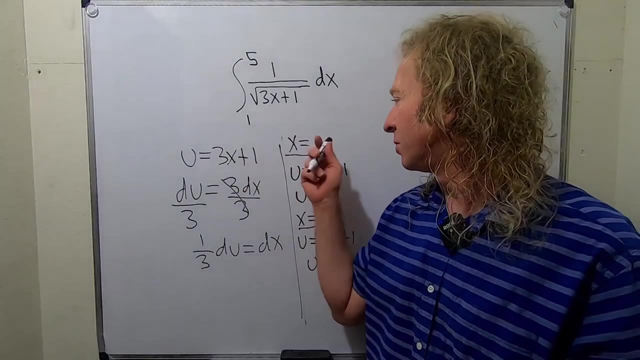 This is a super important technique. I once got stuck on a math problem for over a week because I didn't do this. This was the missing step, so it's so, so important. So when x is 1, u is 4.. 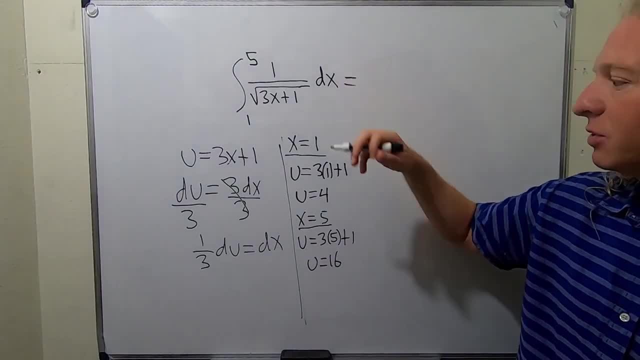 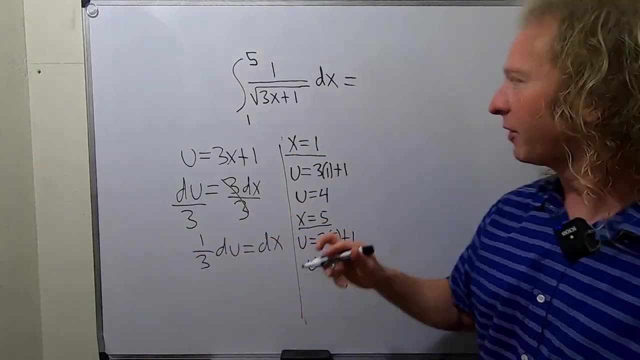 When x is 5, u is 16.. All right, now we're going to make the substitution and we're going to change everything. So let's see, Let's be careful. So the dx is 1 third du, so we can pull out that 1 third. 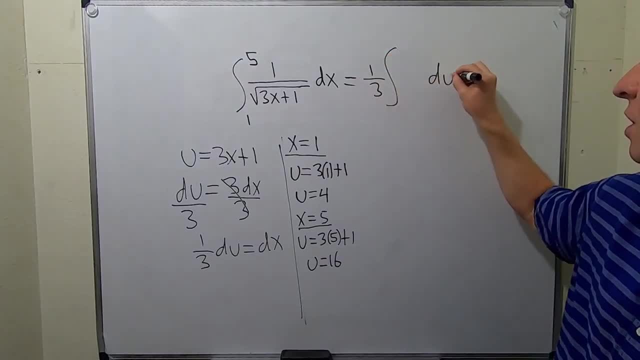 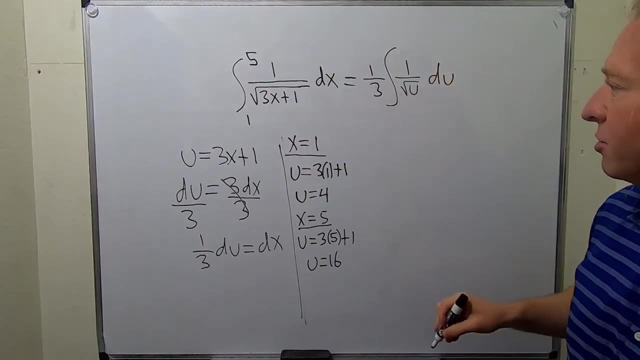 So 1, third. Then we have the du, Then we have the 1 up top. On the bottom we have the square root of u, And then our limits are now u values. Let's see: When x is 1, u is equal to 4.. 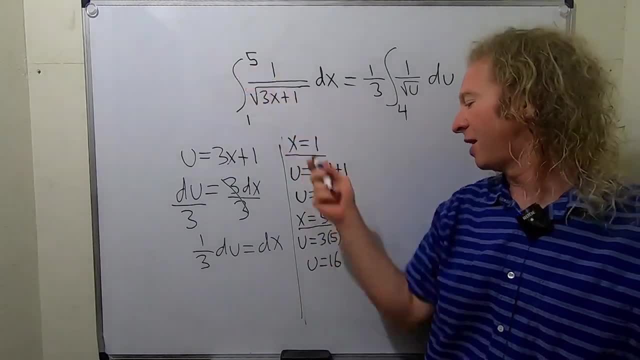 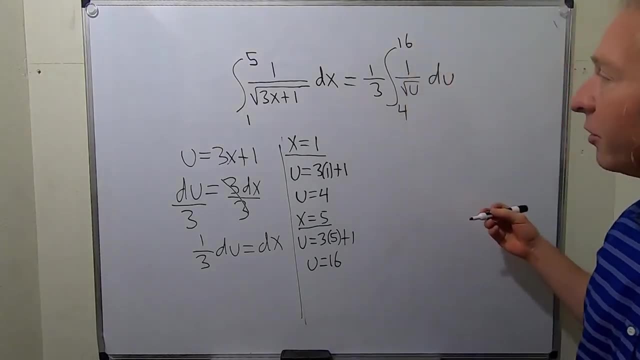 So this becomes a 4.. And when x is 5, u is 16.. So this becomes a 16.. Really, really, really nice. Okay, so now we have to integrate it. So basically, this is 1 over u to the 1 half. 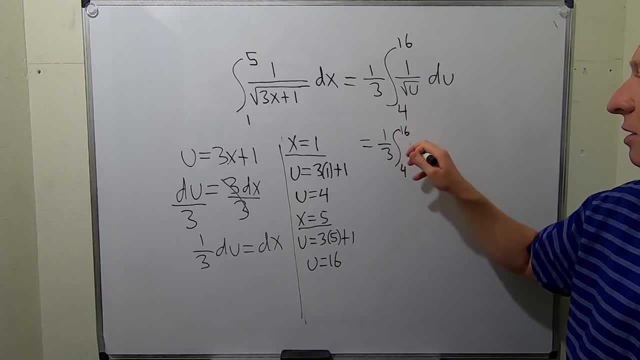 So what you do Is rewrite it like this: 1 over u to the 1 half. I was going to skip a step, but I didn't. The step I was going to skip is I was going to bring it upstairs. So when you bring it upstairs, what happens is the exponent becomes negative. 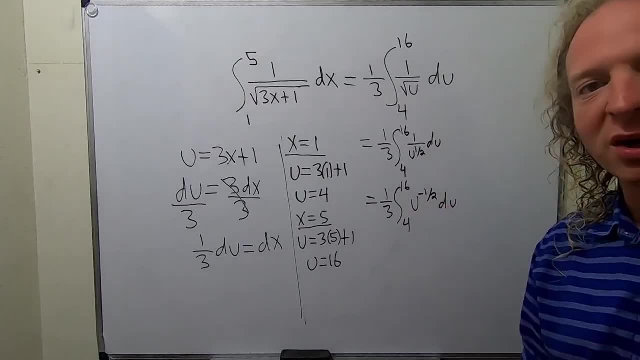 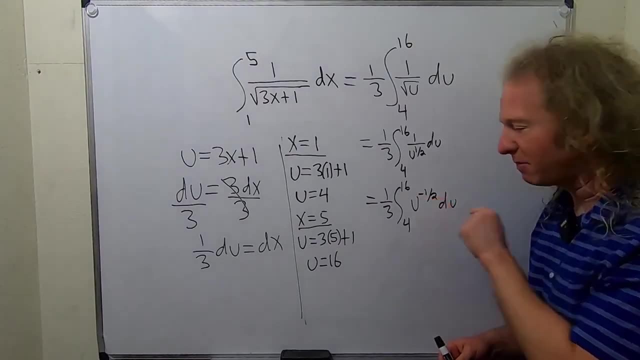 And so the reason you do that is because to integrate this, you want to use a formula, So you want to use the power rule, So now we can do that. So, basically, you add 1 and divide by the result, So this is equal to 1. third, 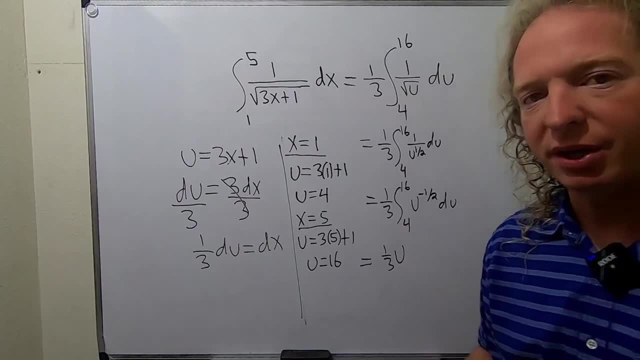 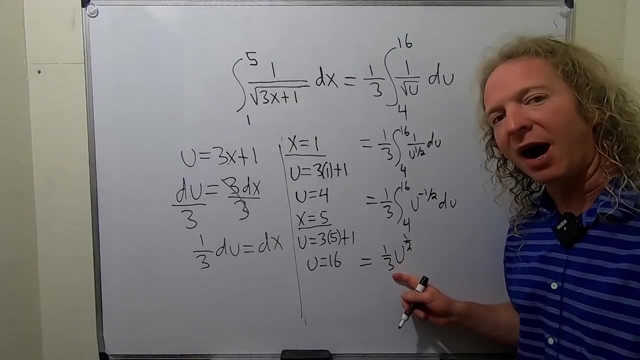 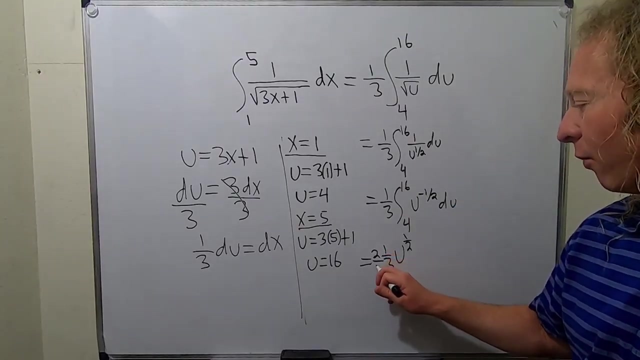 So this is equal to 1 half. u negative 1 half plus 1 is 1 half, so this is 1 half. And then we're dividing by 1 half. When you divide by 1 half, you really multiply by the reciprocal. so 2 over 1, so 2 over 1.. 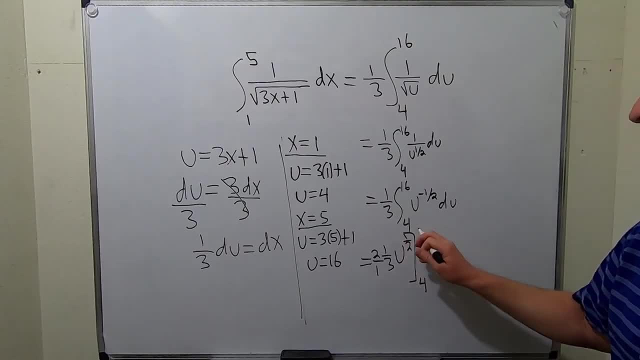 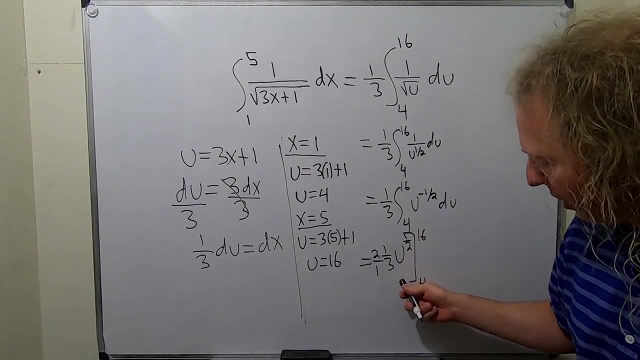 And then we're going from 4 to 16, so from 4 to 16.. Again, we add 1 to the negative 1 half. so we get 1 half. We divide by 1 half. But when you divide by 1 half you really multiply by the reciprocal. 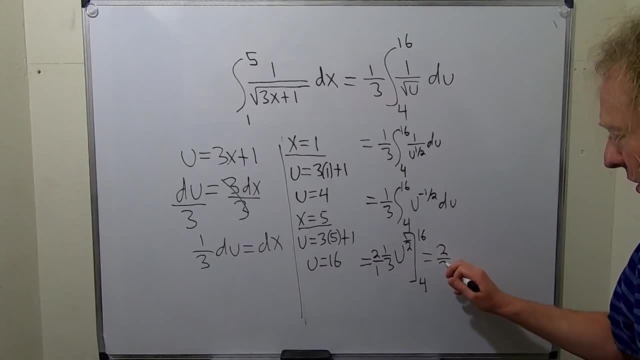 All right, let's clean this up a little bit. This is 2 thirds And I guess now we can plug in the numbers. So you plug in the 16. So you get 16 to the 1 half, You subtract and then you plug in the 4.. 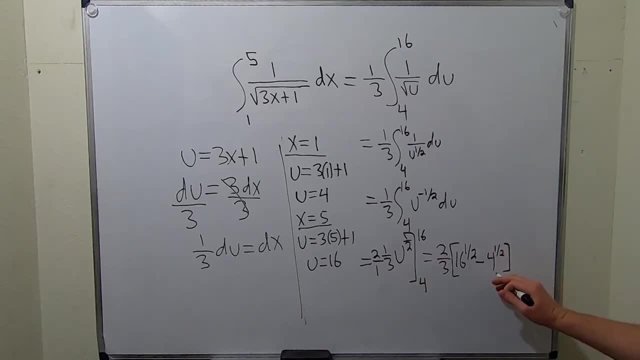 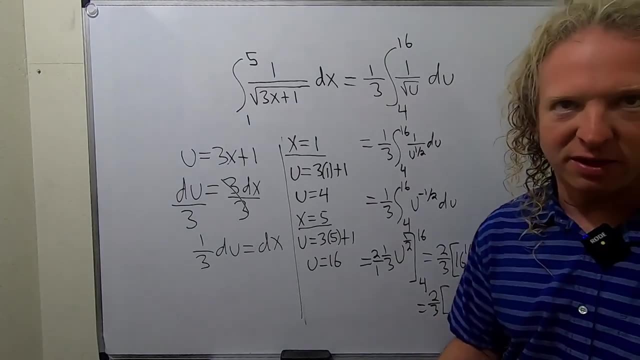 So you get 4 to the 1 half. So this is 2 thirds. It's working out quite nicely. 16 to the 1 half is the square root of 16.. That's going to be 4.. 4 to 16 is 4.. 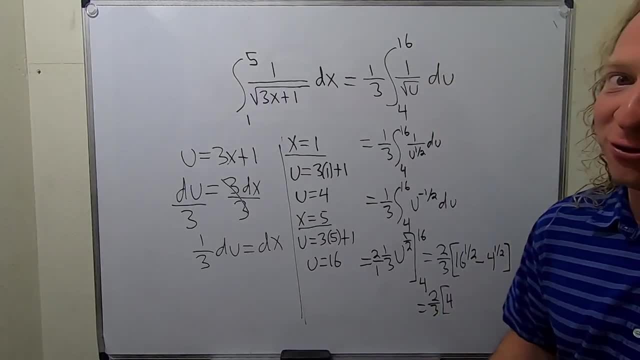 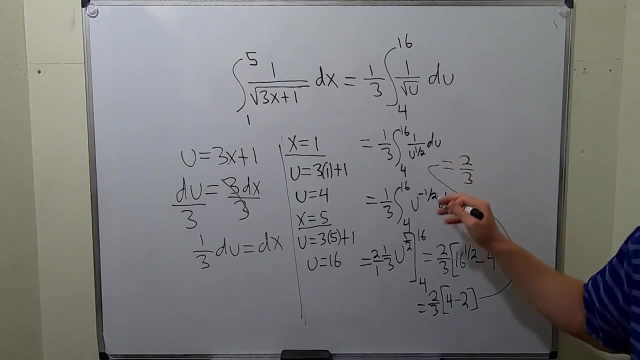 And 4 to the 1 half is the square root of 4, which is 2.. So you get 4 minus 2.. It's a really bad place to get stuck. So this is 2 thirds. 4 minus 2 is 2.. 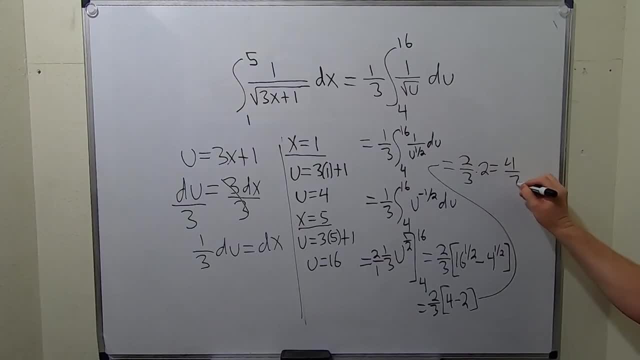 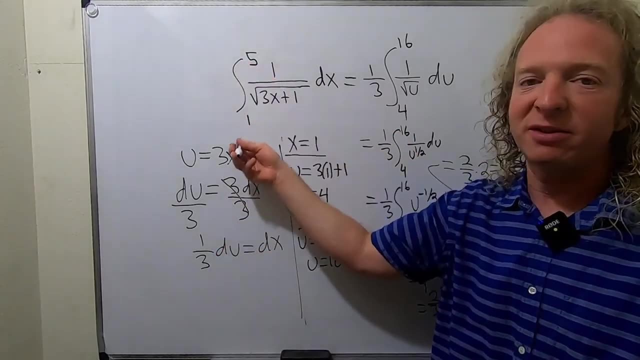 So we get times 2.. 2 times 2 is 4.. So we end up with 4 over 3.. And that's it. So the key point is, whenever you have a U substitution and you have limits of integration like this, 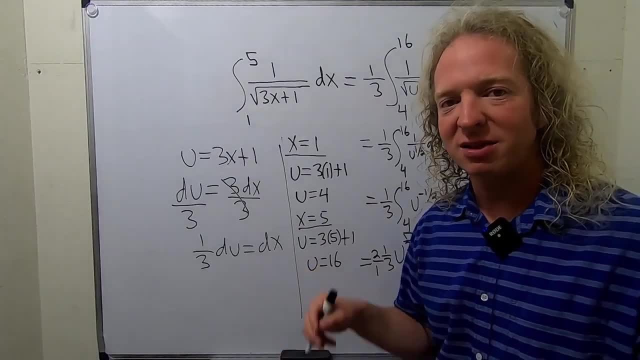 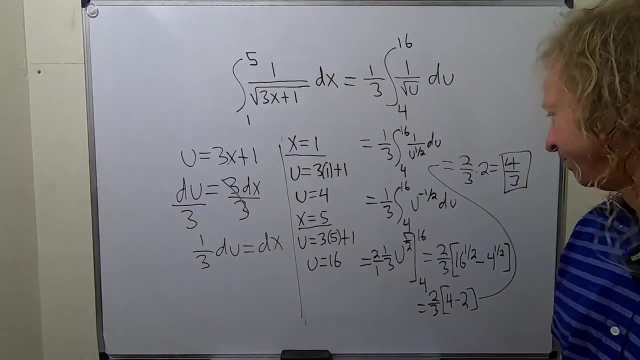 you're supposed to change them. This is something that comes up in all calculus classes. It's really really important. It's a really really useful technique. It comes up in other math as well, like a lot. So yeah, that's it. 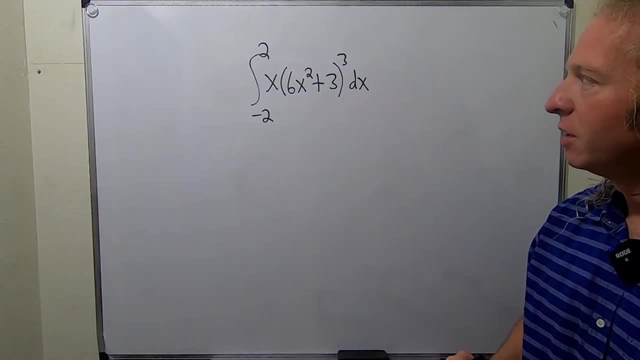 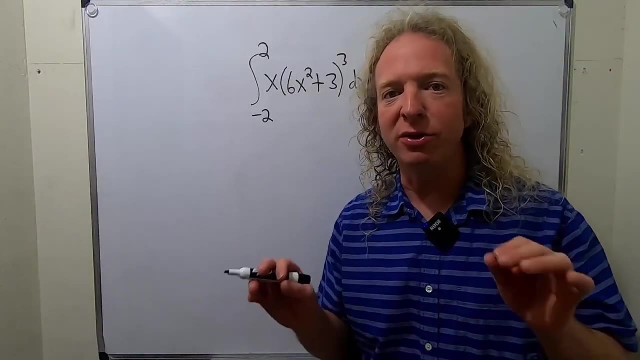 In this video we're going to evaluate this definite integral. So there is a trick to this problem. You can do this immediately and the answer is 0.. So the answer is 0, and you can do it just by looking at it, if you know some stuff. 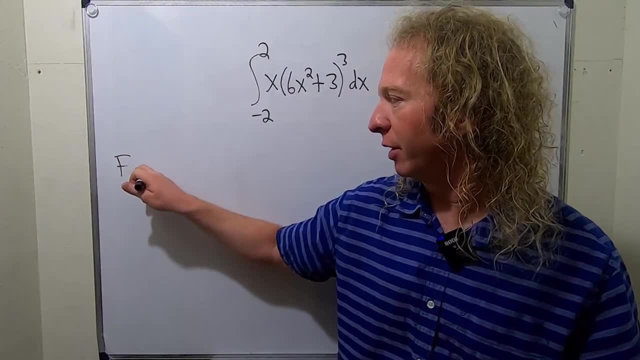 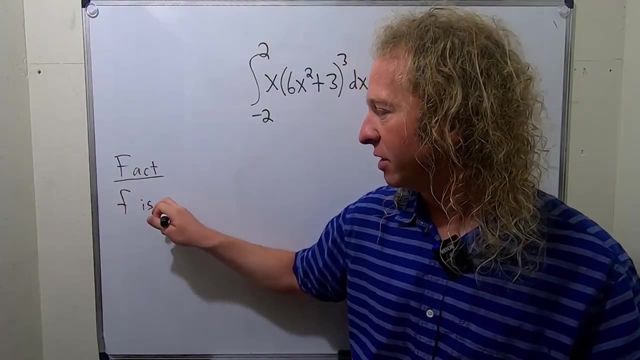 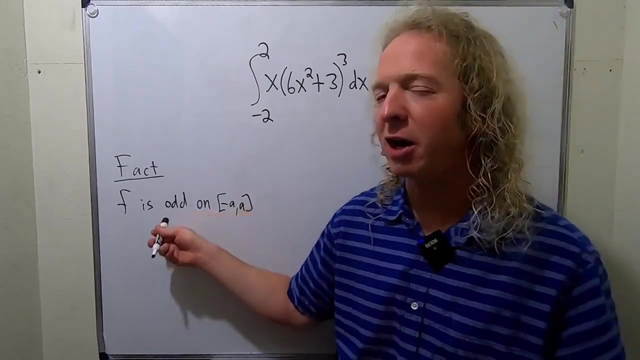 So let me show you This is really really useful in higher level math and in math in general. If you have a function, so if f is odd on, say some interval negative a to a. So we'll talk about what odd means in a second. 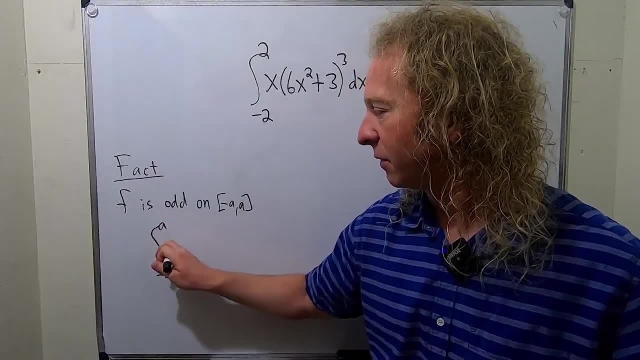 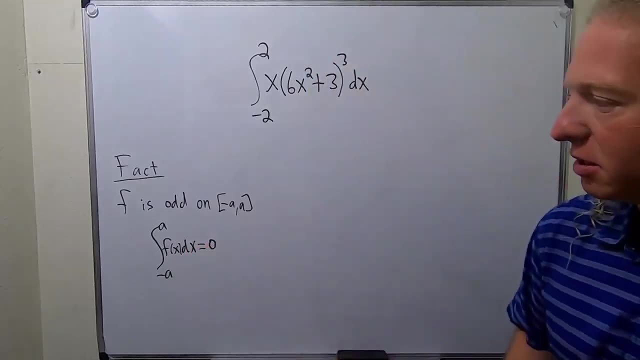 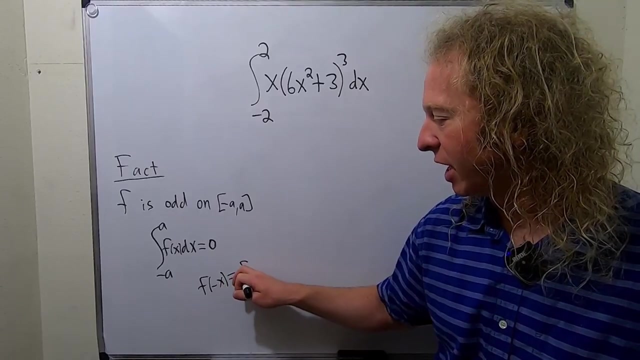 And you integrate f from negative a to a with respect to x, you get 0.. So odd. basically means, when you plug in negative x into the function, the negative comes out and you get negative f of x. So in this example here, this is your f of x. 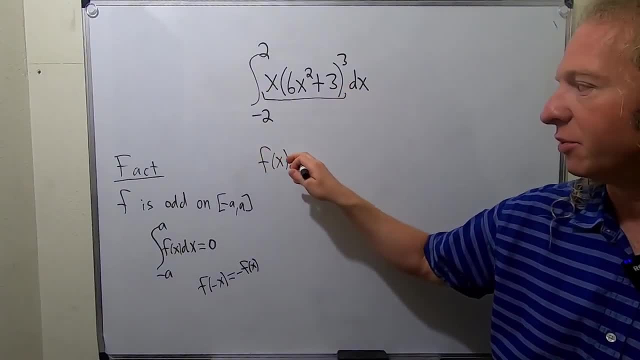 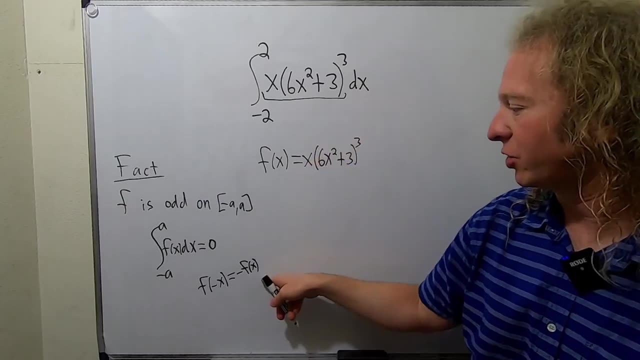 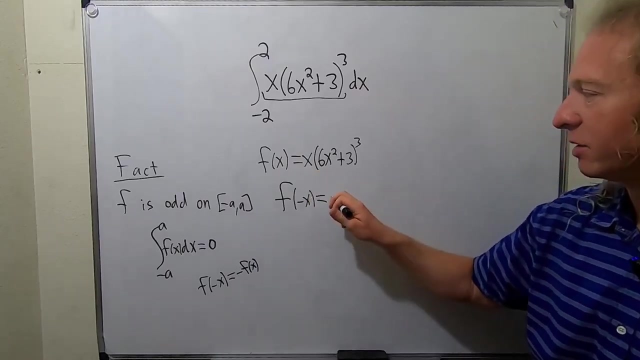 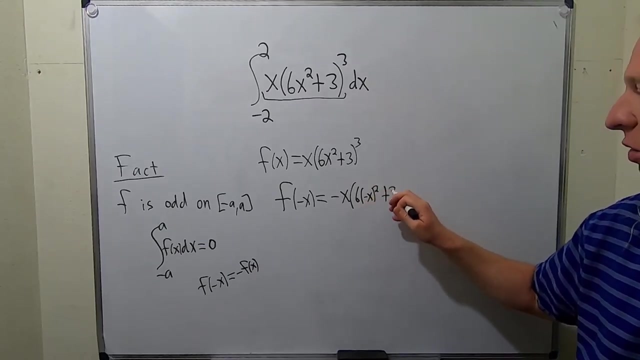 So if you were to write it down, f of x equals x parentheses, 6x squared plus 3 cubed, you could actually check the definition. You could replace the x with the negative x, So your x would become negative x. And then here you would get 6 negative x squared plus 3 quantity cubed. 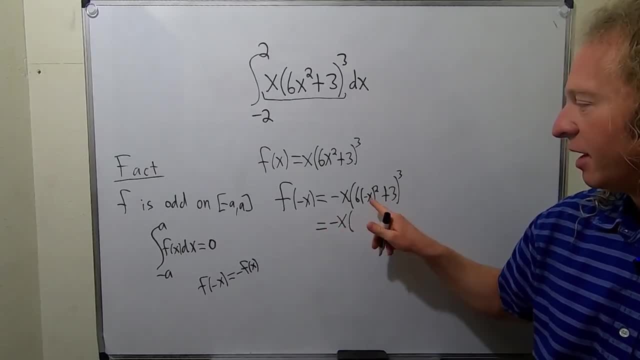 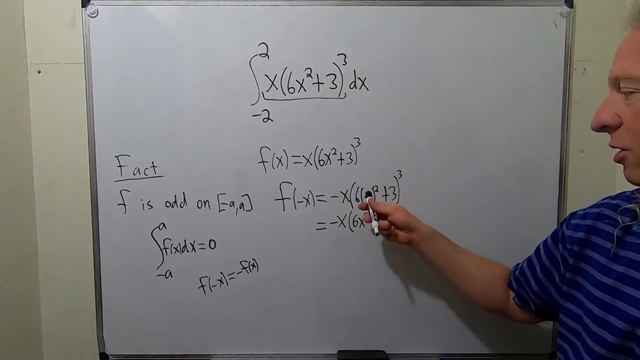 And this is where the magic happens. This is still negative x. This negative, it's being squared right, this negative x. So it's going to become x squared plus 3 cubed, So it goes away because of the 2.. 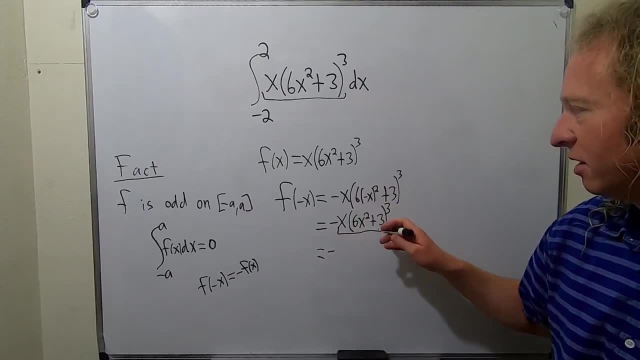 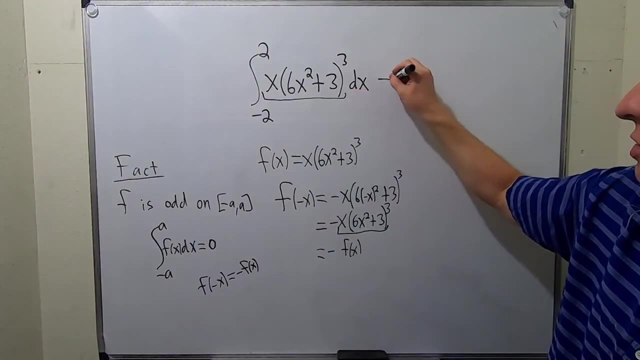 And then this is negative. and what's all of this? This is what we started with, So we proved it. We proved that this function is odd. We're going from negative 2 to 2.. Therefore, the answer is 0.. 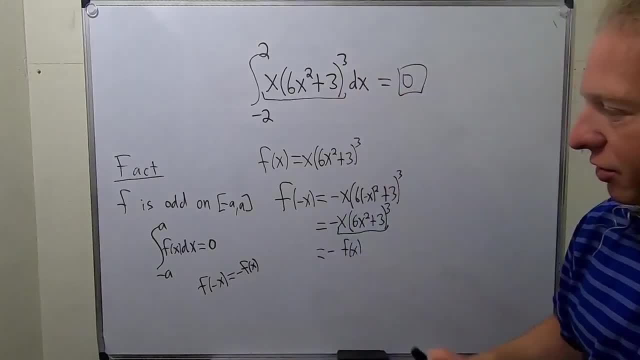 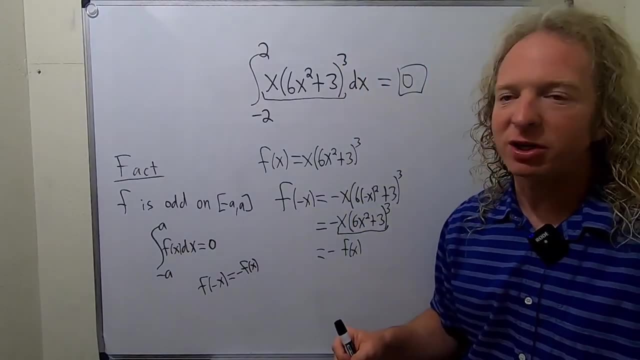 So it's an extremely, extremely powerful technique. Just because it's worth learning some extra stuff. What does it mean for a function to be odd graphically? It basically means it's symmetric about the origin. So, as a quick example, something like this would be odd. 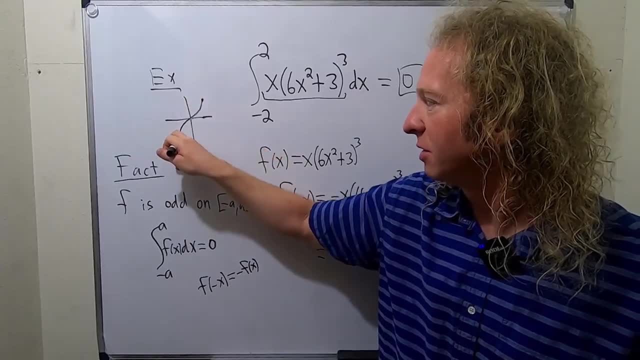 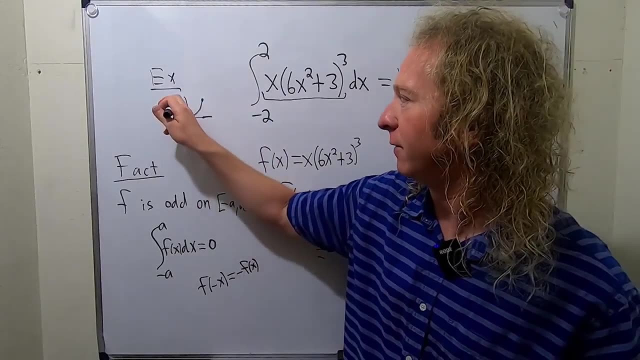 Something like this. Let's just say it stops here and stops here. This is called symmetry. about the origin: This is an example of an odd function. So if you flip it twice, you get the same thing. That's how I think about it. 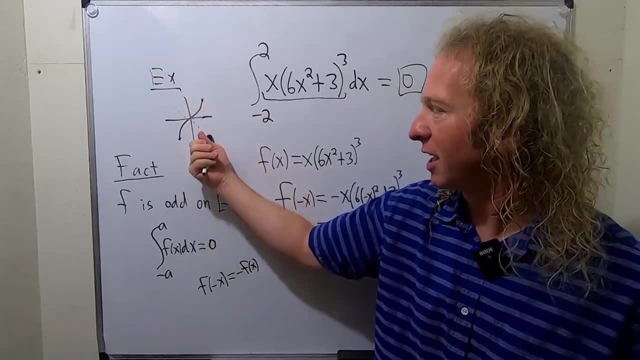 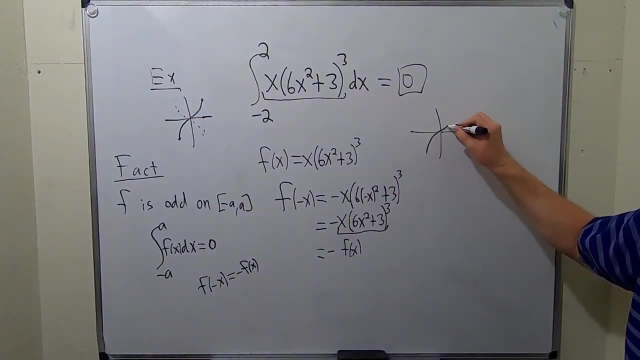 So if you flip it, if you flip it down, you get that. If you flip it down, you get that. Flip it that way, you get that. So flip twice, same thing. So why should this make sense? Well, let's say you were integrating this, right. 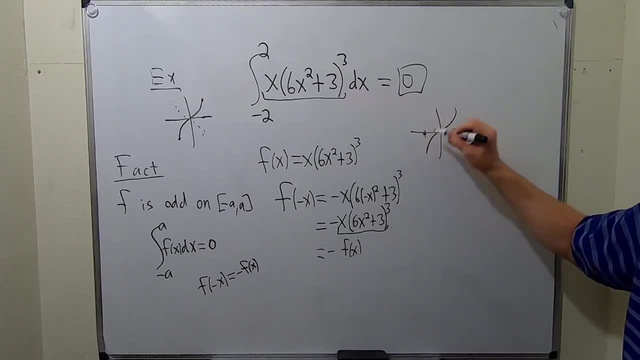 and you were going from here to here. If it's symmetric, this area here is the same as this area here, except this has a negative in front of it. So they cancel each other out when you integrate, and that's why you get zero. 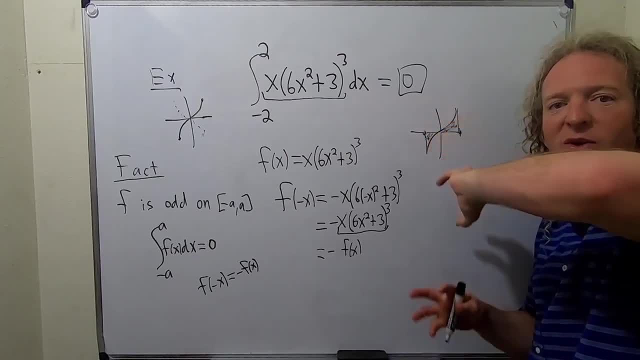 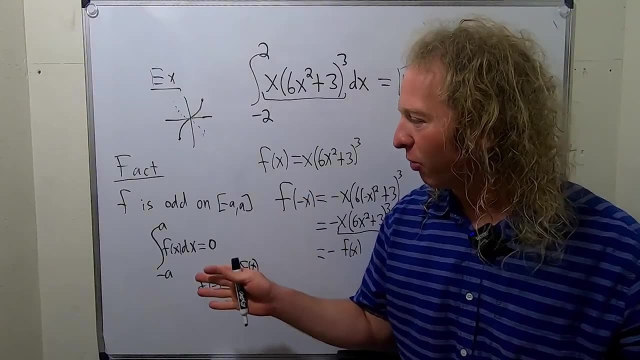 That's the idea, Because if this is positive 2, this is negative 2, and so it cancels when you integrate and that's why you get zero. So, anyways, got sidetracked there a little bit, but really really important fact. 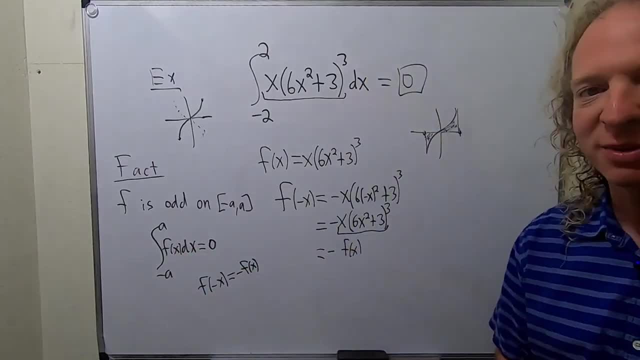 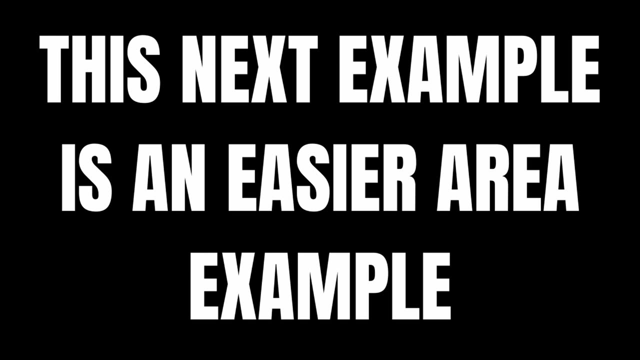 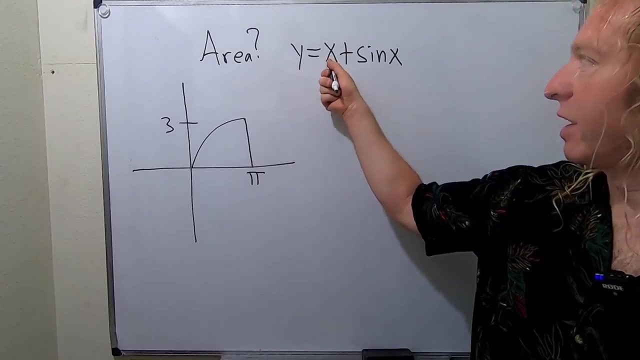 So if f is odd, you get that. I hope this video has been helpful. Take care: In this video we're going to find the area given in this picture. So this is the graph of x plus sine x and we're restricting the domain from 0 to pi. 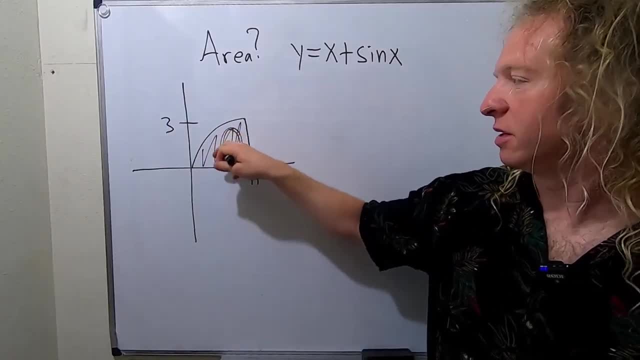 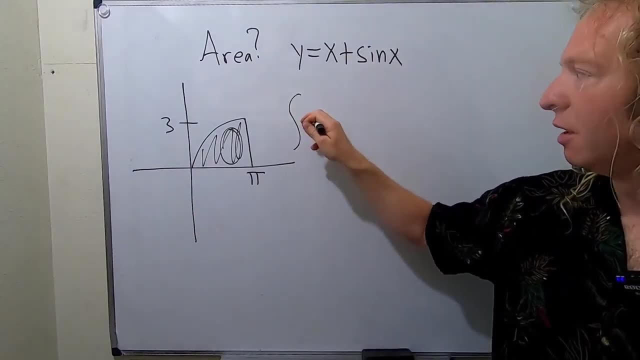 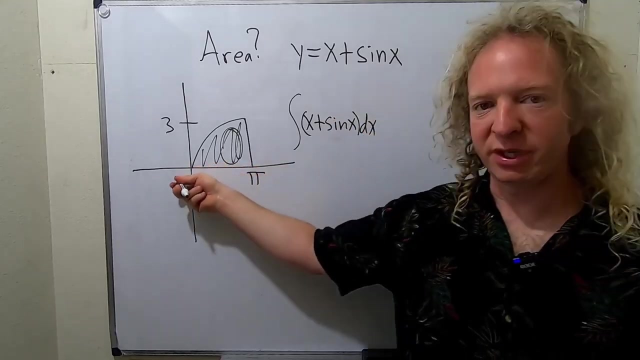 So we're looking for this area here. So this area here is given by the definite integral from 0 to pi. So basically all we have to do is integrate this, so x plus sine x, and then we have dx and we have to go from 0 to pi. 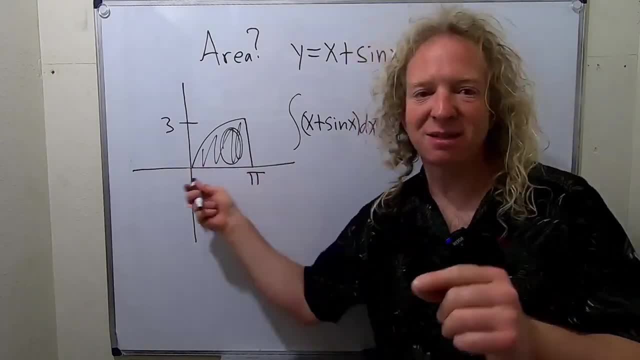 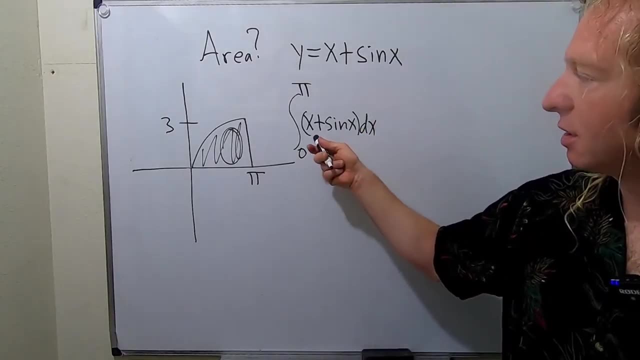 We're integrating with respect to x, so we have to use x's for our limits of integration, Alright. so all we have to do now is integrate this. So to integrate x, we use the power rule. There's a 1 here. 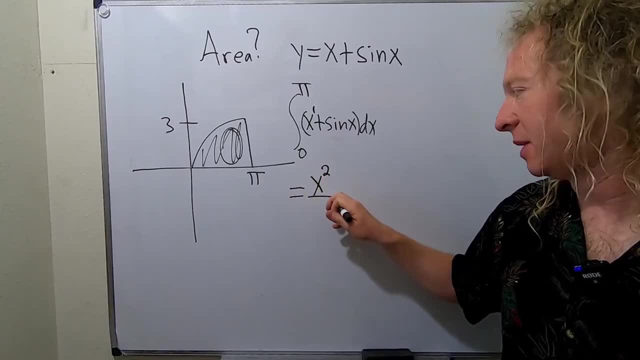 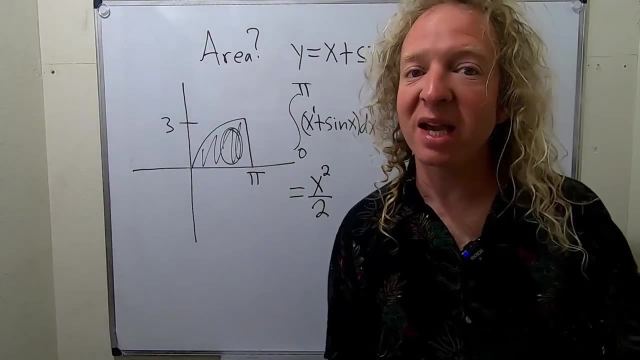 so this is simply x squared, because you add 1, and then divide by 2.. So 1 plus 1 is 2, then you divide by that To integrate sine. it's going to be negative cosine. So the reason I know that is because if you take the derivative of cosine, 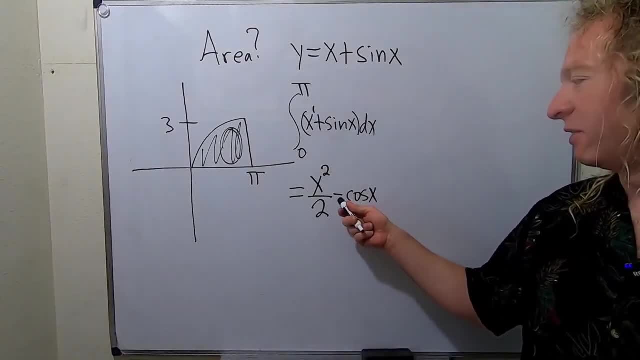 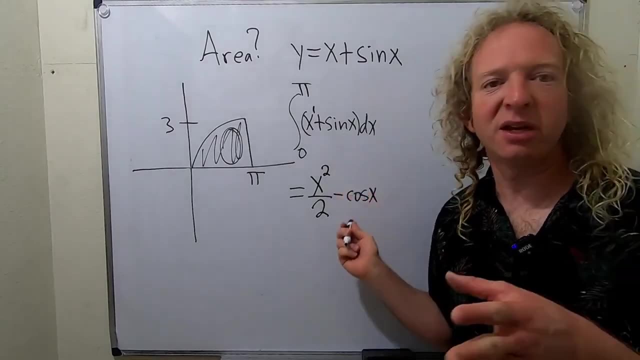 you get negative sine, But there's already a negative here, so it'll make it positive. Okay, so the derivative of this is negative sine, but negative and negative is positive. So when you integrate sine, you do get a negative cosine. 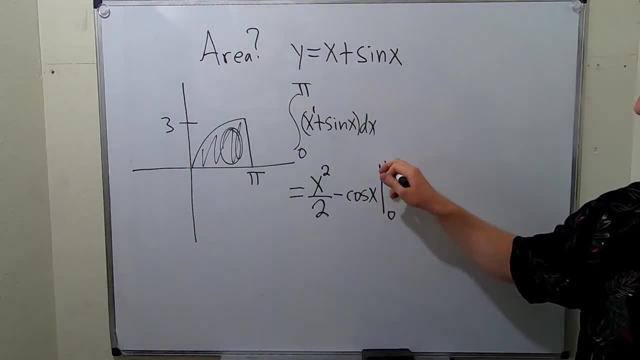 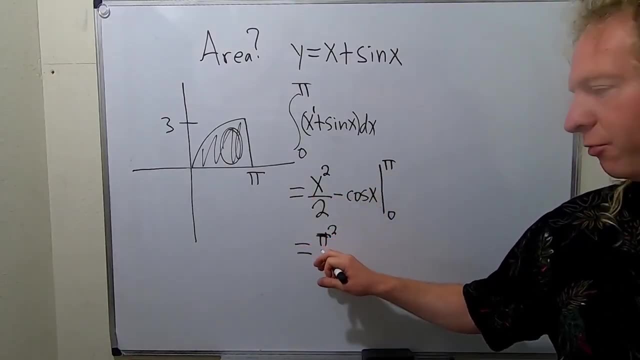 And I'll just put a line here: and we're going from 0 to pi. Alright, so first we plug in the pi. So this is equal to pi squared- whoops, whoops, pi squared over 2, minus, and then plug in the pi. 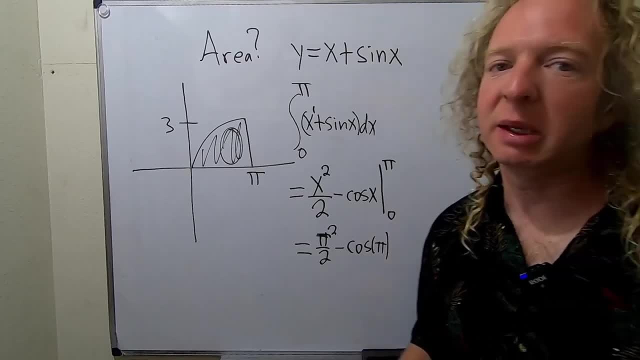 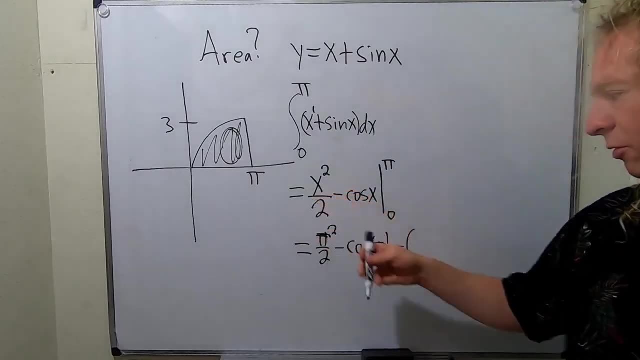 cosine of pi. So you always plug in the pi first, And then minus, and now you plug in the 0. So- parentheses- plugging in 0, we get 0 squared over 2.. I'll even write it, Why not? 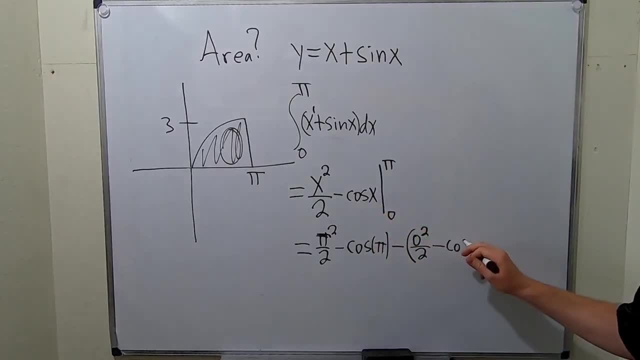 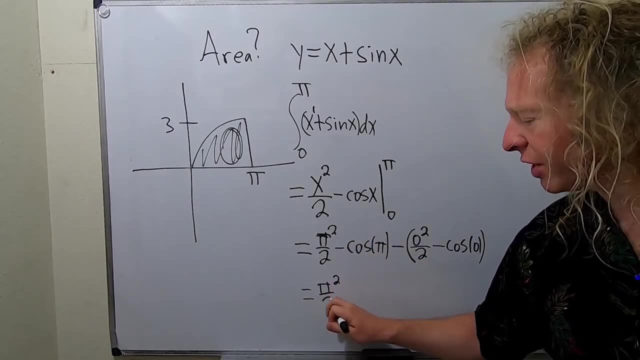 Minus cosine of 0. So this is cosine of 0.. So boom, there we are. Alright, so we have pi squared over 2.. Pi squared over 2. Cosine of pi is negative 1. So this is oh minus. 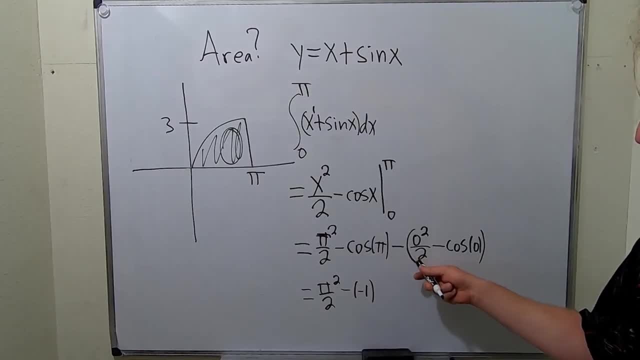 I'll write it minus negative 1.. This is gone. Okay, this is 0.. So this is minus. this is negative. this is 1.. Cosine of 0 is 1.. So this is minus that, because this becomes 1.. 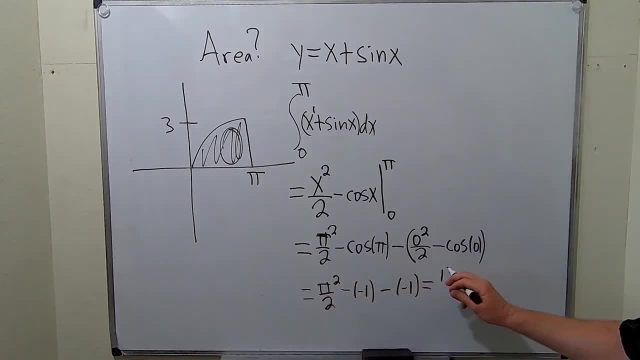 So this is equal to: let's see pi squared over 2, and then 1 plus 1, plus 1 plus 1, because these will all become pluses. So we end up with pi squared over 2, plus 2.. 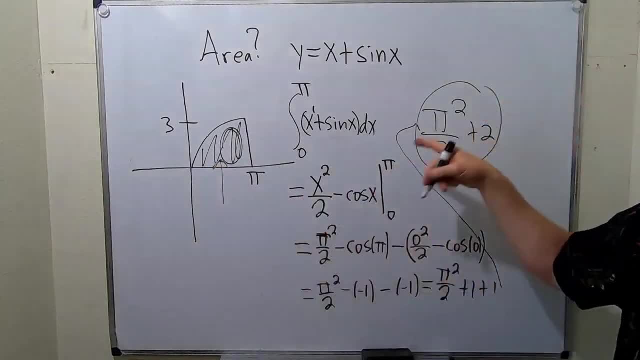 So this is, this is the area. So this area here, this area is given by pi squared over 2, plus 2.. Kind of cool, Kind of a cool answer. right, We got some, some pi's in the mix. 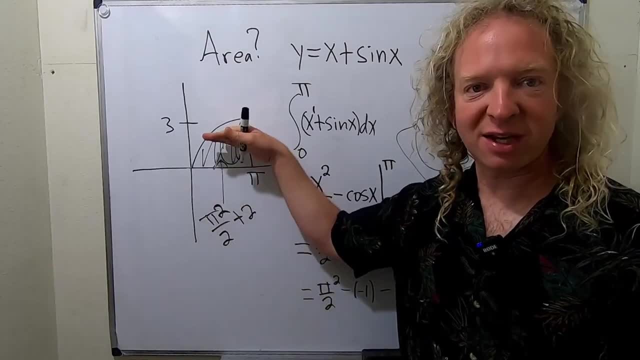 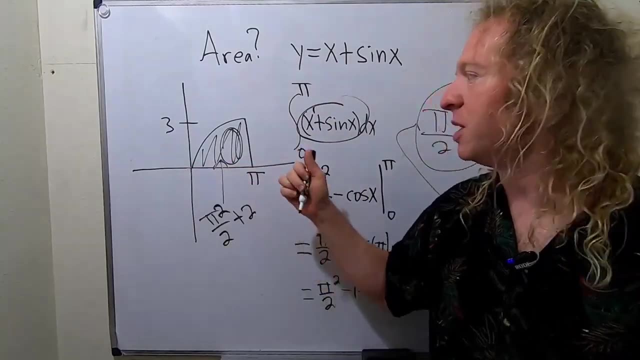 So whenever you have to find an area of a function that's above the x-axis, all you do is you integrate from left to right. So you take your function and you just integrate from here to here. The reason is, if you remember, 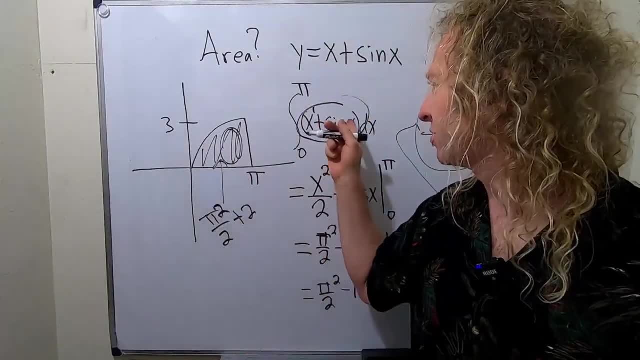 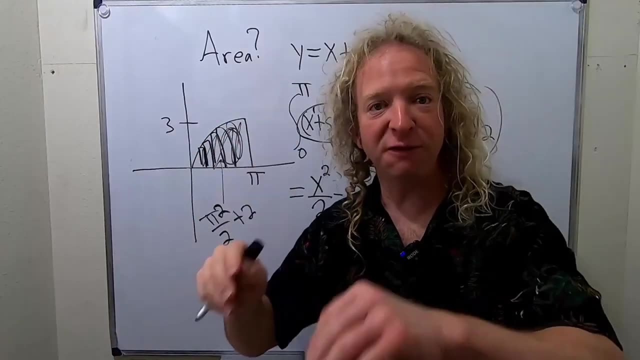 in the construction of the Riemann integral. what you do, this is actually equal to a limit. you approximate this with, with rectangles, and then you take the limit of infinite, of the sum of infinitely many rectangles, and that gives you the area. 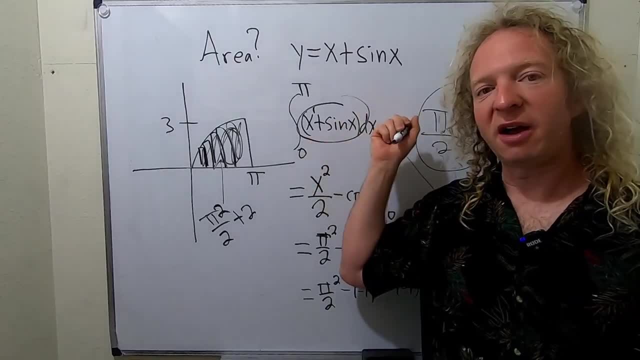 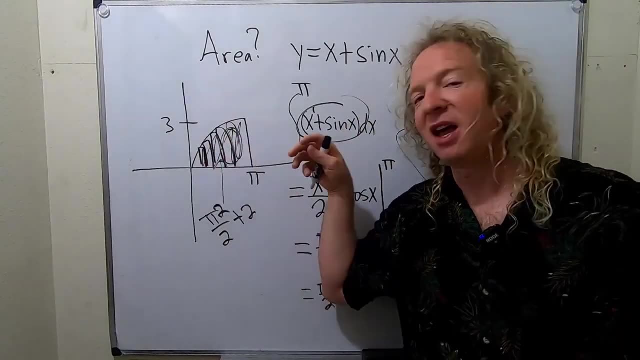 That's what this is. This is actually equal to the limit of the sum of finally many rectangles. So this is actually equal to a sum of infinitely many rectangles, and that covers this area and that gives you the area. So I hope this video has been helpful. 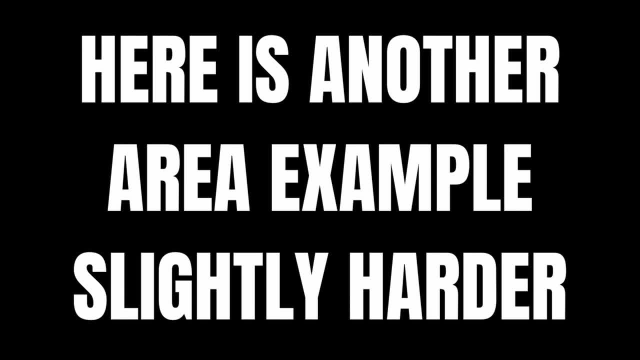 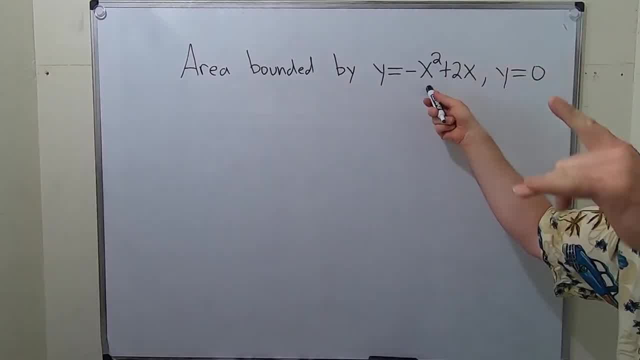 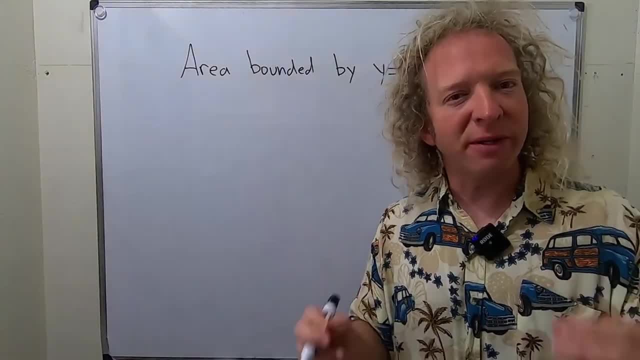 Take care In this problem. we're going to find the area bounded by the graph of this parabola and the line y equals 0.. So to do that, the first thing we have to do is draw a picture so we can figure out the limits of integration. 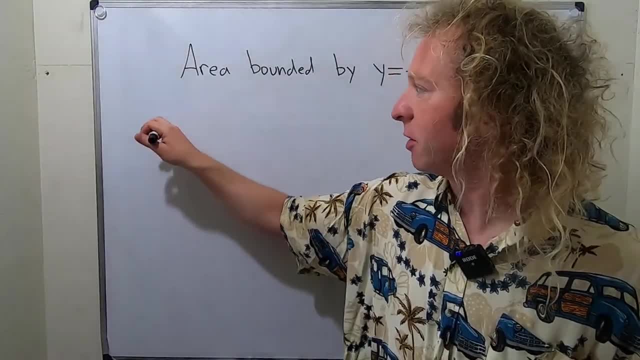 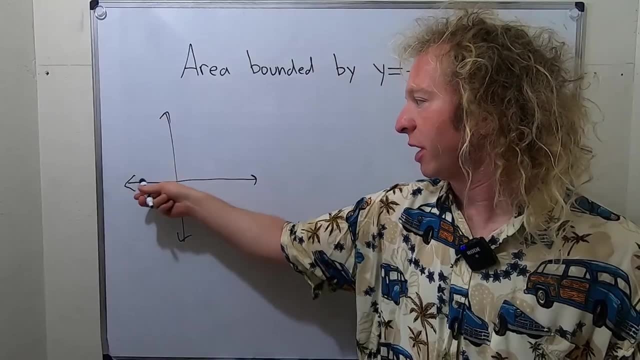 for the integral that gives us this area. So let's do it, Let's draw the picture. So there's the y-axis, there's the x-axis, So the line y equals 0 is just like a horizontal line right here on the x-axis. 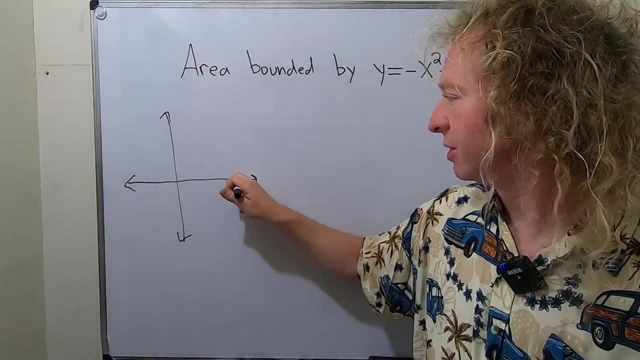 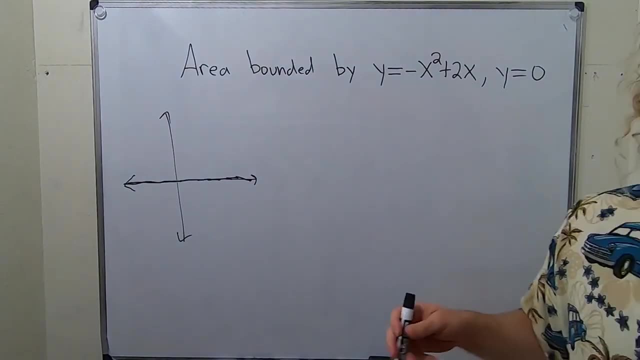 So that part's pretty easy. So I'll just do this to indicate that that is: y equals 0.. Then we have to figure out how to graph this parabola. So what I'm thinking is, maybe we can set it equal to 0. 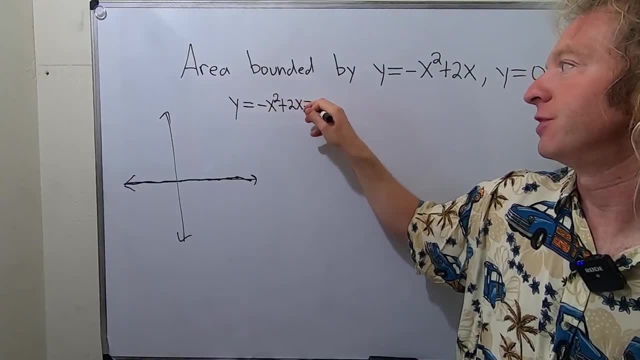 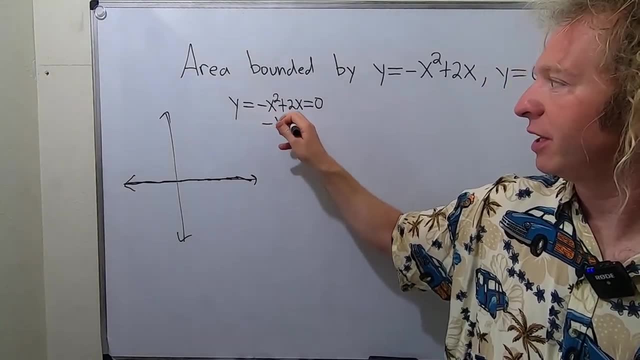 to find the x-intercepts. So it's a good first step. Alright, so then we have to factor. I guess we can factor out a negative x. So pull out a negative x. That'll leave you with x minus 2.. Right, because negative x times x. 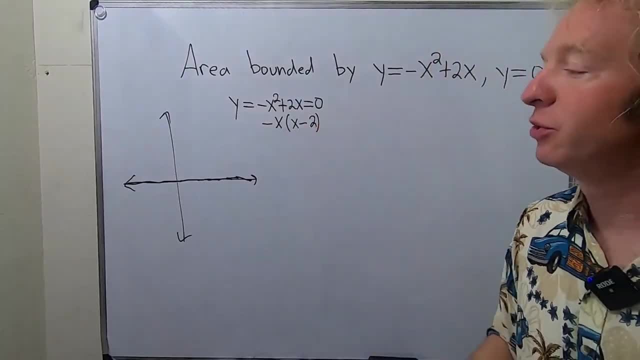 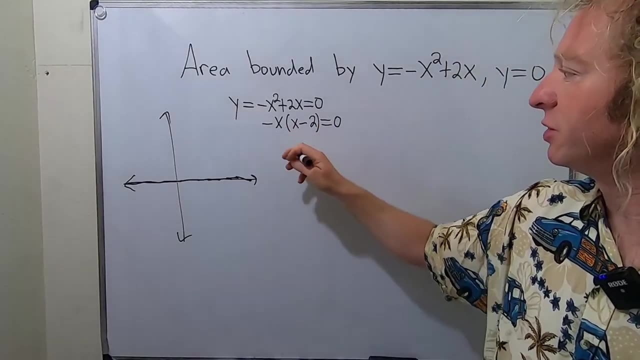 is negative x. squared Negative x times minus 2 is positive 2x, So this is equal to 0.. So it looks like we get two possible x-intercepts. x equals 0 comes from here, And this one's going to give us. 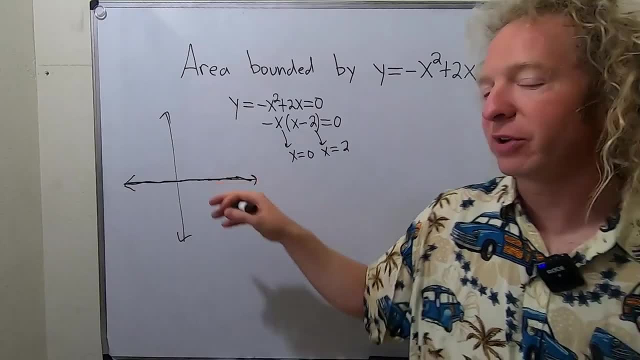 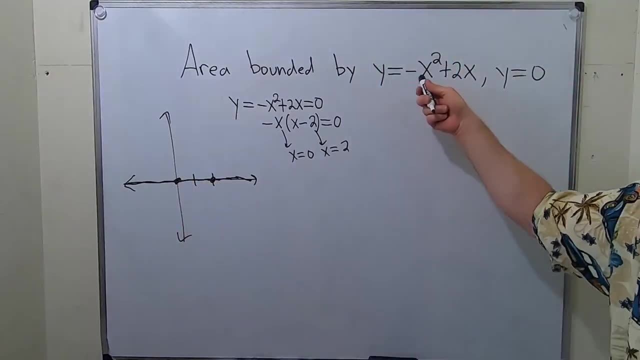 x equals 2.. So I'm going to come over here to the graph and just plot the 0.. And then over here plot the 2.. Alright, so this has a negative number here. So that means it opens down. So it's a parabola opening down. 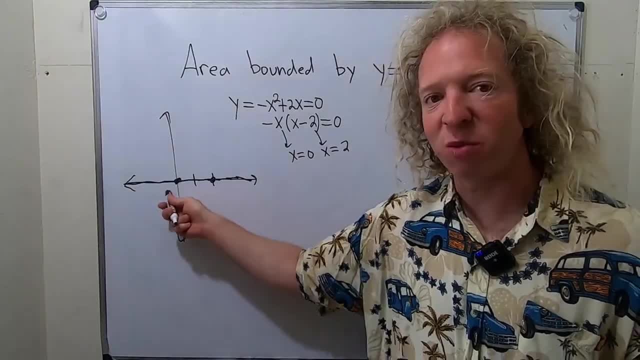 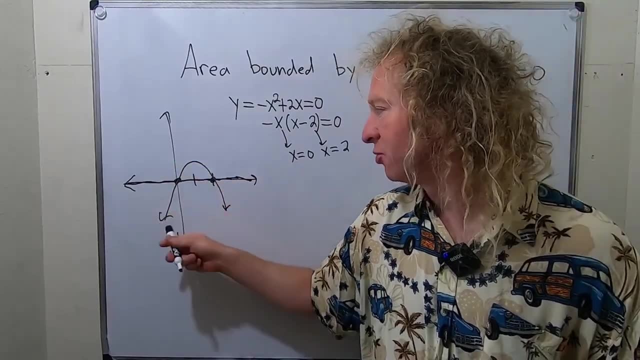 So it cannot look like this, because it has to cross at these points. That means it must be up here somewhere, So it has to do something like that. There's no way for me to draw it down here, because it would have to cross these x-intercepts. 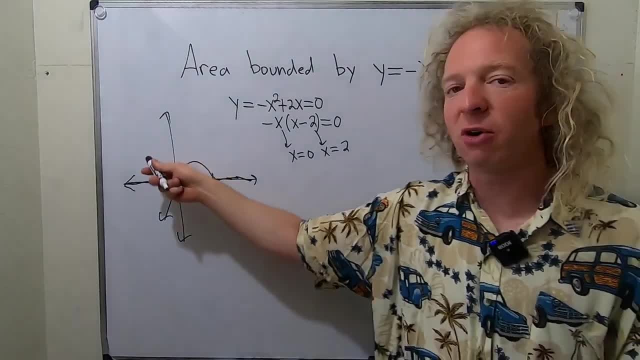 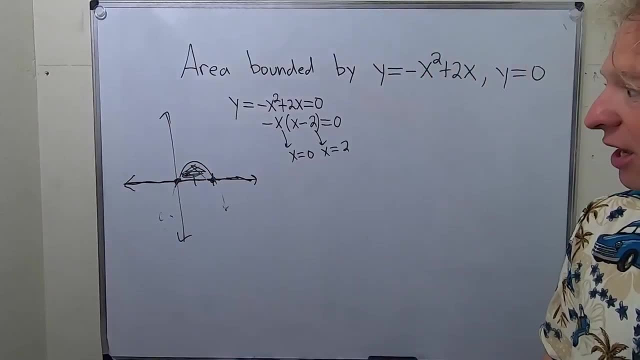 So then you know it opens down because it's negative. If this was positive, you know it would be opening up, Okay, so basically we have to find this area here And we're done So. to do that, all we have to do is integrate. 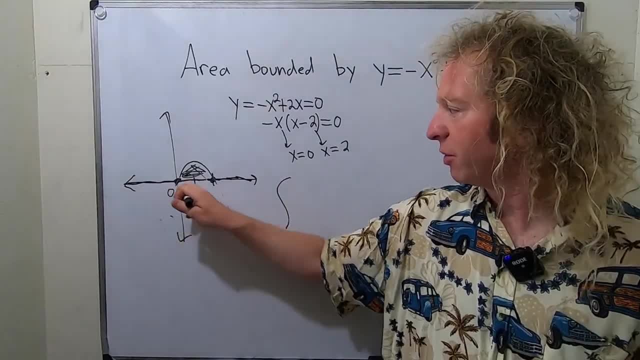 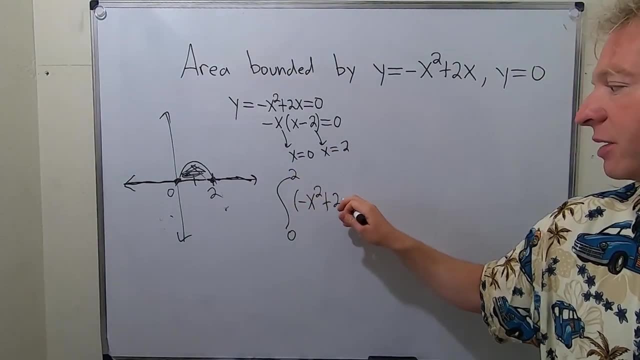 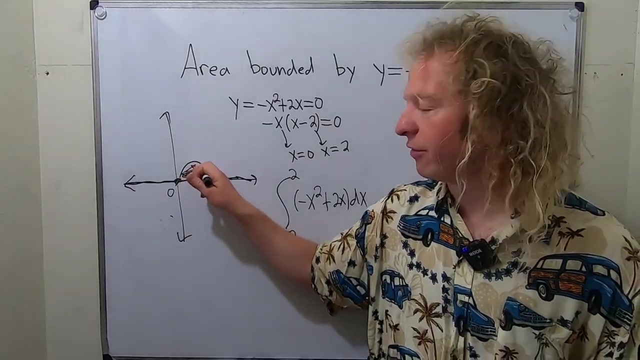 This area is given by the definite integral from 0 to 2 of this graph, So negative x squared plus 2x dx. Okay, so all we have to do is work this out and this will give us the area of this shaded region. 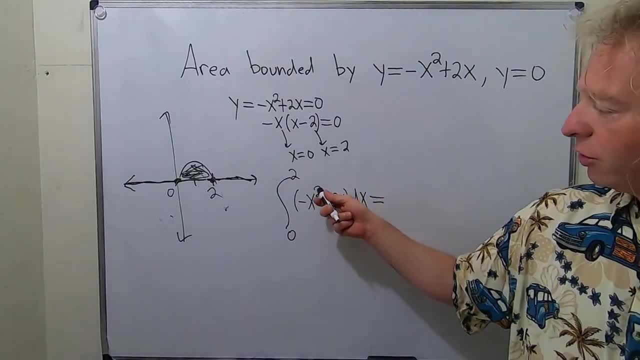 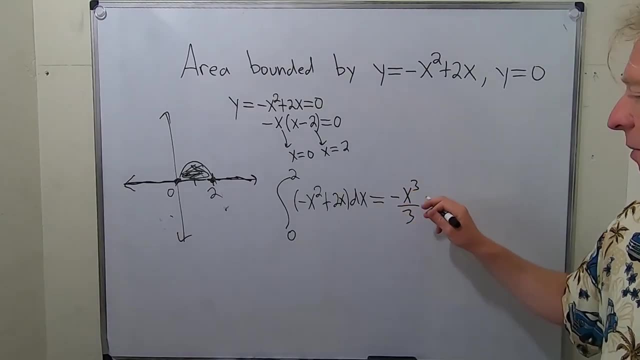 So to integrate this we'll use the power rule. So you add 1,, so you'll get 3.. Then you divide by that number, So this is negative x cubed over 3.. And then plus Here there's a 1,. 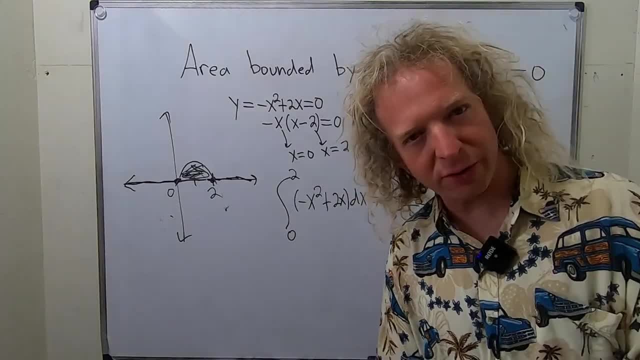 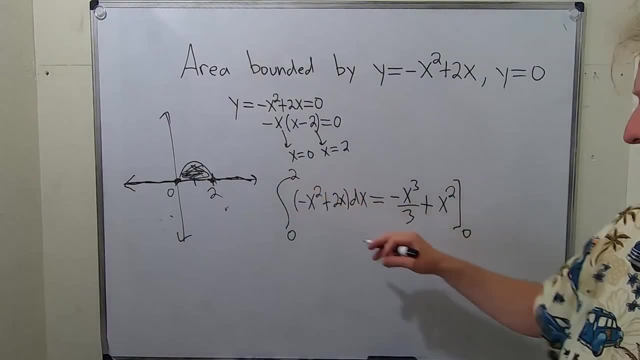 so you add 1 and divide by that, So it'd be 2x squared over 2.. That's just going to give you x squared And we're going from 0 to 2.. So everything looks good so far. All right, good stuff. 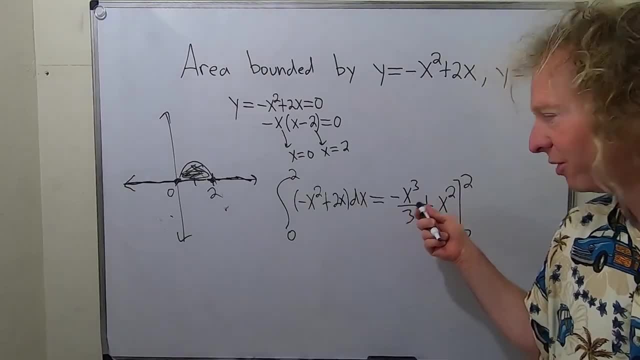 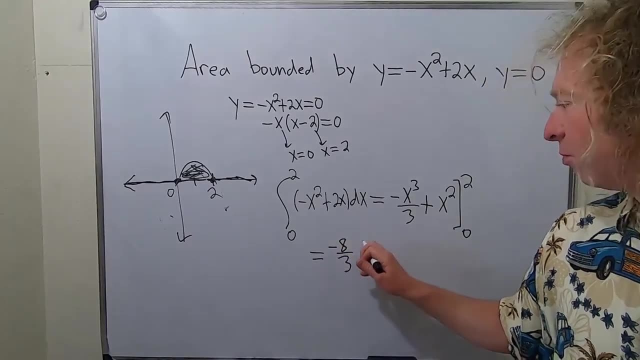 You plug in the 2 first subtract, then plug in the 0. So plugging in 2 here, that's going to give us 2 cubed, which is 8.. So this is negative 8 thirds plus, and then 2 squared is 4.. 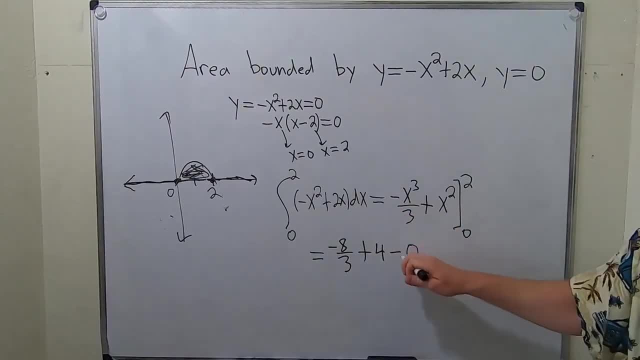 Minus and then when you plug in 0, it's all 0, so I'm just going to do that. So now we have to add these up. This is negative 8 thirds. To add the 4 and the negative 8 thirds. 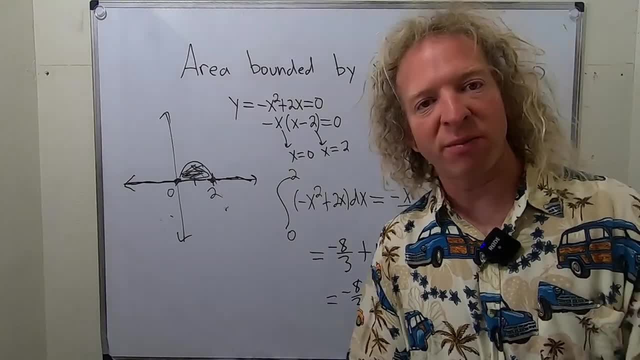 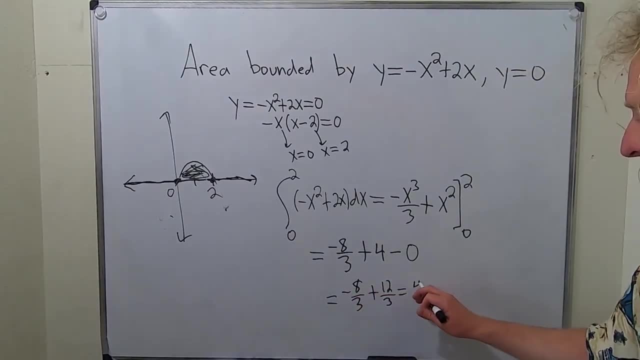 what you can do is think of 4 as a number over 3. So 12 over 3 is equal to 4. So 12 over 3.. Adding these up, you just get 4 thirds, and that is the area bounded by the graphs. 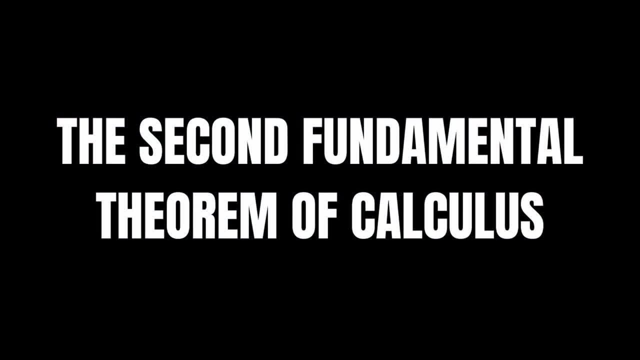 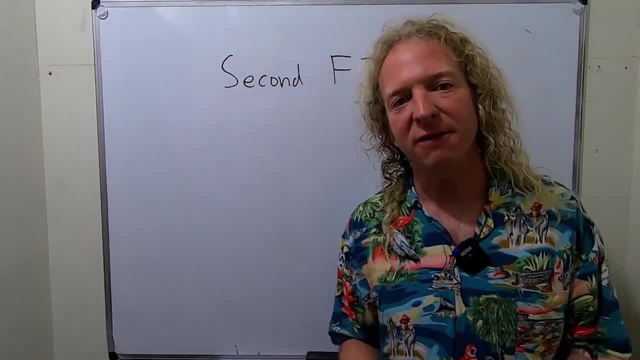 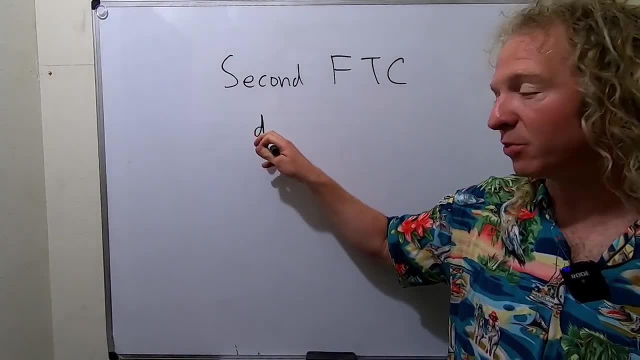 I hope this video has been helpful. Take care: In this video I want to talk about the second fundamental theorem of calculus. It basically says, if you have a continuous function, that there is a formula you can use, and it's actually really easy. 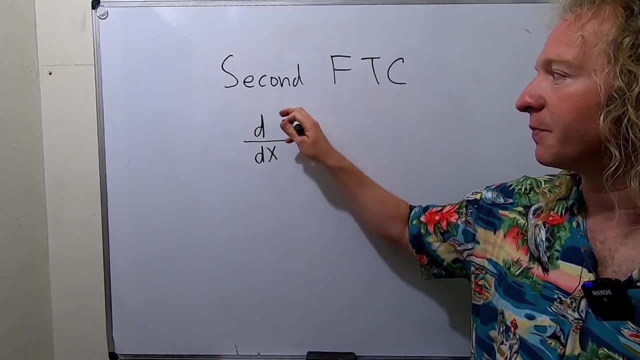 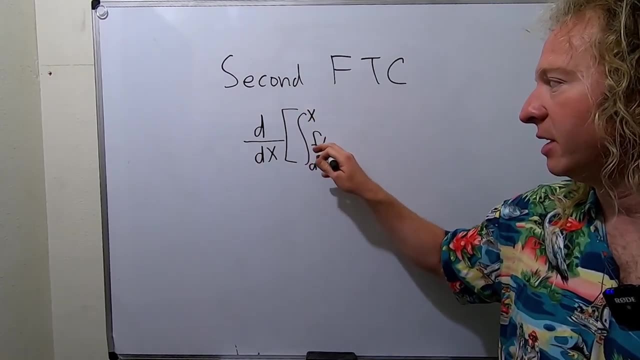 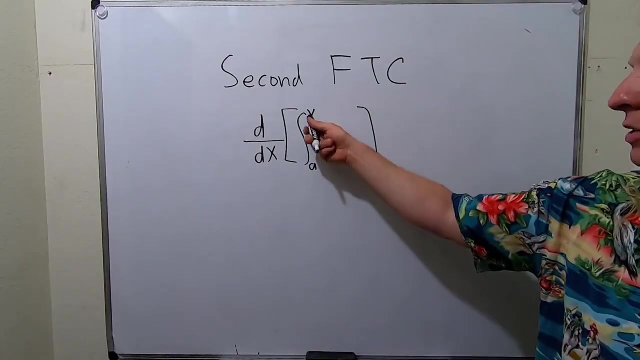 So if you take the derivative with respect to x of the definite integral from a to x of f, of t, dt, all you have to do, okay, is you just put the x where the t is. So this is just f of x. 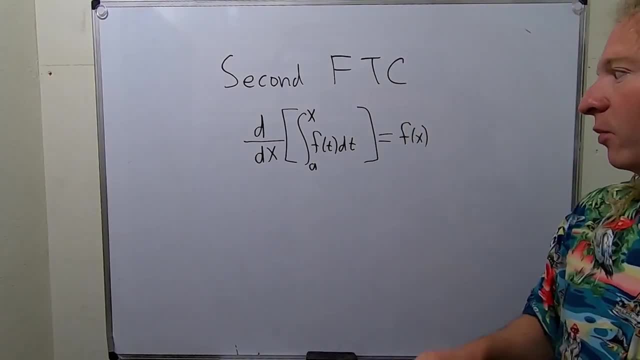 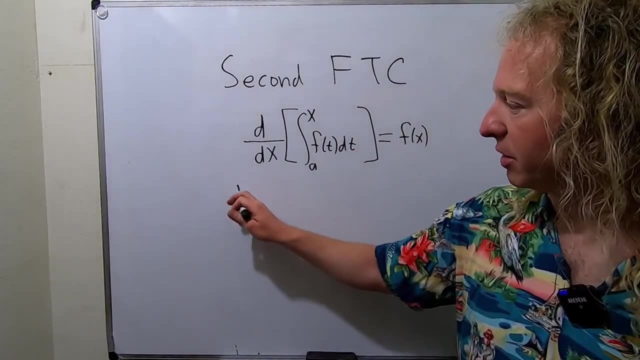 That's all you do. So let's do a simple example right away, and then maybe we'll go through the proof Again. the condition here is that f is continuous. Let's do a simple example so you see how simple this actually is. 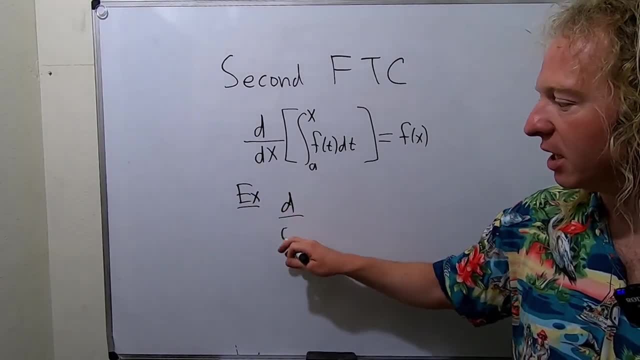 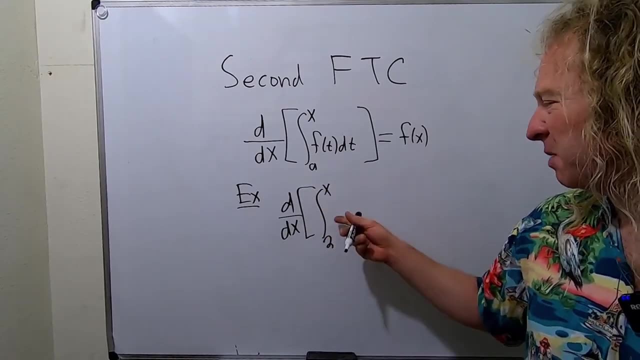 It looks really hard, but it's actually really easy. So if you have ddx of, let's say the integral, let's make the a a 2. Let's make this an x. Let's put something here. Ooh, let's put something weird here. 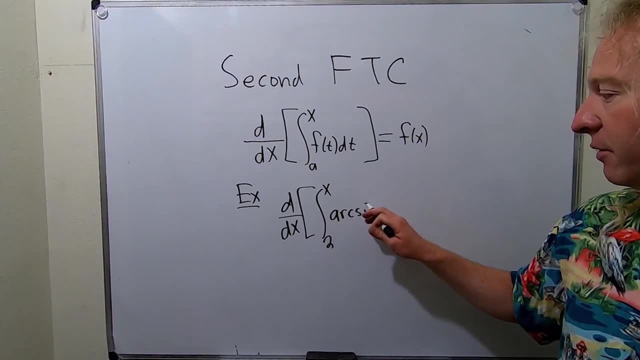 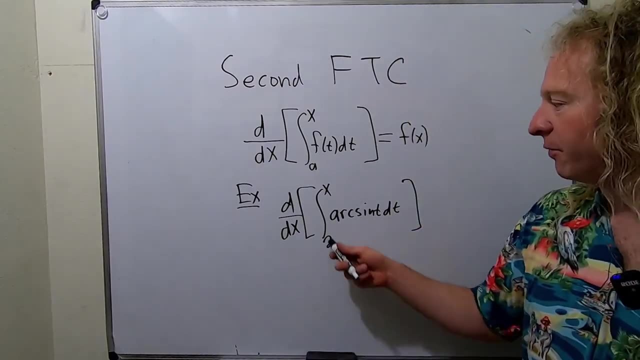 something that you might not be familiar with: Arc sine of t, dt. So, according to the formula, all you have to do when you take this derivative is just take the x and you put it where the t is, So it's arc sine. 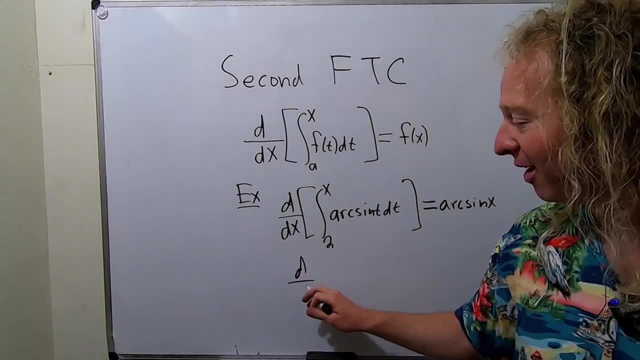 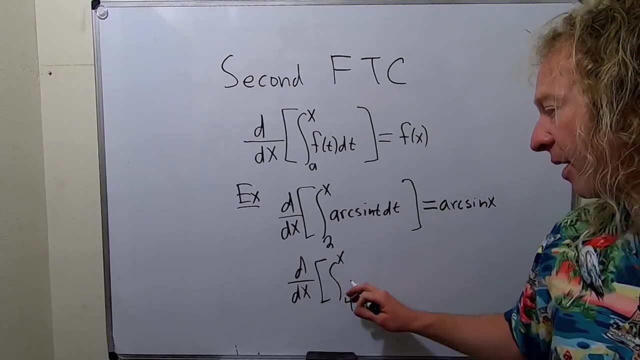 of x. That's it. So let's do another one, one more. so you see how simple it is: ddx. let's do 4.. Let's put an x here and let's put e to the t squared dt. 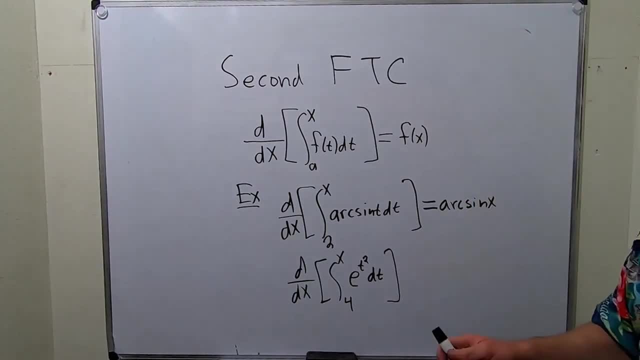 That's a fun one. So same thing. All you do is you take the x and you put it where the t is. So this will be e to the x squared. So that's how you use the second fundamental theorem of calculus. So whenever you have a number here, 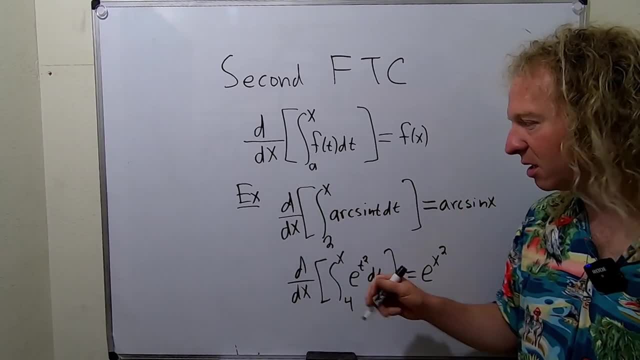 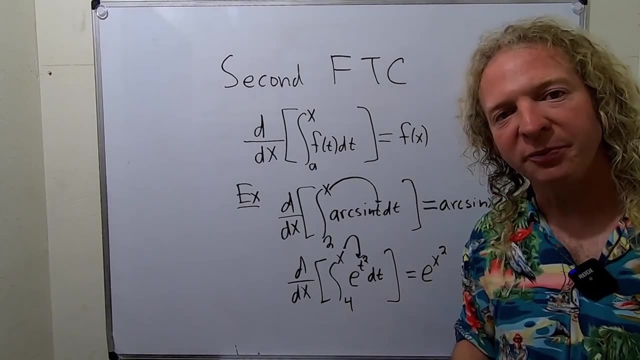 and an x and you take the derivative and it's set up just like this: you just take the x, put it where the t is, Take the x, put it where the t is. Let's do a really, really, really quick proof sketch. 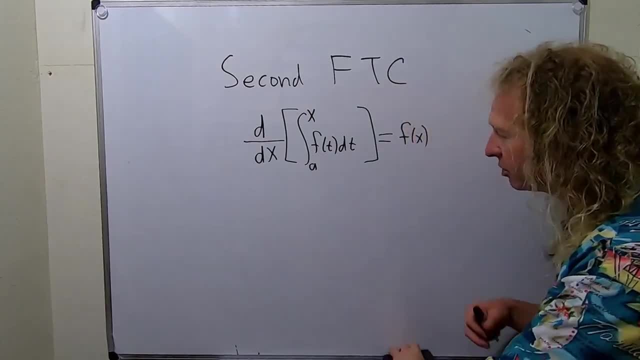 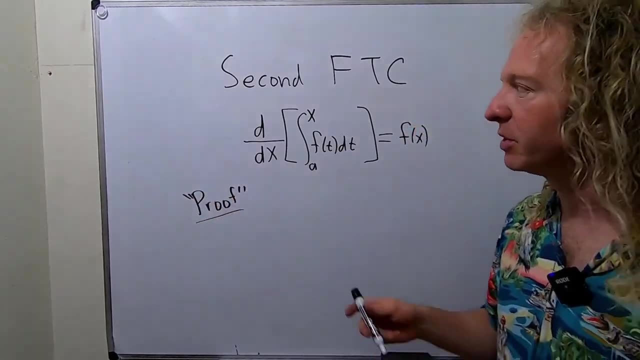 just so you see why this is true. So this is like a proof sketch. I can be really formal here, So I'll just call it a proof and put it in quotes, just for understanding purposes. So our function's continuous. So what we can do here. 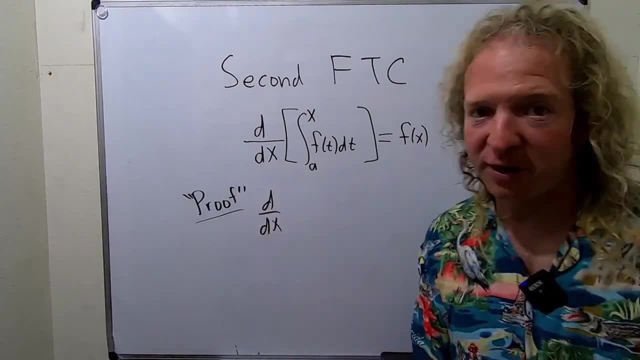 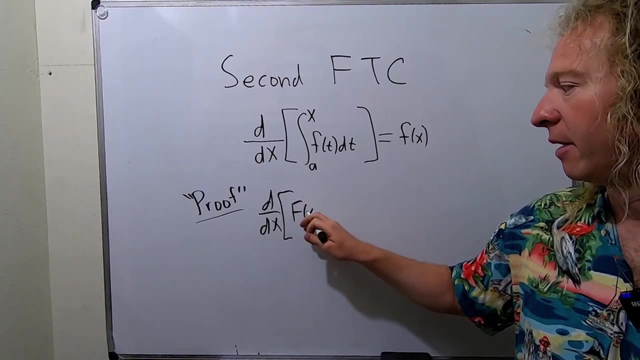 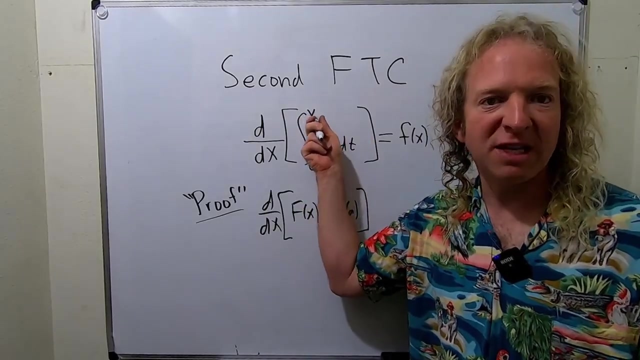 is, we can use what's called the first fundamental theorem of calculus. So this says that this is going to be equal to big F of x minus big F of a. If you remember this from before, it was big F of b minus big F of a. 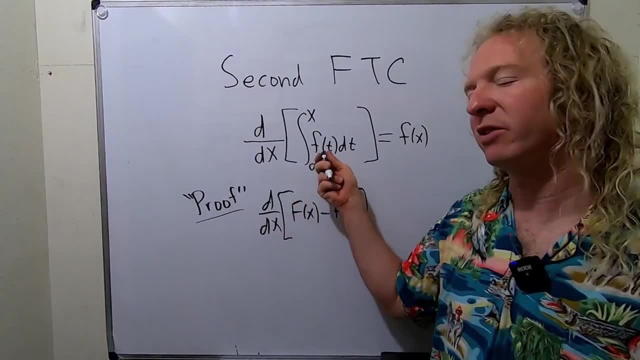 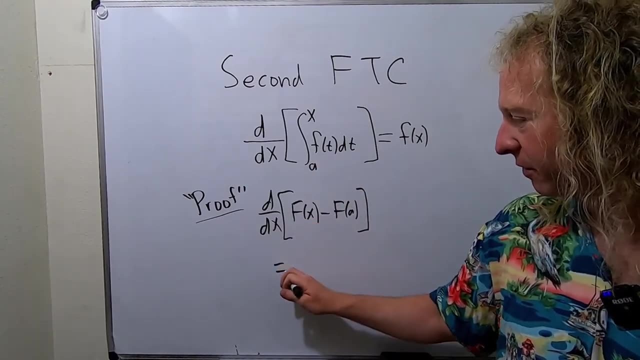 except this time it's x. Well, big F is an anti-derivative for little f. That means if you take the derivative of big F, you get little f. In fact, when you take the derivative of big F, you get little f. 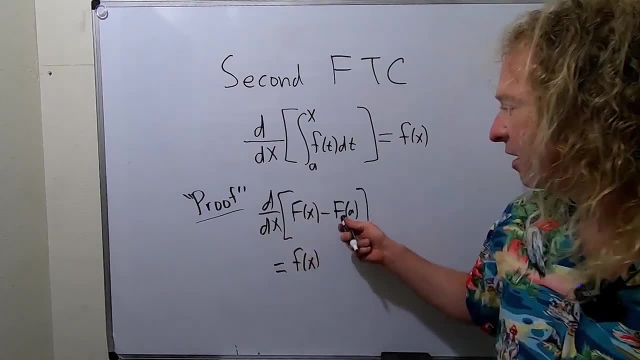 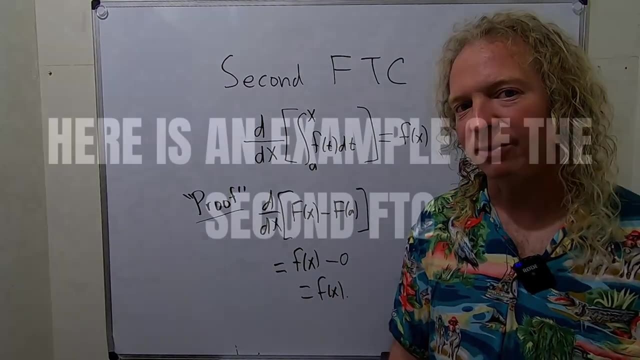 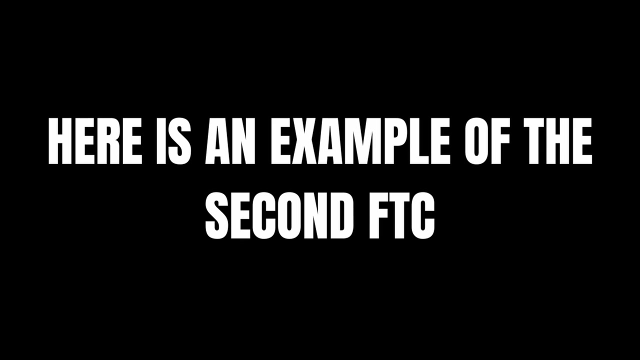 That's the definition, right? The derivative of big F is little f. This is a number, so it's just 0, so we just get F of x. So I hope this video has been helpful. Take care In this video. 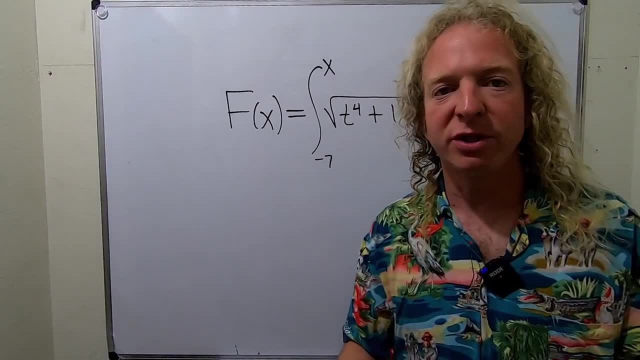 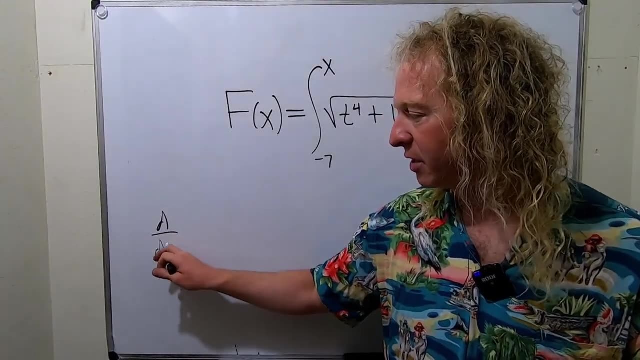 we're going to find the derivative of this. We're simply going to use something called the second fundamental theorem of calculus. So the formula for the second fundamental theorem of calculus says: if you have the derivative, with respect to x, of the definite integral from a to x, 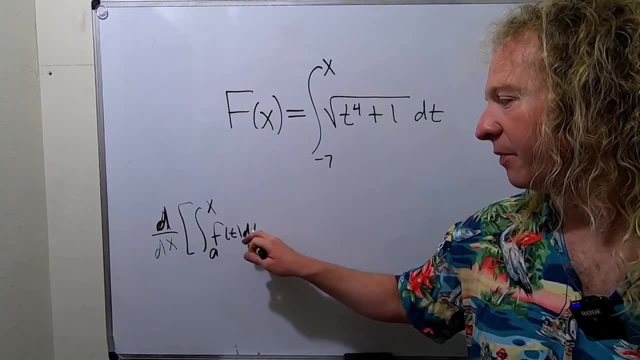 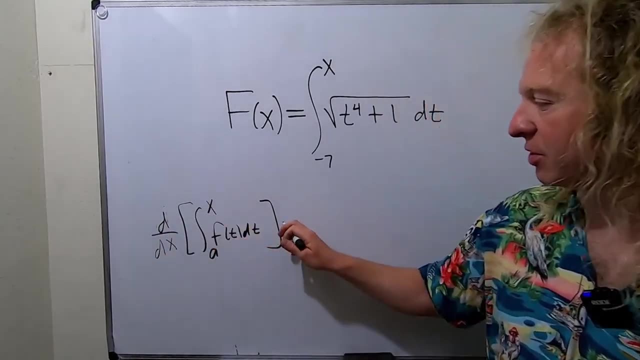 of F of t dt. so if you have this set up and you take the derivative, that's a, d with respect to x, all you do is you put the x here. So this is equal to F of x. So in this case here, 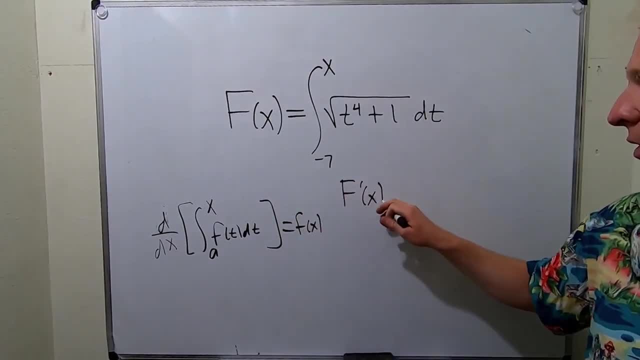 when we take the derivative. so all you do is you put the x where the t is. So this will be equal to the square root of x, to the fourth plus 1.. And that's it. That's it. That is the final answer. 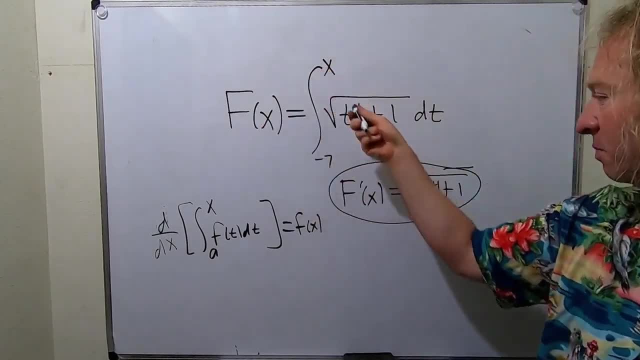 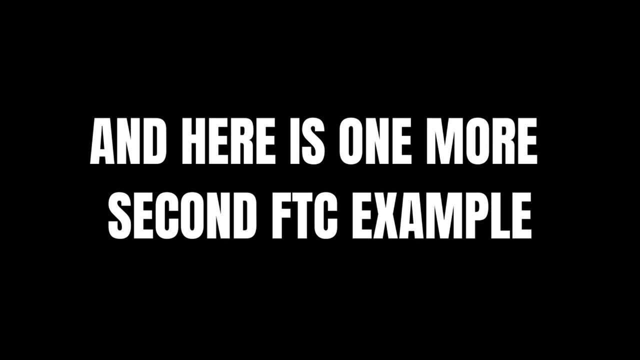 So whenever you have an x in a number here and you take the derivative, just put the x where the t is and that's it. Take care, In this video we're going to find the derivative of this We're going to use. 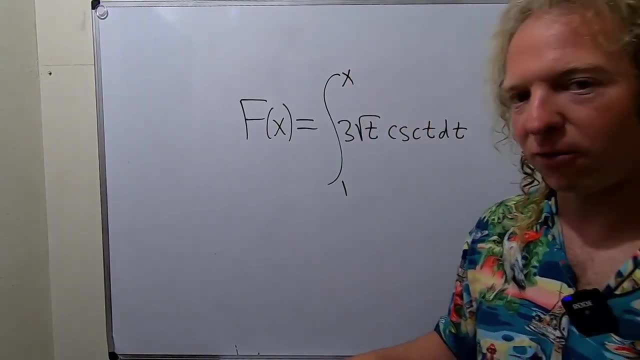 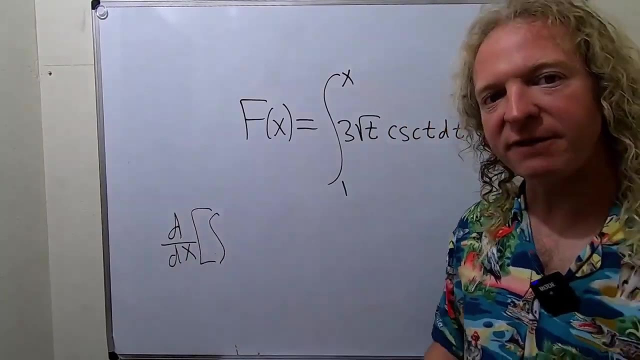 something called the second fundamental theorem of calculus. The formula for the second fundamental theorem of calculus says: if you have the derivative, with respect to x, of the definite integral from, let's say a number, a to x, of F, of t with respect to t, 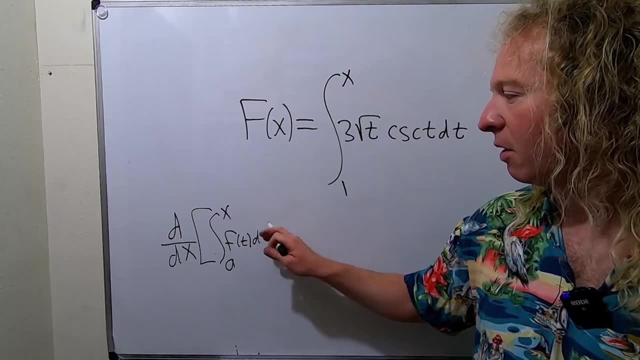 all you do is you take the x and you put it where the t is, So it's just F of x. That's all you do. So in this case, here, when we take the derivative, so big F, prime of x, all we do is: 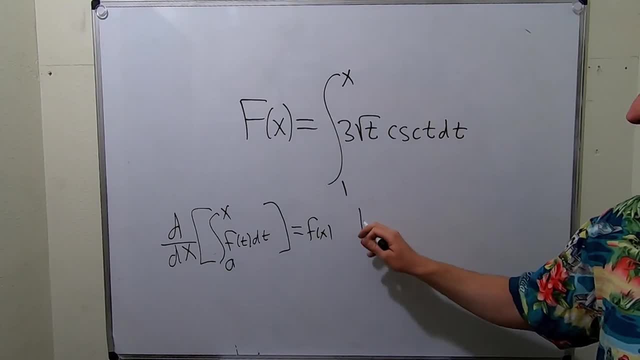 we take the x and we put it where the t is. So it will be 3 square root of x plus secant x, And that is it, Thank you. See you next time. Bye, Bye, Bye, Bye, Bye. 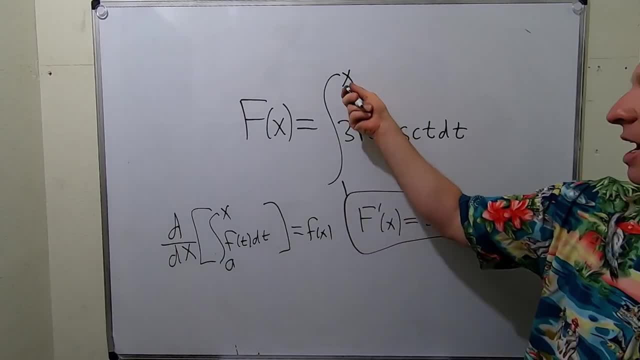 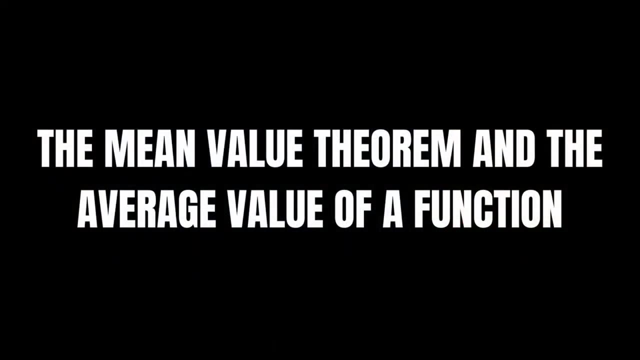 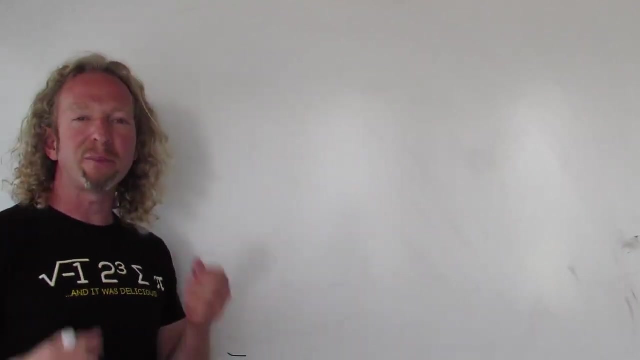 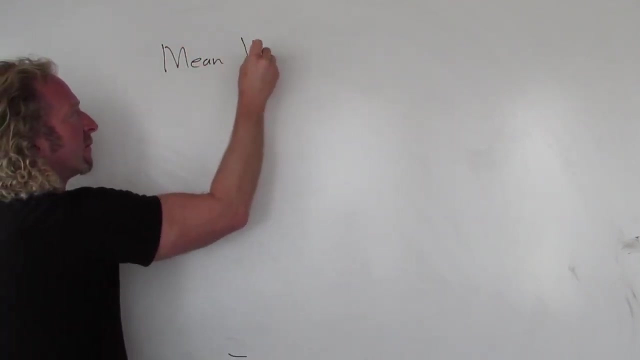 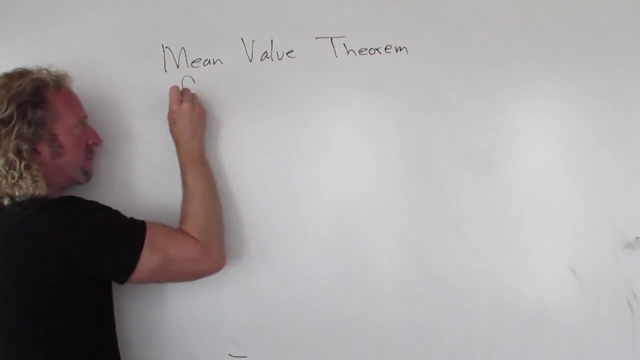 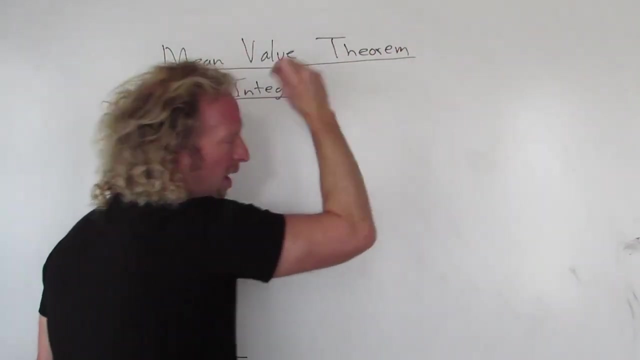 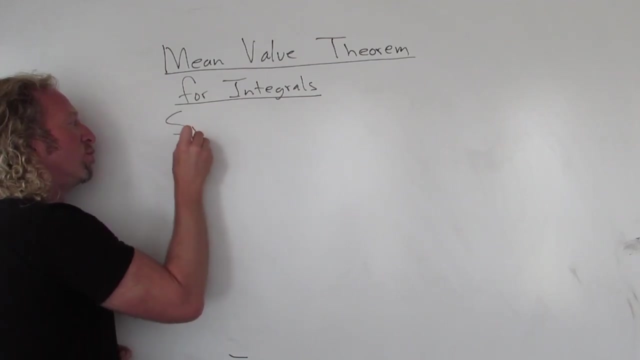 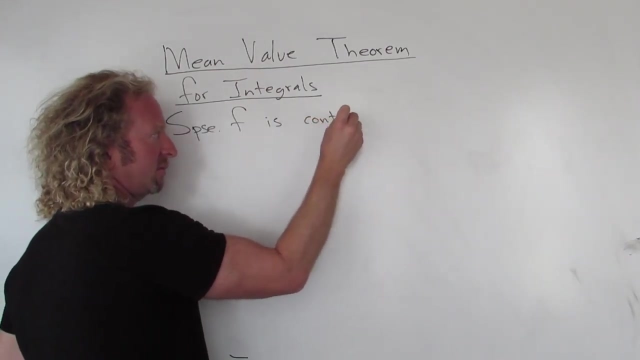 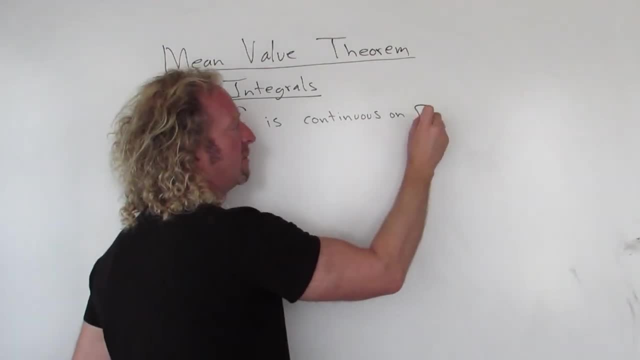 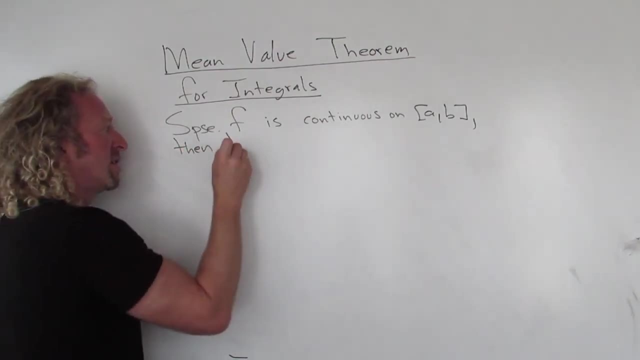 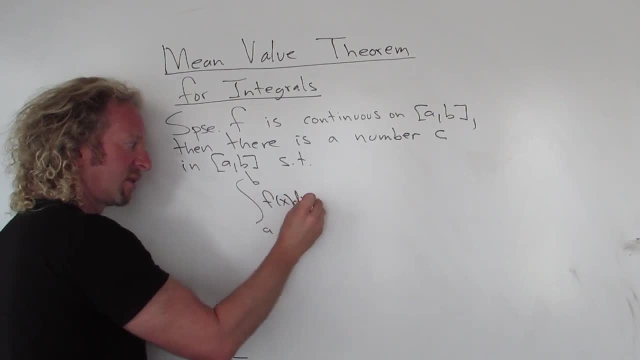 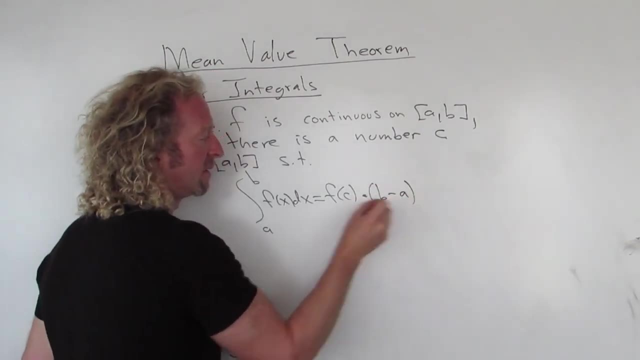 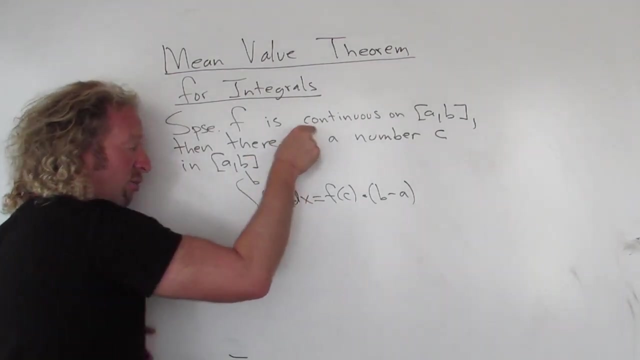 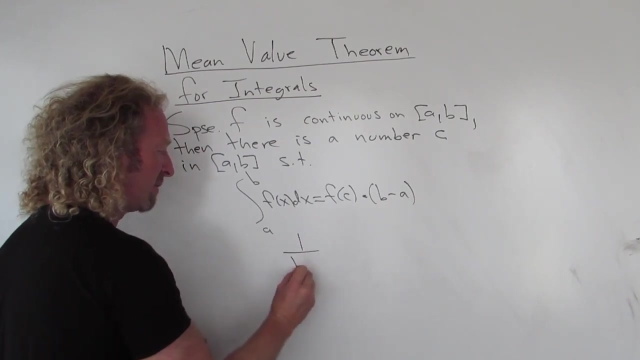 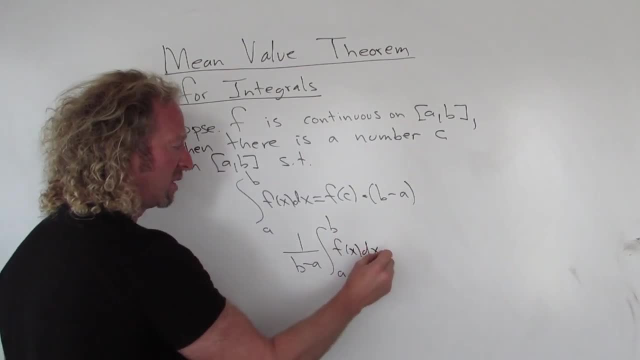 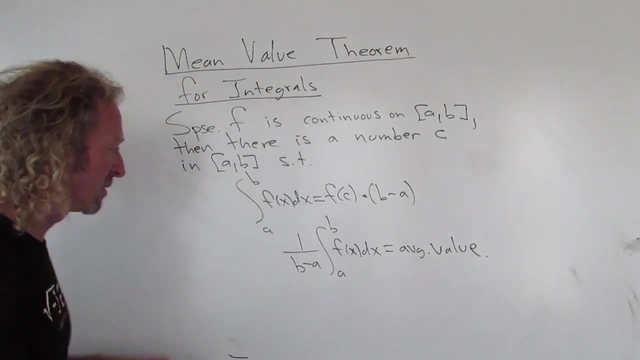 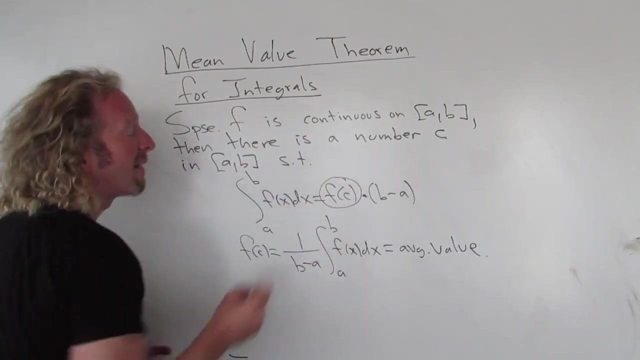 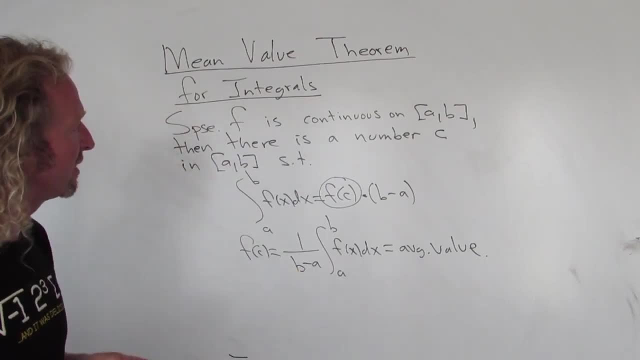 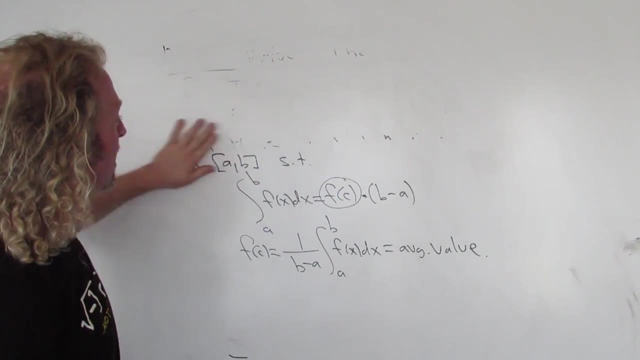 f of c is the average value of the function. Let's draw a picture so you see what all of this is. It's really, really interesting. So I'm going to erase this because we don't need it anymore, And I'll draw the picture up here. 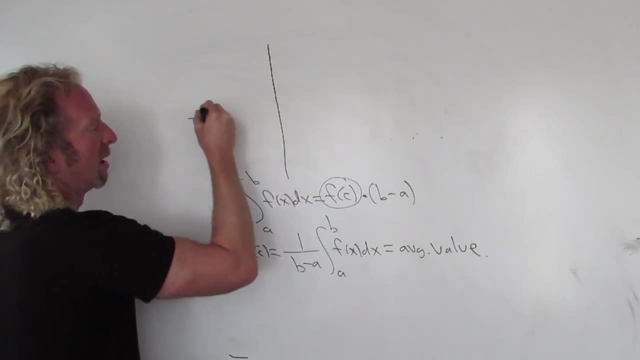 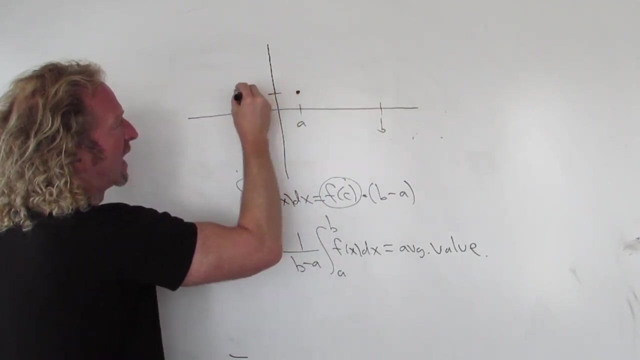 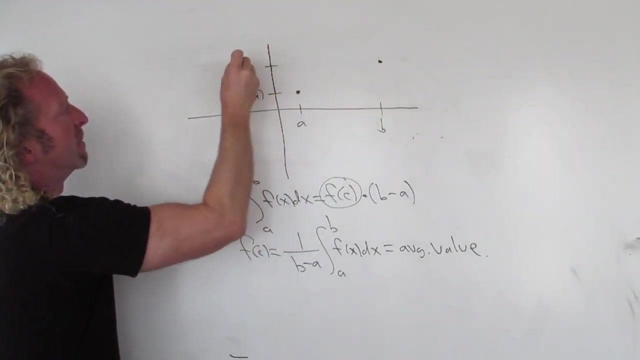 So this will be our y-axis, This will be our x-axis. So here's a and here's b. I'm going to be careful: here This is f of a, And then maybe here, this is f of b. So this is f of b. 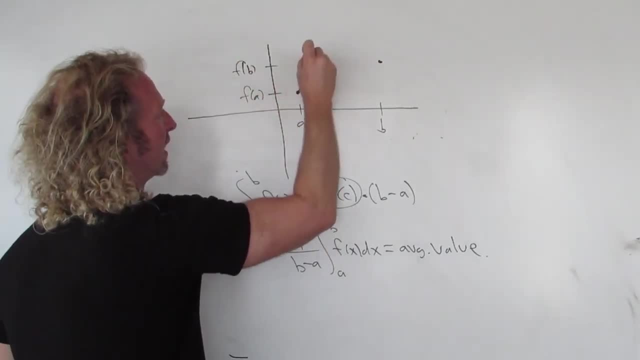 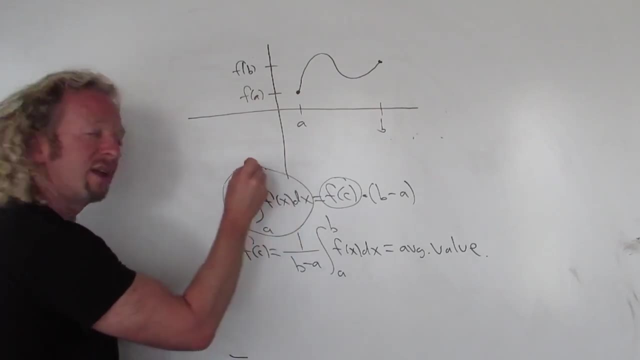 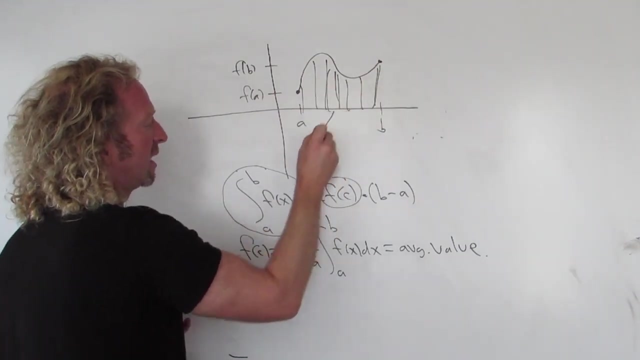 Good stuff And then maybe draw it like this: There we go, There's our function, And so first let's examine this. This is the area under the curve, So this area here, This is the area right, That's the area under the curve right. 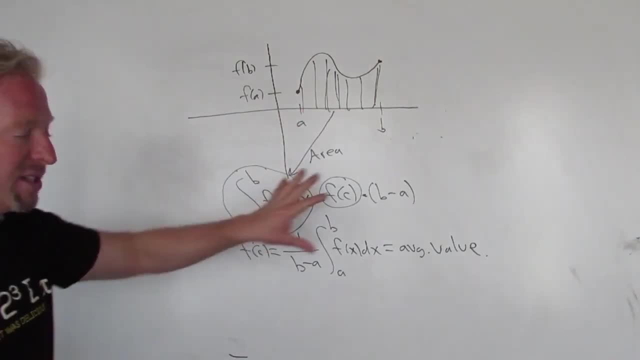 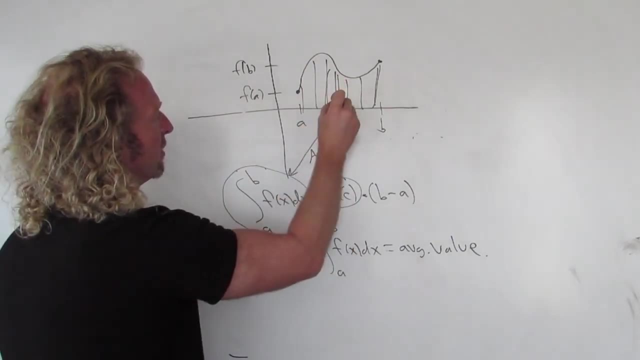 So the area under the curve? okay, the area under the curve is equal to this expression. So what is this expression? Well, the mean value theorem says there is a number c, So I'm going to pick the number to be here so that the picture makes more sense. 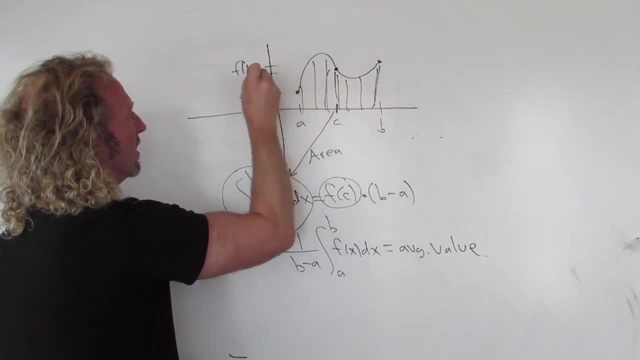 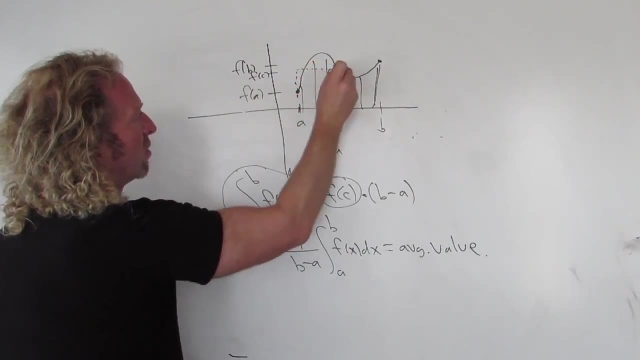 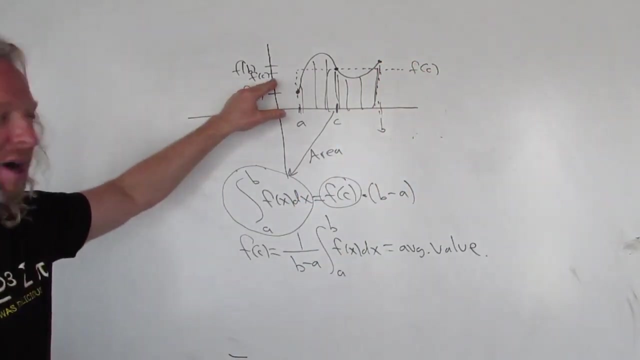 I'll do it here. So if this is c, this is f of c. okay, so I'm just picking the number And what you can do is you can draw a box whose height this f of c. so this is f of c. so f of c is the height of this box. 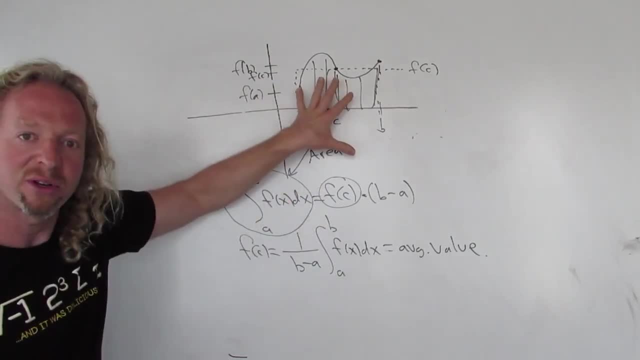 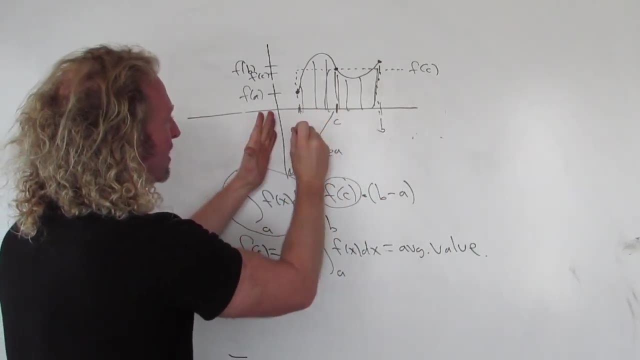 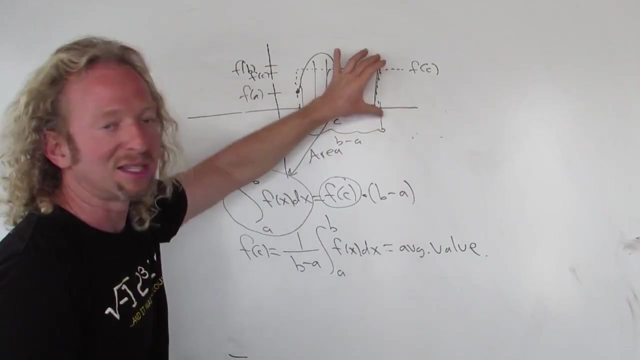 And so what the mean value theorem is saying is that the area under the curve is equal to the area of the box, right? Think about it: If this is a and this is b, then this distance here is b minus a. So, remember, the area of a box is the width times the height, right. 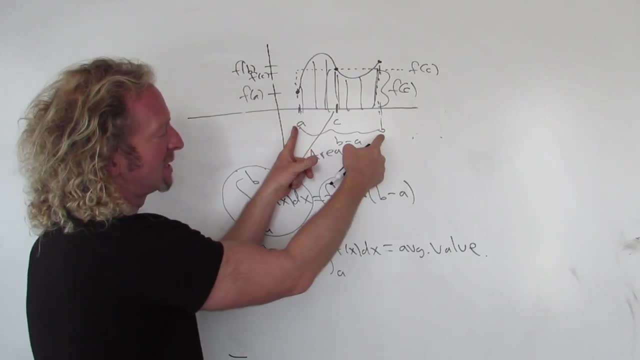 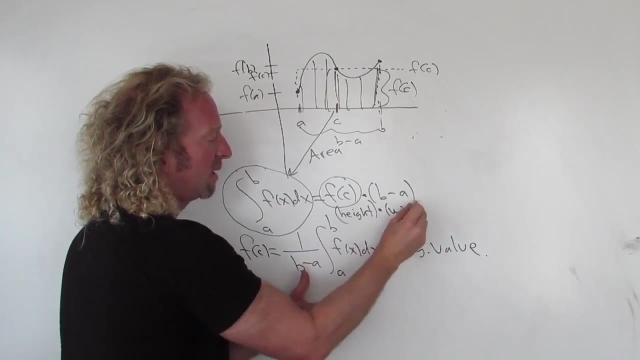 The height of the box is f of c, The width is b minus a, So this is the height. So this is the height, The height times the width. So the mean value theorem for integrals says: if you have a continuous function, 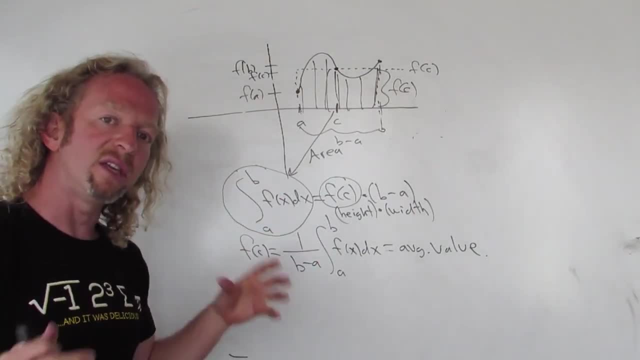 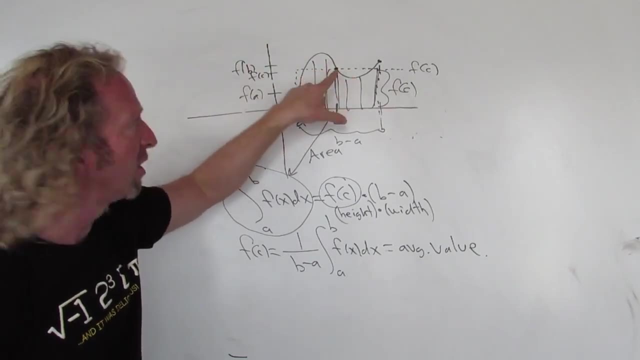 it's continuous right. There is a number c in the interval, such that the area under the curve is equal to the area of the box, whose height is f of c. And what is the height of the box? The height of the box is the average value of the function. 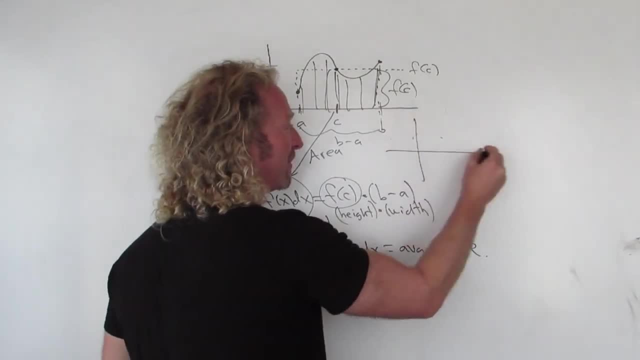 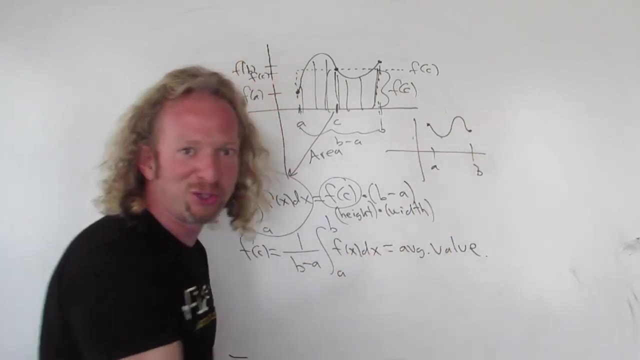 Deep stuff, Pretty wicked, So again. so if you have a and you have b and you draw a picture like this, you should be able to find a box that gives you the same area somewhere. So maybe this is that box, right. 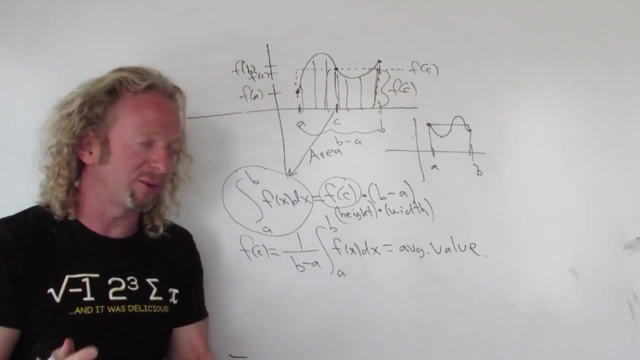 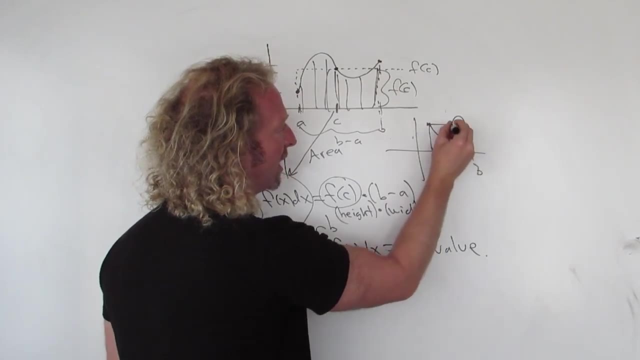 And the height of that box is called the average value of a function, right. So the height of that box is called the average value of the function. In this case, this here would be the value of c, right, And this would be your f of c. 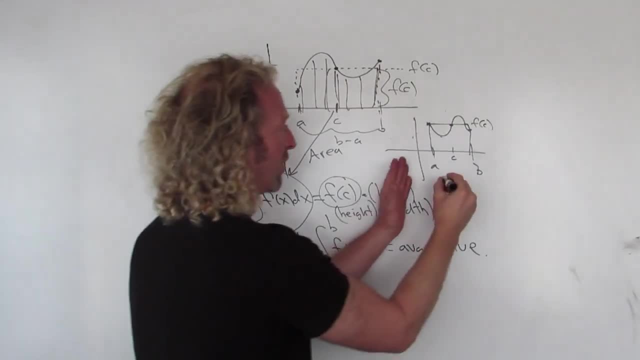 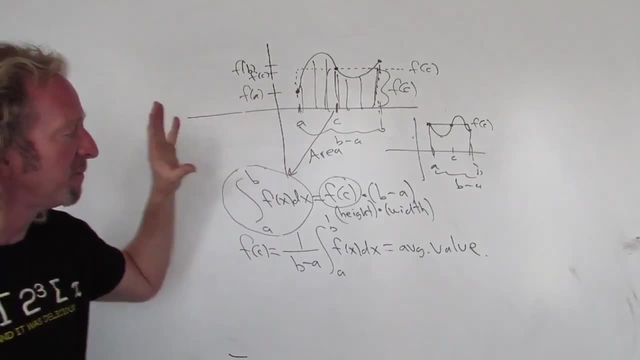 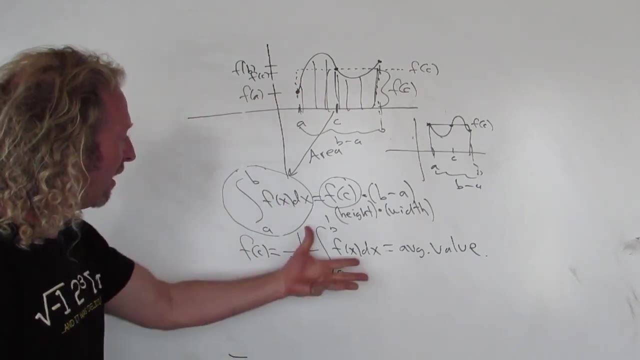 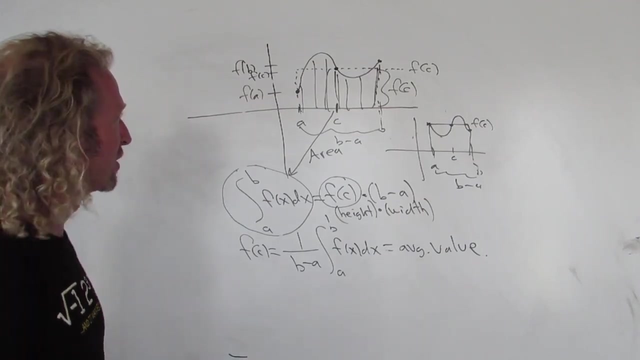 It's height times width, or width times height, So the area under the graph is equal to the area of the box. All right, Let's go ahead and do a simple example of finding c. maybe Let's try to find c and let's try to find the average value. 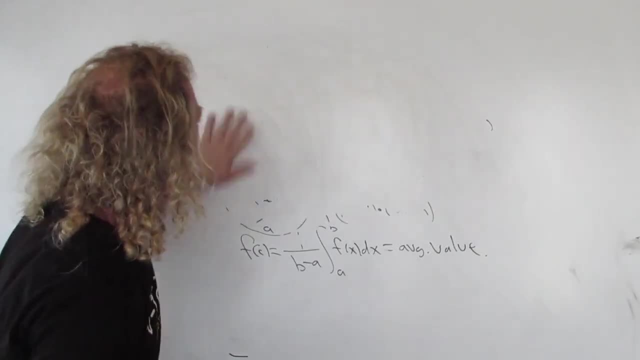 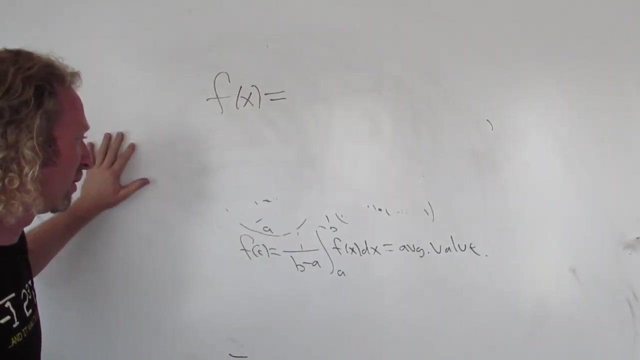 So I'll see if I can make one up. Let's see: f of x equals, f of x equals. Let's see, I guess we should be able to do this regardless, As long as we have a continuous function. right, this should work. 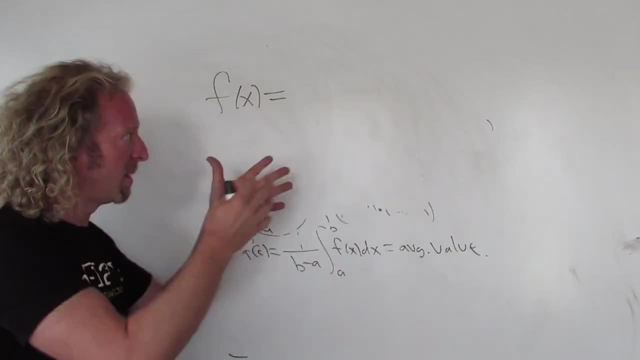 The criteria is: we have a continuous function on the closed interval, So if I make one up, we should be able to do it. Here we go. I'm going to try to make up the easiest possible one. f of x equals x squared. 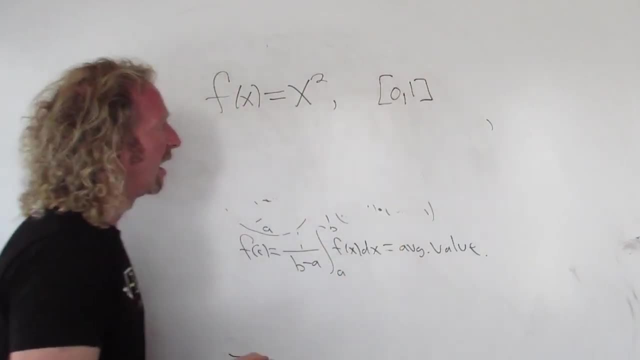 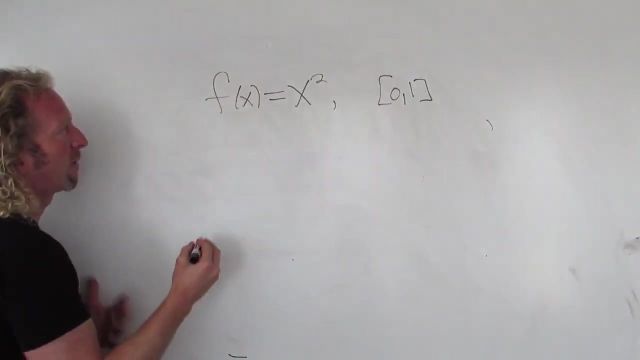 Let's just look at 0, 1.. OK, Let's find the average value, and then let's find the value of c. So the formula, the way I like to memorize the formula for these problems is as follows: 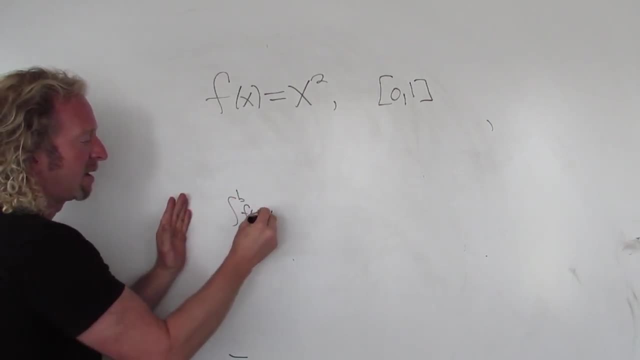 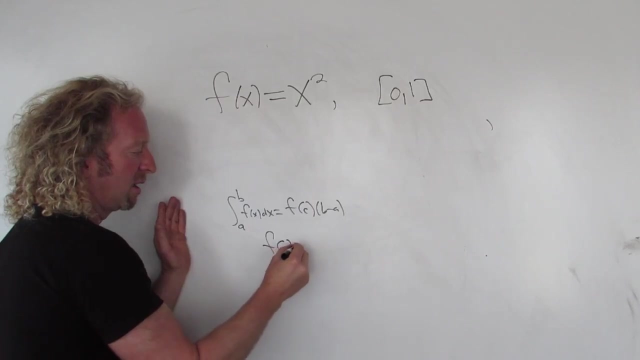 The theorem says you have the definite integral from a to b and that's equal to f of c, b minus a. So if you divide by b minus a, you get f of c equals 1 over b minus a times the definite integral. 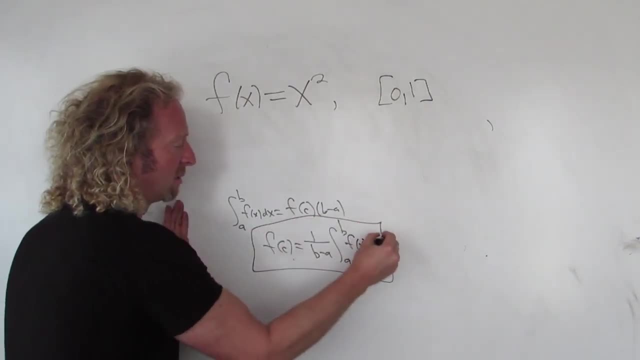 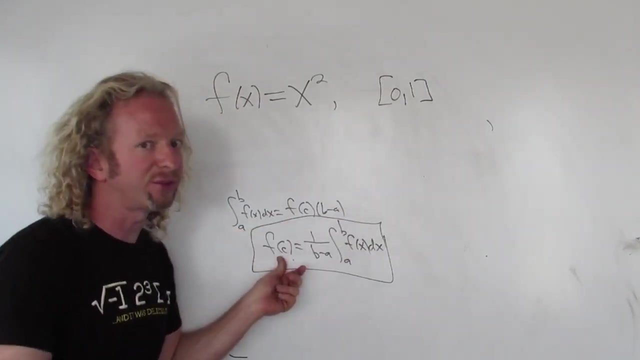 So this is the formula I always use for the problems. It's just easier, So I'm going to use this one. f of c is the average value. So if you had to find c, you just work this out and then you set it equal to f of c. 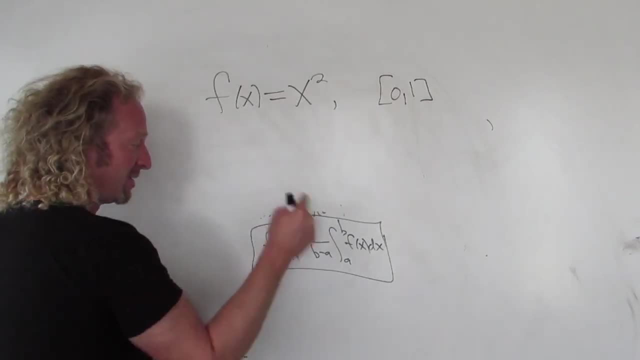 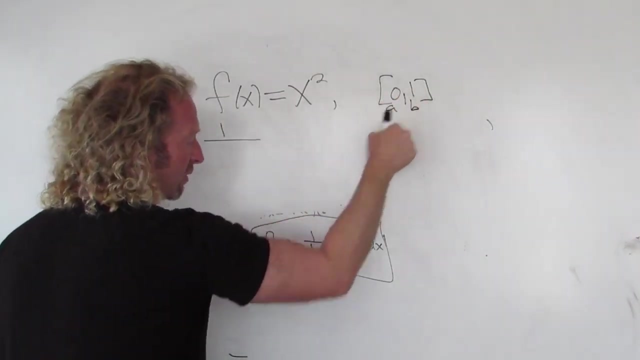 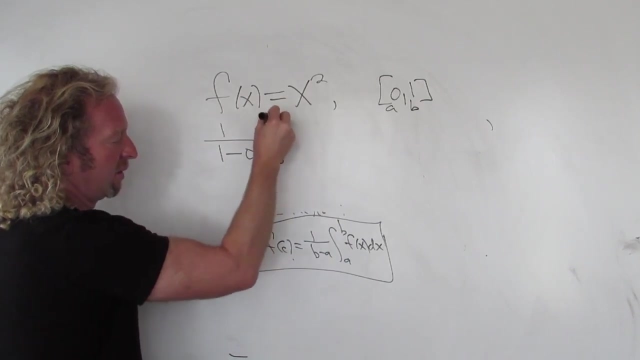 It's pretty simple. I hope Let's find out. So let's work out this piece first. That will be the average value, So it'll be 1 over. so this is a and this is b, So it'll be 1 minus 0, and then we're going from 0 to 1, right? 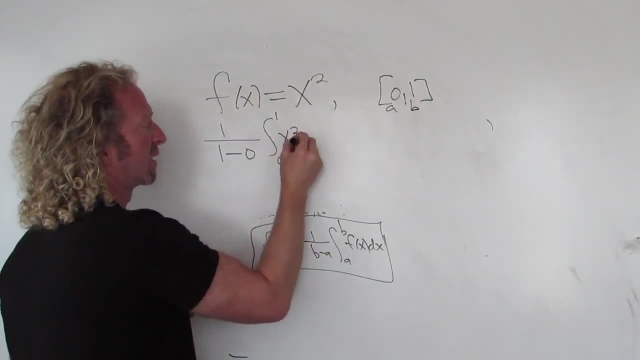 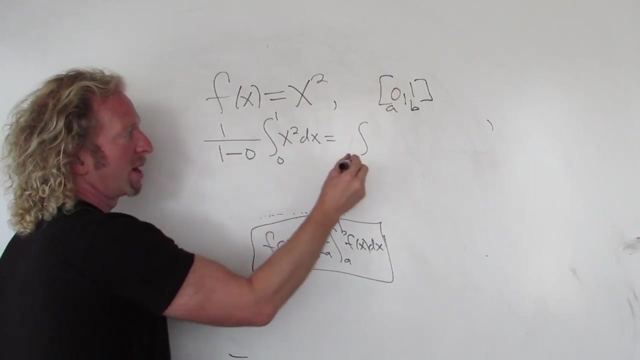 So far, so good. And then f of x is x squared, so x squared dx. That's just 1,. and then so it's just 1.. So it's just 1.. I won't write it. And then 0 to 1, x squared dx. 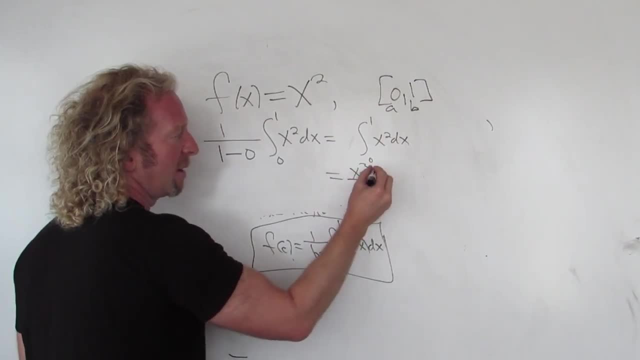 When you integrate x squared, you get x cubed over 3, and we're going from 0 to 1.. Then the final law of theorem of calculus says you plug in the 1, subtract and plug in the 0.. 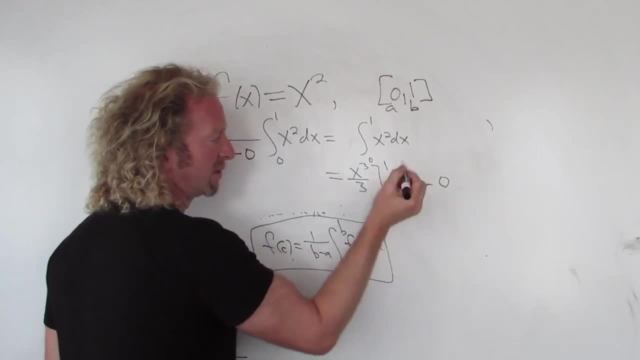 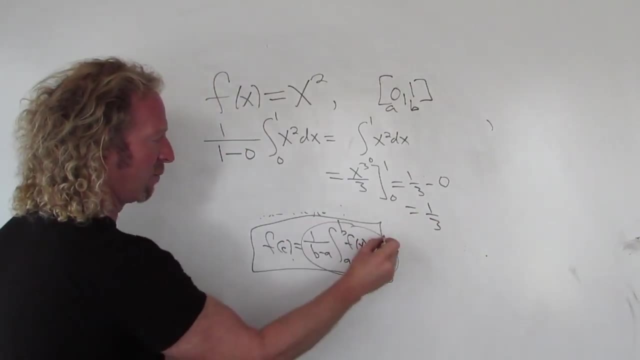 So you get 1 third minus 0, because 0 over 3 is 0. So you just get 1 third, So 1 third. So we work this out and we got 1 third right. So now we just take f of c. 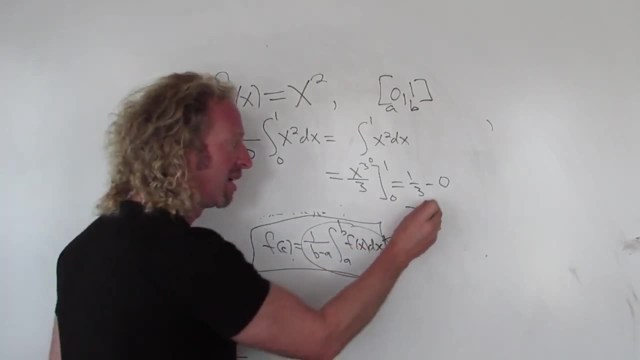 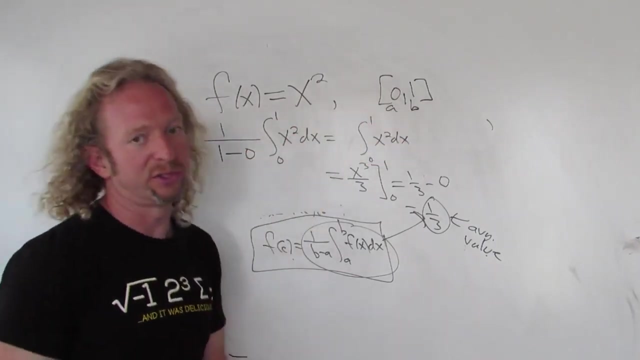 Oh, and what is this? This is the average value. This is the height of the box right. This is the average. This is the average value of the function over the interval 0 to 1, right, It's the height of the box right. 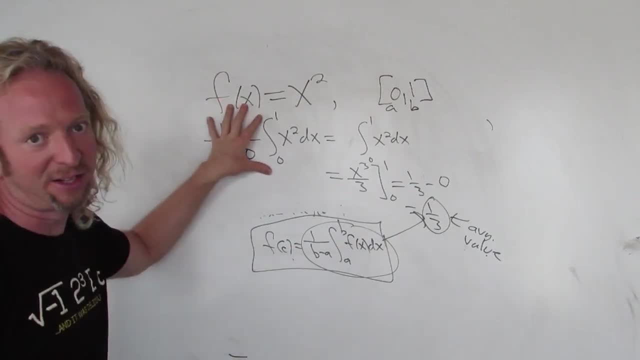 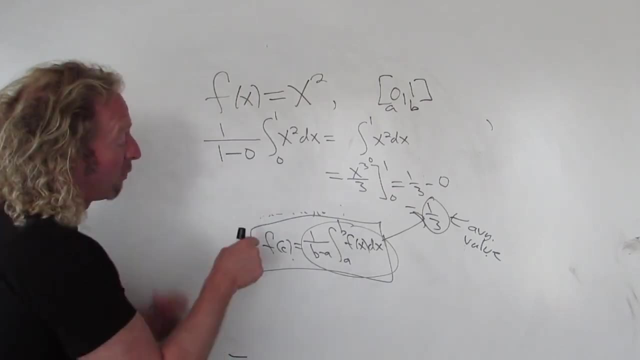 That gives you the same area as the definite interval from 0 to 1.. Okay, so now we're going to find f of c. So how do you do that? Well, we're going to find c. rather Sorry, we're going to find c. 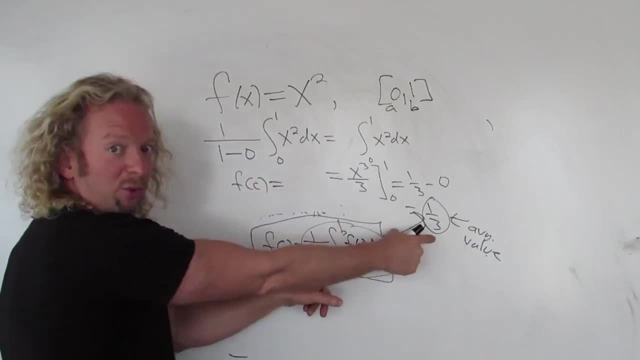 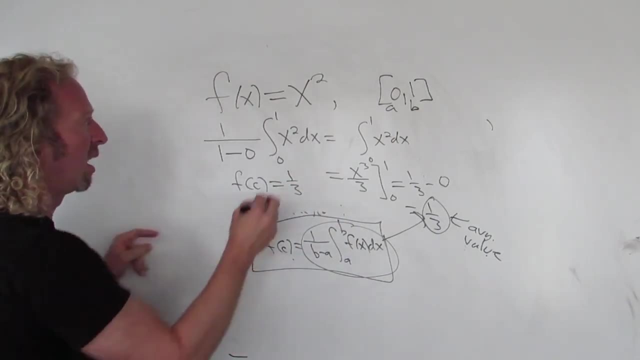 So we'll set f of c equal to the quantity which we worked out, equal to the average value, okay, And then we just replace c with what it is, So f of what it is. So f of c is the same as f of x, except x is c. 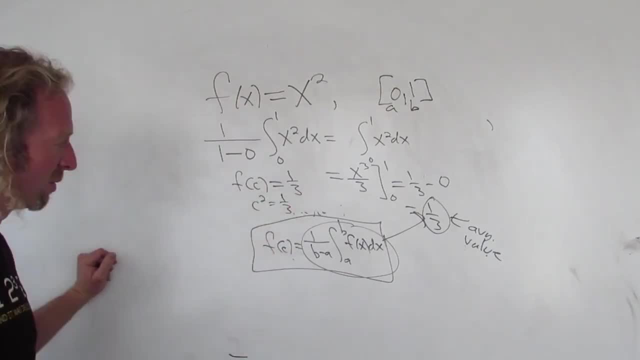 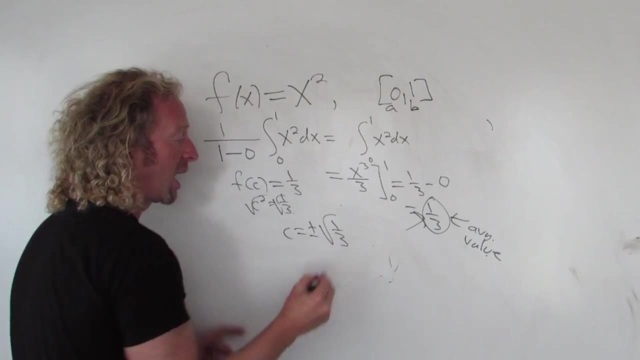 So this is: c squared equals 1 third. All right, c squared equals 1 third. And then, to finish, we just take the square root, So you get c equals plus or minus the square root of 1 third. We had to throw one of these away, right? 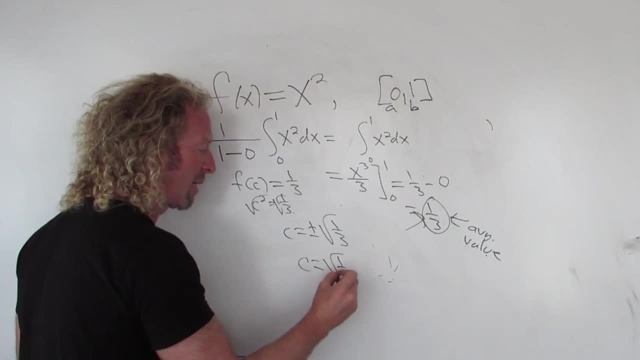 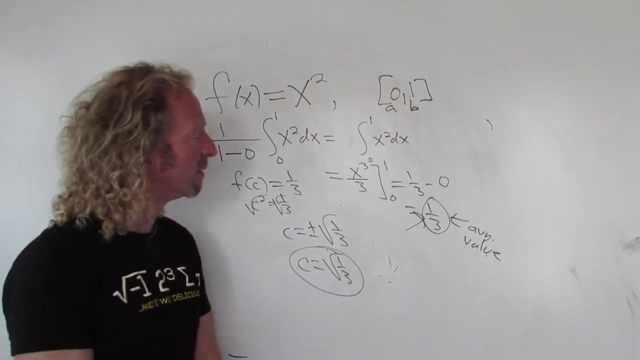 Because our c has to be in the interval, so we want the positive one. So that would be the value of c. I hope this video made sense and I hope it's helped you understand what the mean value theorem is. In the videos that follow I have lots of harder examples of finding c and so on. 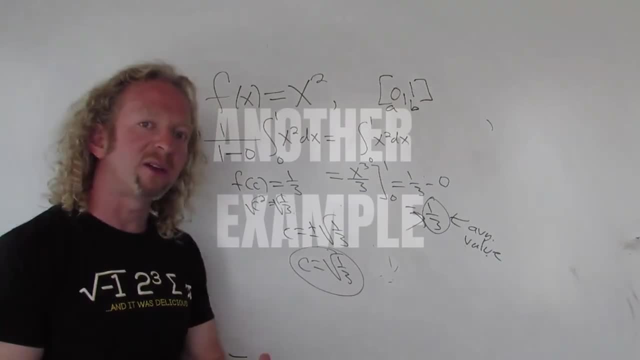 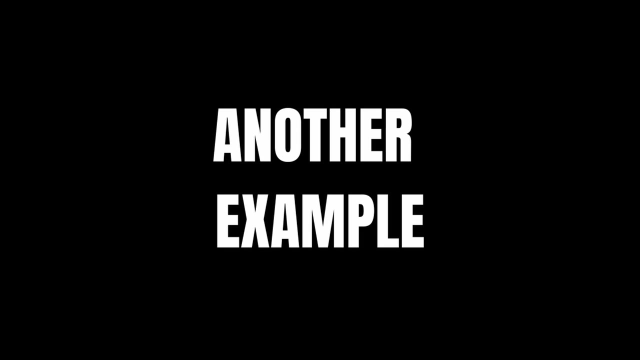 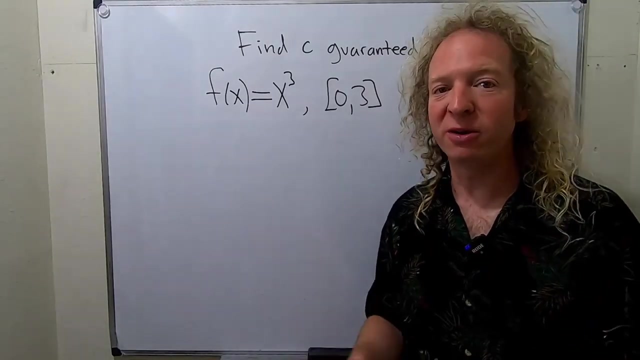 The purpose of this video was mainly to give you the idea of what the mean value theorem is. In this video we're going to find the value of c, guaranteed by the mean value theorem for integrals for this function on this interval. So that's a lot to say. 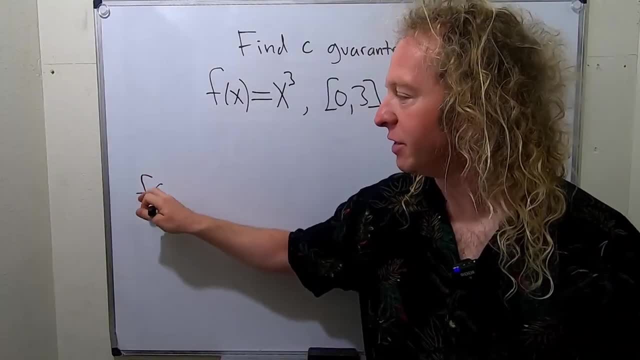 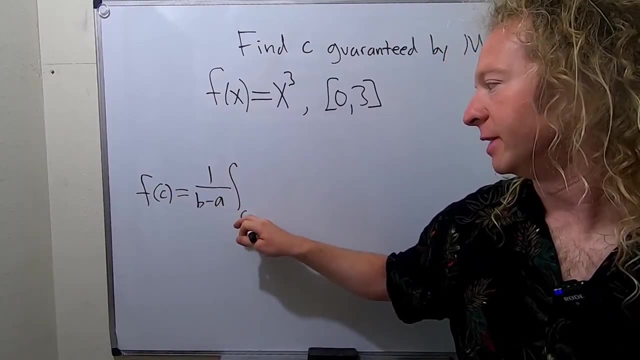 Let me just give you the formula and I'll explain it. So we have f of c. This is the formula, And this is equal to 1 over b minus a times the definite integral from a to b of f of x, dx. 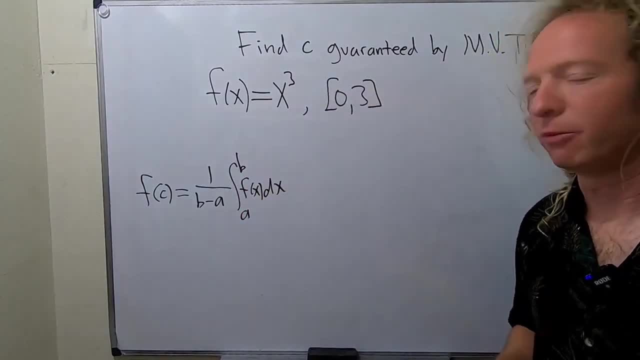 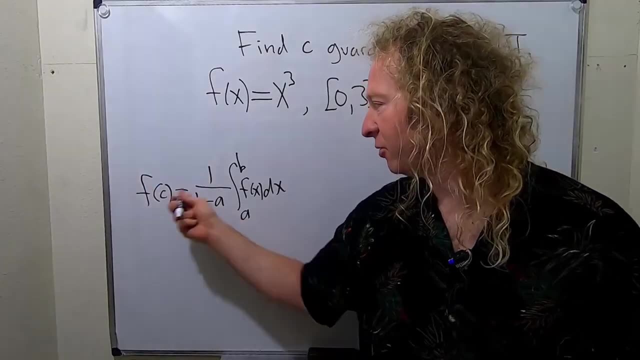 So this is the formula that we have to use in this problem. This is a mean value theorem for integrals type problem. So this is called the average value of the function, this whole thing here. This is the average value of this function over ab. 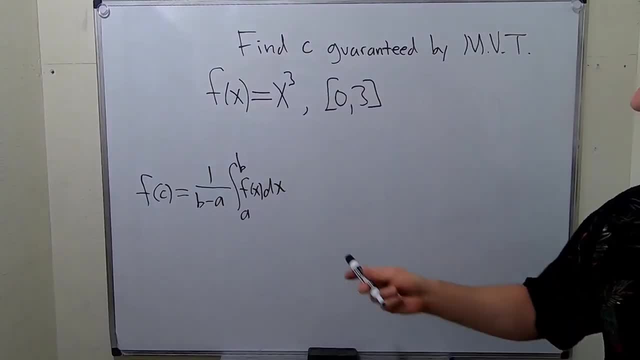 We have to find c, So we basically have to work this out. So let's go ahead and work this out. So let's go ahead and work this out. So let's go ahead and work this out. So this is your a and this is your b. 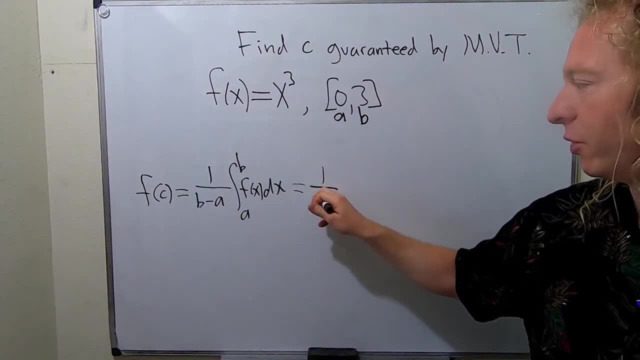 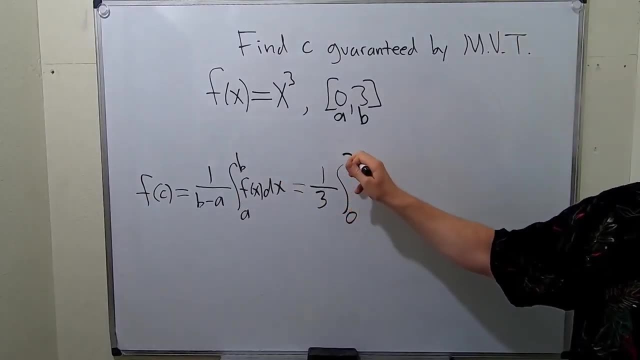 So this will be 1 over 3 minus 0. So 1 over 3, because it's really 3 minus 0. And then we're going from 0 to 3.. So 0 to 3.. And then f of x is simply x cubed. 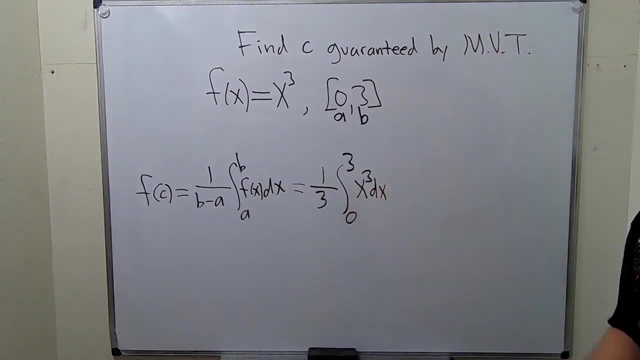 So this is x cubed. OK, this is a little bit easier than I thought. OK, so 3 minus 0,, 3 minus 0.. I haven't done these in a while, So now you just integrate, right. 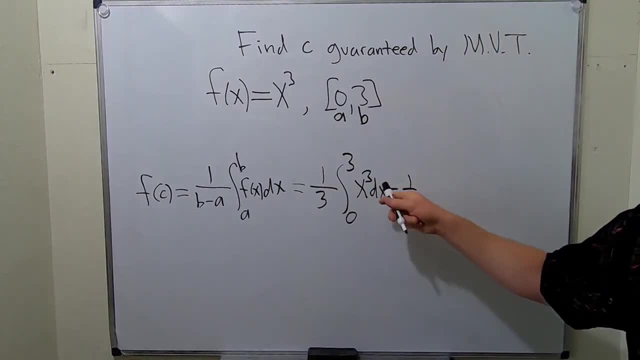 You just use the power rule, So this is 1. third, So you add 1, so you get x to the 4 over 4.. That's the power rule for integration And we're going from 0 to 3.. 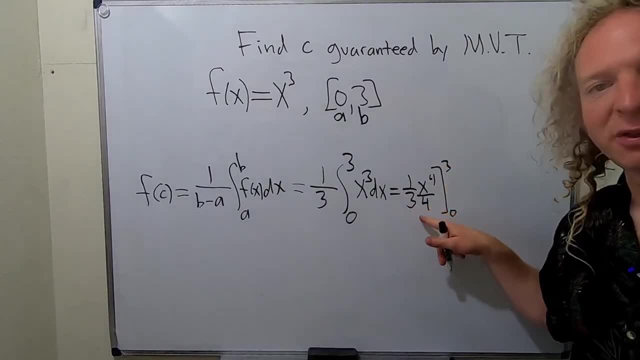 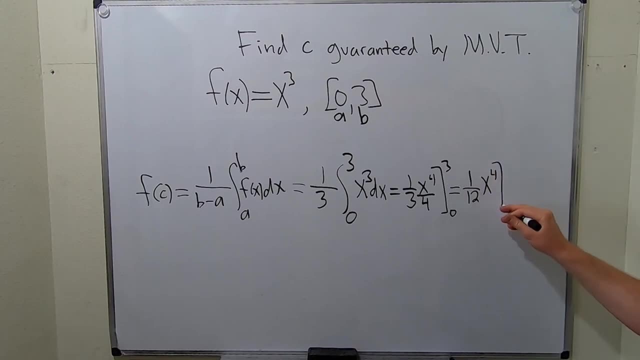 So 0 to 3.. Let's clean this up a little bit: 3 times 4 is 12.. So this is 1 over 12. x to the 4. And then we're going from 0 to 3.. 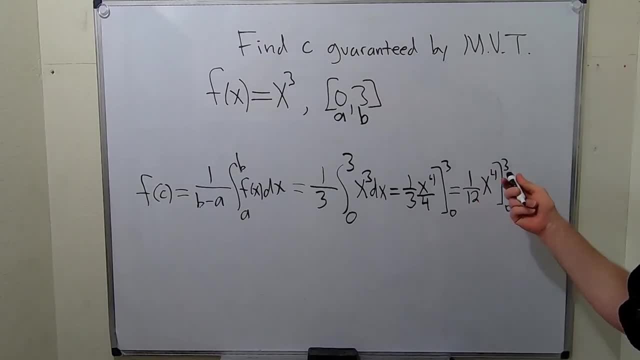 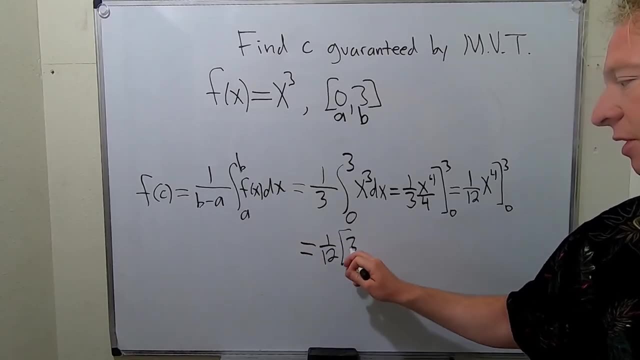 Good stuff, Really, really nice math. Oh, big numbers here. So you got to plug in the 3, subtract, plug in the 0. So this is equal to Come here. That's 1- 12th. This is 3 to the 4th minus 0 to the 4th. 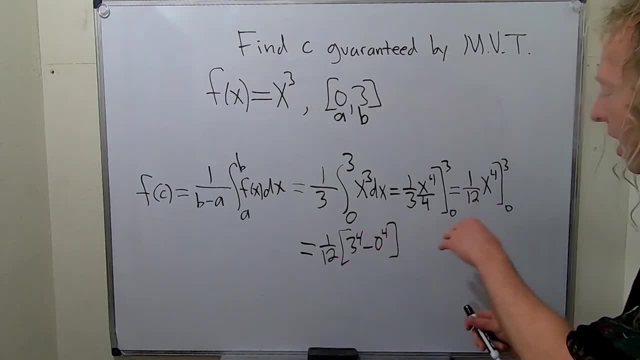 Notice how I left the constant out. You can do that, right. You can let this hang out and then plug in the numbers. So 3 to the 4th. I got to think about this. This is 1, 12th. 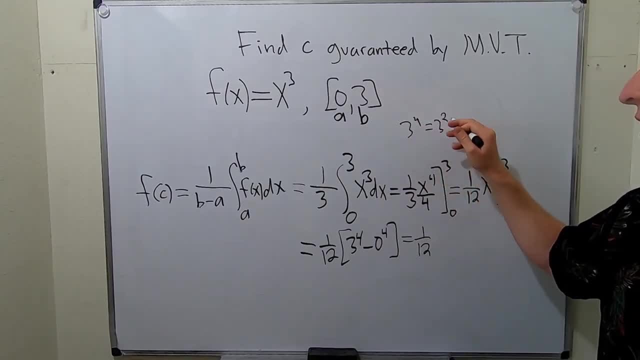 So, baby, math 3 to the 4th is 3 squared, 3 squared. Ah, I see, said the blind man. It's 9 times 9, which is 81. So this is 81. So 81 over 12.. 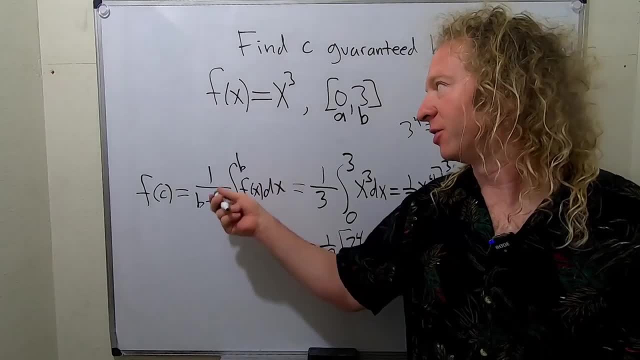 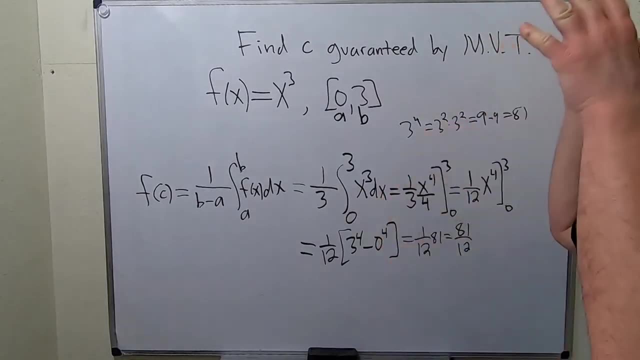 So this is called the average value of the function over this interval, because this is f of c. So that's not what the question wanted. The question wanted the value of c given by the mean value theorem for intervals, But this is called the average value. 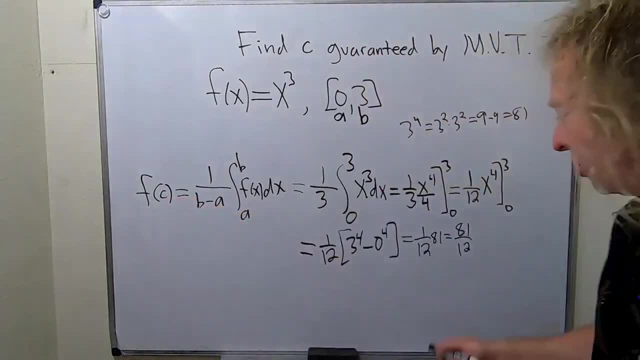 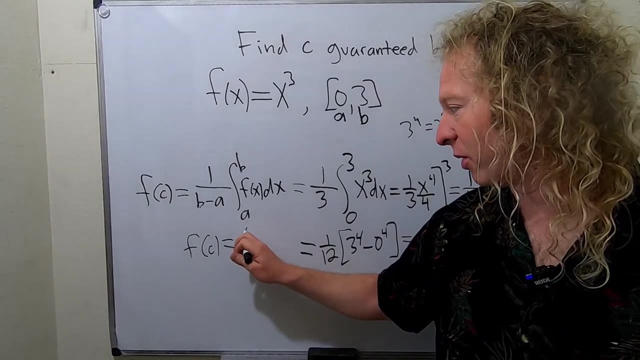 So now we have to find c. So f of c is equal to this. So, basically, you just take f of c and set it equal to this. You can use x. by the way, Most of the time when I do this, I just put f of x here.